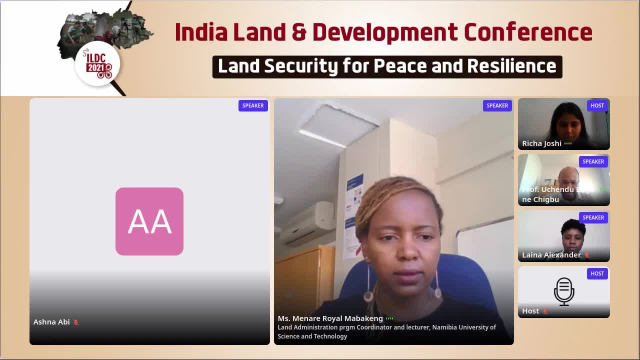 Hello everyone. Hello everybody, This session is the land use planning and land tenure session, And in this session I will be your moderator. My name is Uchendu Eugene Chiwu. I'm from the Namibia University of Science and Technology. As a matter of fact, this session itself is: 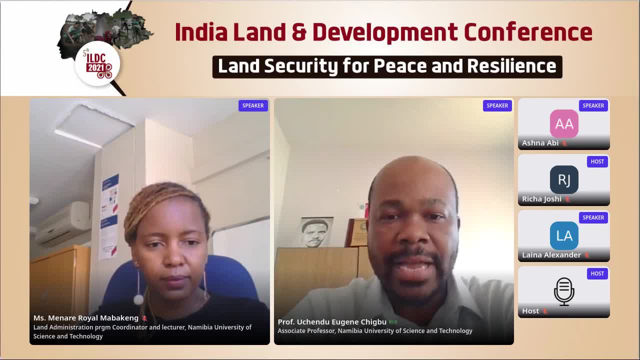 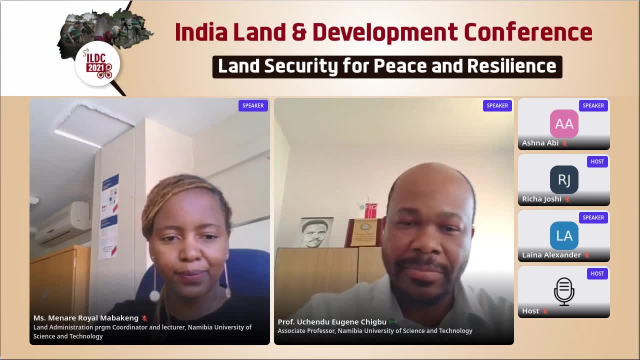 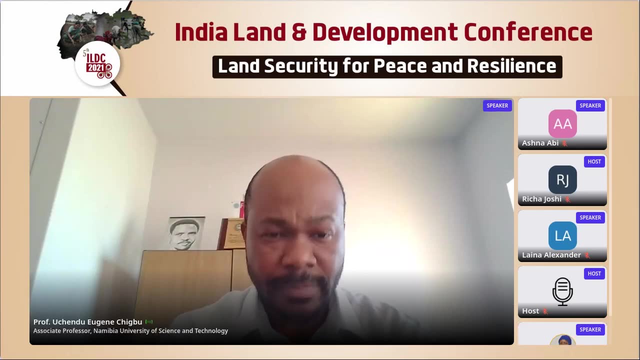 being hosted on the Africa Day. So the Namibia University of Science and Technology is one of the premier universities in the southern part of Africa, And today our session will focus on not just introducing our own university, but introducing the work that we do. But the 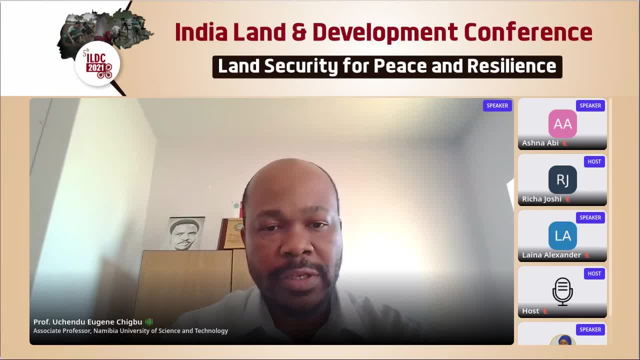 Tenant Responsive Land Use Planning itself is just most is much more than a concept and a practice, But it's. it's been a project since 2014.. And we'll seize every opportunity to discuss all issues relating to tenure. The rules: it's simple. As your moderator. 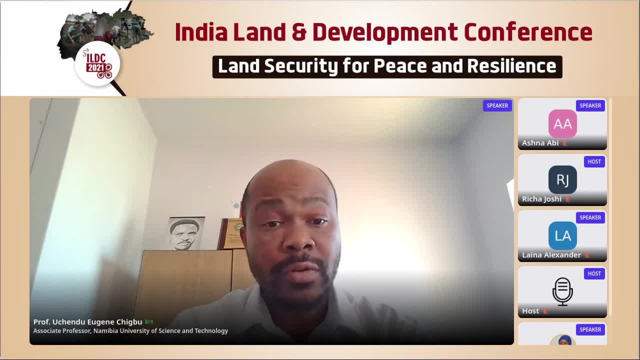 I would introduce the first speaker, who would speak about NOST and the work we do- And of course she will introduce herself as well- And then afterwards I would present the Tenant Responsive Land Use Planning And later on, the third speaker, who would be the last speaker. 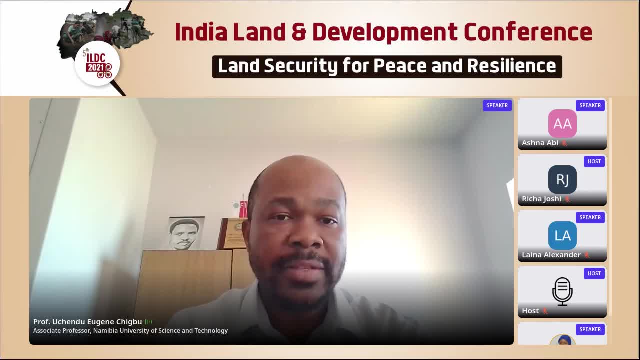 would present, at the local level, how this Tenant Responsive Land Use Planning has been implemented in various versions. Just to start, I would like to introduce Laina Alexander, who will be the first speaker, And before that I would like to simply mention that. 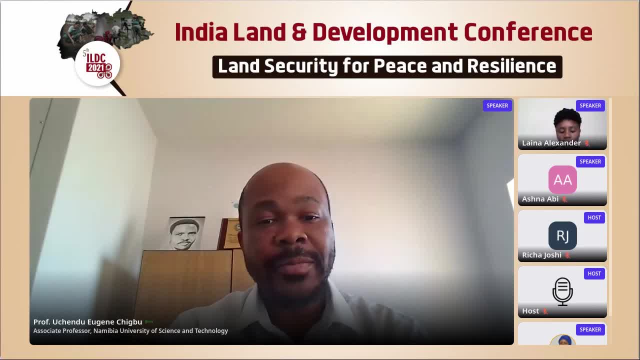 the Namibia University of Science and Technology is coming from the southern part of Africa. It's a university where we have the vision to commit 100% to Africanness, but as well as 100% to global structures. So you would find out from this work, as Ms Laina Alexander will present soon, that we have our tentacles. 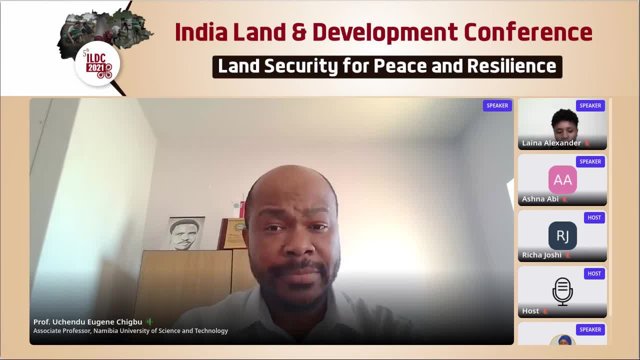 all over the place And our interest in this particular conference and special thanks to the organizers of the conference. Our interest in this conference is to connect, to raise the discourse, as to contribute as well to the global agenda, And with that I will invite. 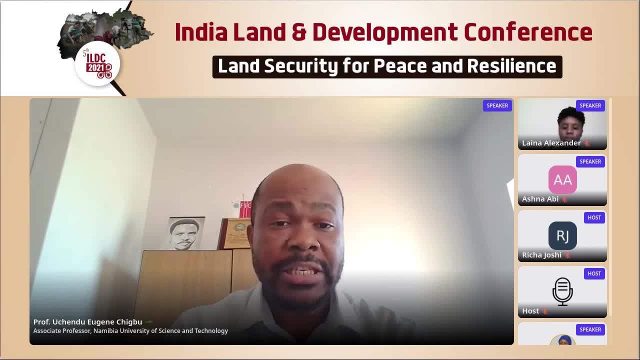 Laina Alexander, who will do the first presentation, And I will expect that the three presentations will be completed before we begin to take questions, And so, Ms Laina Alexander, you can introduce yourself and go on with your presentation. Thank you. 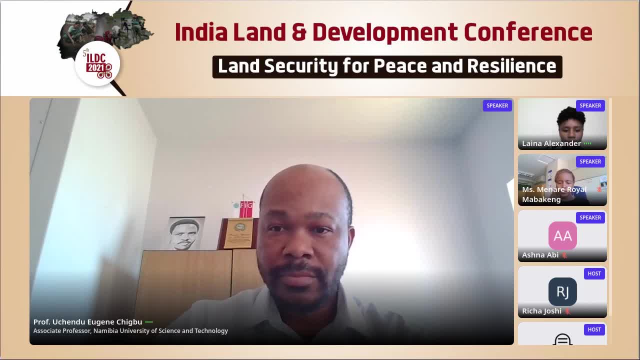 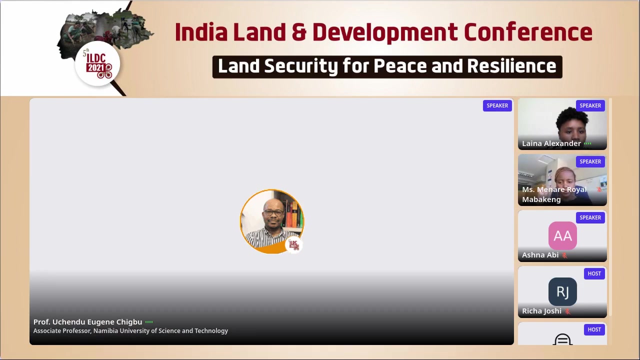 Thank you so much. Let me just share my presentation. Please, if you have any questions, put it on the chat. I'll be taking record of the questions and at last we'll have a discussion. Go on, Laina. Okay, the presentation is loading up, But in the meantime let me just introduce myself. 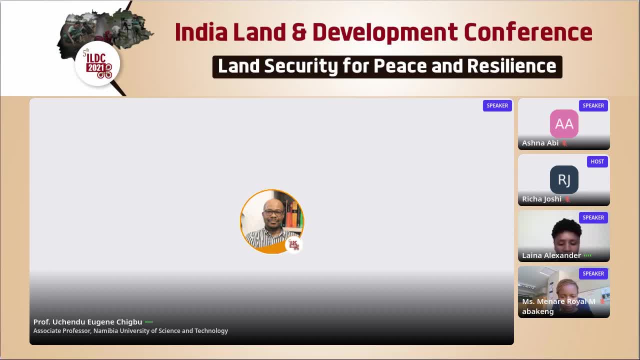 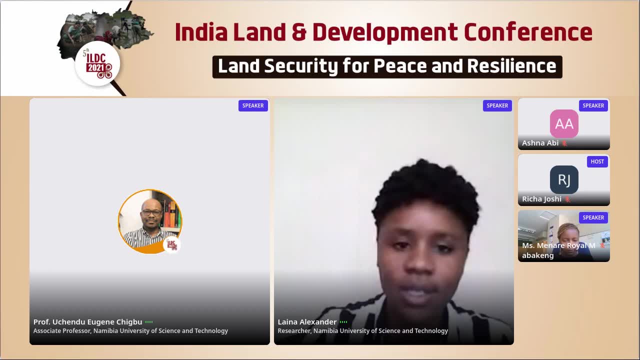 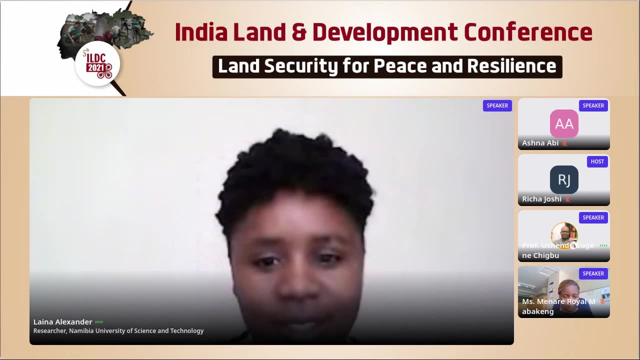 My name is Laina Alexander and I'm a research assistant here at the Namibia University of Science and Technology in the Department of Land and Property Sciences, Nice to be in my home for almost, I think, five years now. I did my bachelor's degree here and I've got 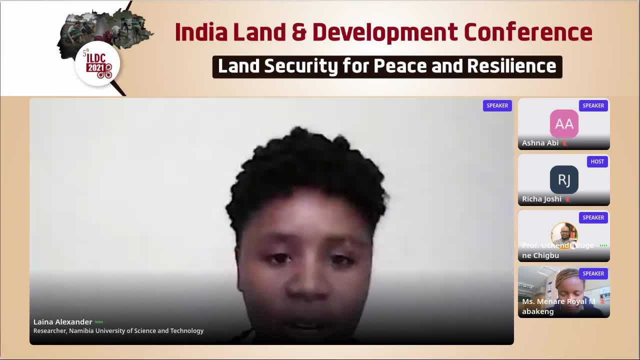 later continued with my honours in land administration And I'll also be continuing my master's here at the university. So is my presentation up? Are you seeing it? Not yet, Not yet. Okay, Prof, maybe if you could share it on your end. I sent it via email. 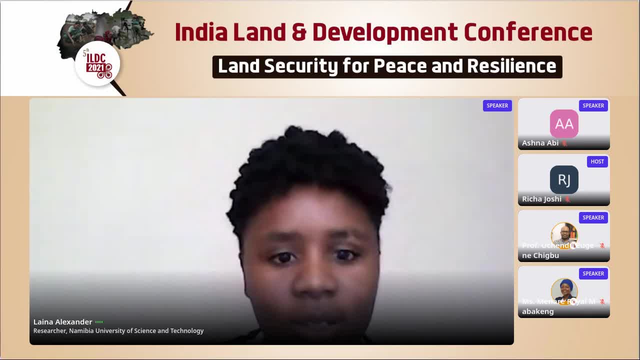 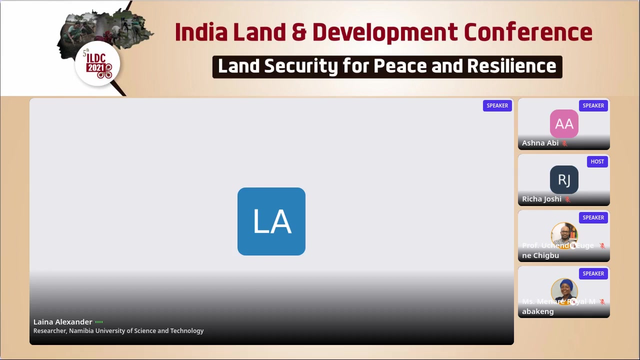 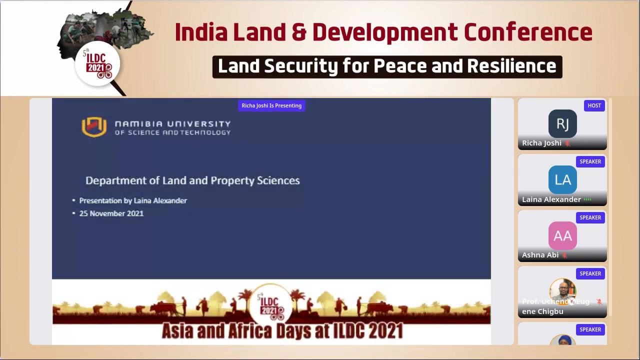 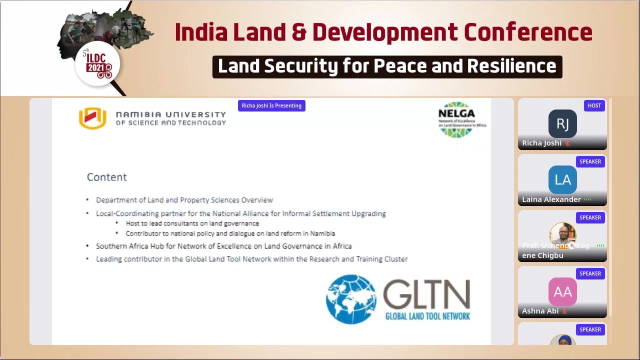 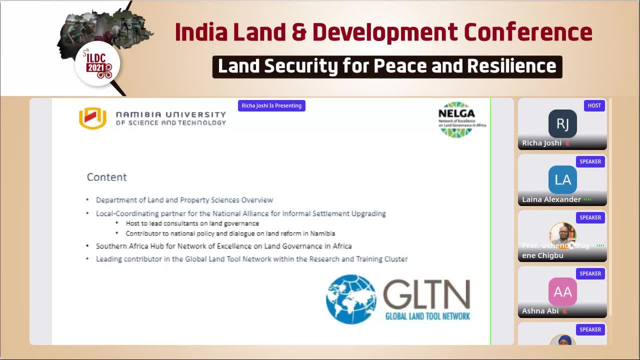 So this is the content that will be covered in the presentation, where I'll give an overview of our department and also cover the local coordinating partners for the National Alliance for Informal Astronomy and Upgrading. We'll also discuss the Southern Hub for Network of Excellence. 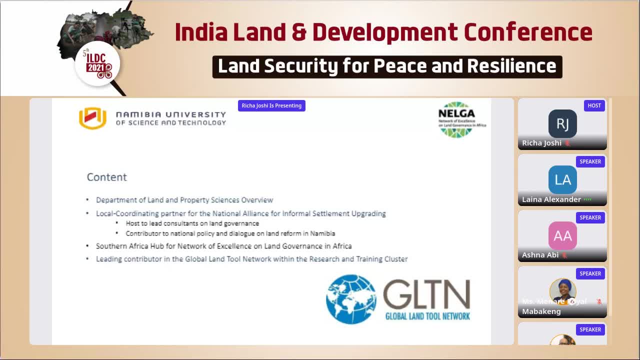 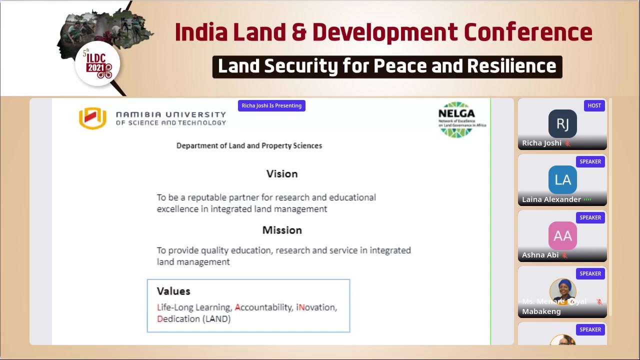 on Land Governance in Africa, that is, NELGA. And then, lastly, we'll look at the leading contributor in the NGLTN within the research and training cluster. Next slide, Sorry. So the vision for the department of Land and Property Sciences is to be a reputable partner. 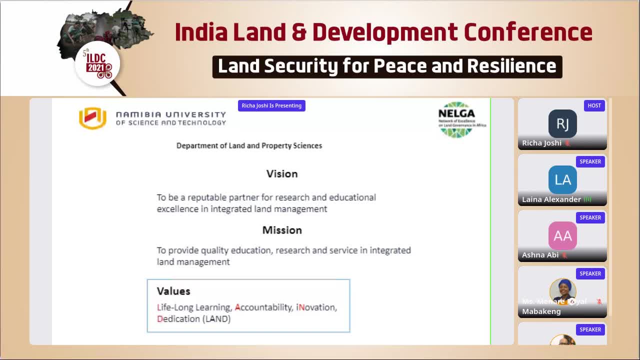 for research and educational excellence in integrated land management. Our mission is to provide quality education, research and service in integrated land management. The values are lifelong learning, accountability, innovation and dedication. Next slide: So what you see here is the structure. 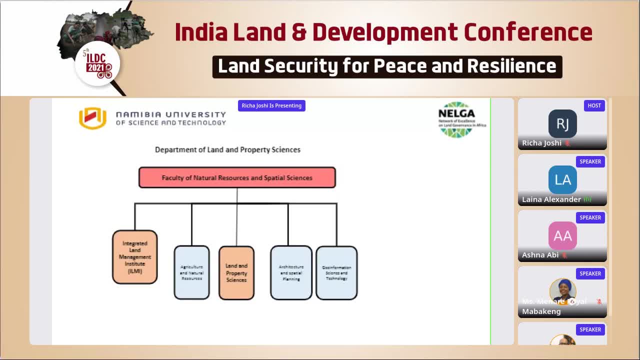 So the Department of Land and Property Sciences is under the Faculty of Natural Resources and Special Sciences. Under this faculty now we have integrated land management institute, We have agriculture and natural resources, We have land and property sciences, We have architecture and special planning. 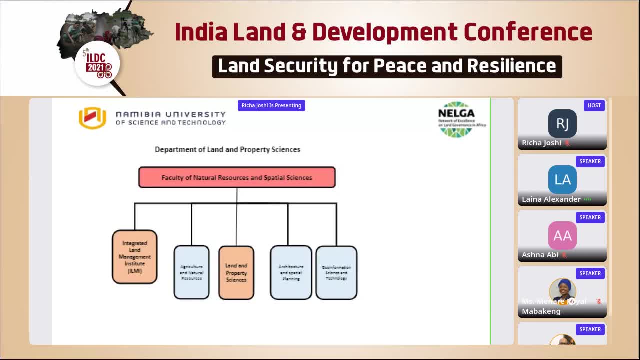 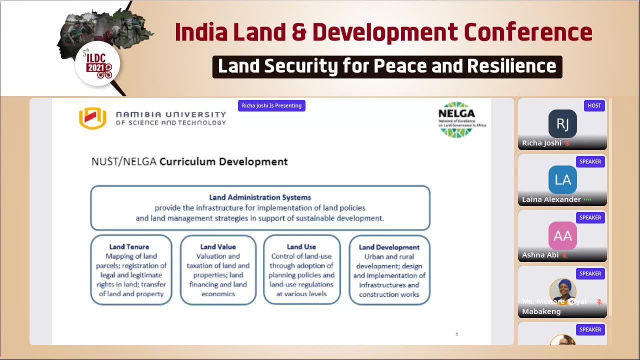 and geoinformation science and technology. Next slide: OK, Okay, OK. So last on NELGA's curriculum development. So some of the of the stuff from our NIST have also been involved in curriculum development at the University of Zambia. 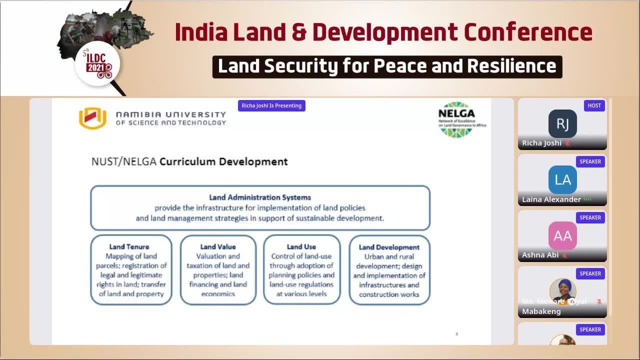 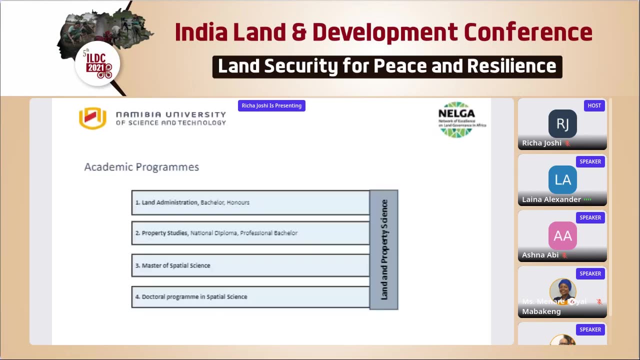 And yeah, Right, next, slide, Right, Next, OK, OK, Next slide, Next slide. These are the academic programs that are offered by the Department of Land and Property Sciences. We have the bachelor's degree and the honors degree in land administration. 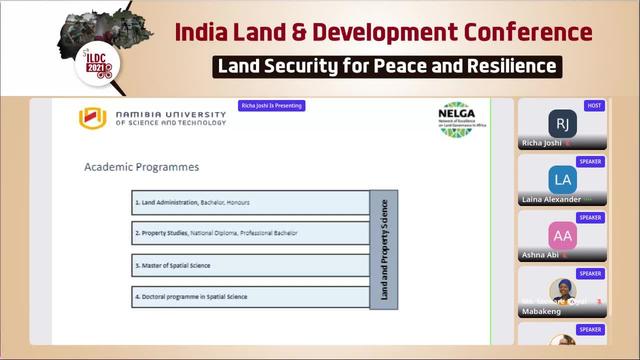 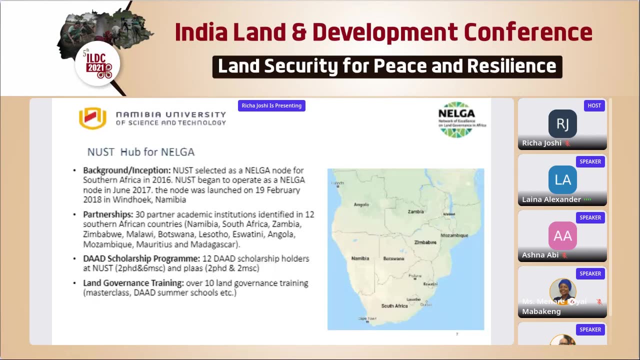 Then we have our national diploma in property studies and a professional bachelor's degree. Then we have the master of special science. Lastly, the doctoral program in special sciences. Okay, so is my voice. okay, Sorry, Okay, Yes, we can hear you. 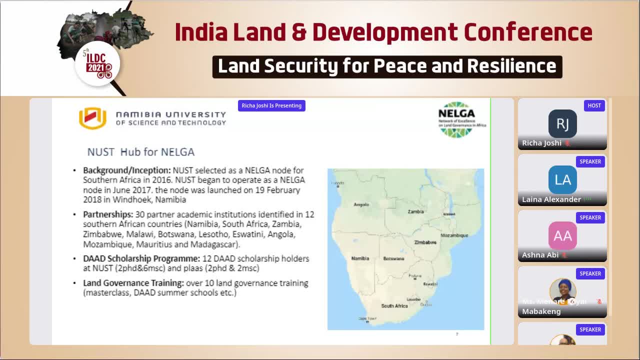 Okay, So NAST has been selected as a node by NELGA for South Africa in 2016.. NAST then began to operate as a NELGA node officially in 2017.. However, the NELGA node is not yet available. 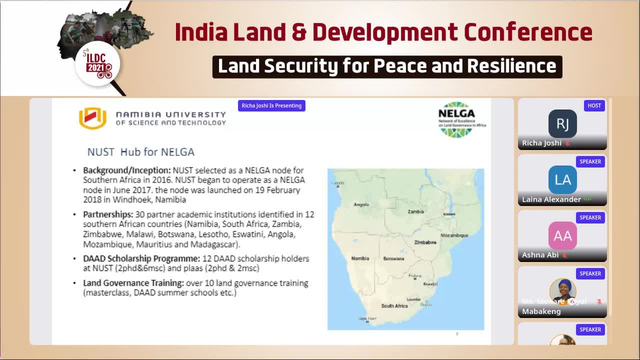 The NELGA node was launched on the 19th of February in 2018 here in Windhoek in Namibia. So the partnerships: There are 30 partner academic institutions that have been identified in 12,000 African countries. 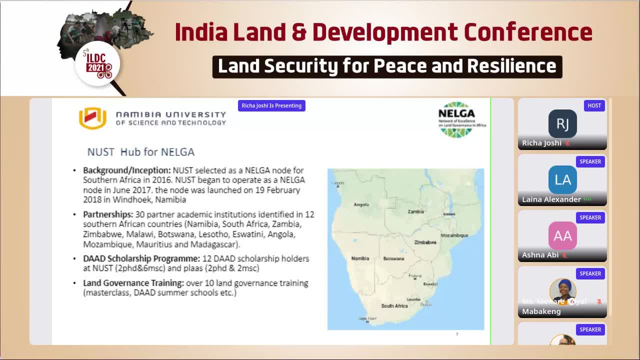 We have Namibia, South Africa, Zambia, Zimbabwe, Malawi, Botswana, Lesotho and Eswatini, Angola, Mozambique, Mauritius and Madagascar. So the DAAD scholarship program, The 12 DAAD scholarship holders, are currently at NAST. 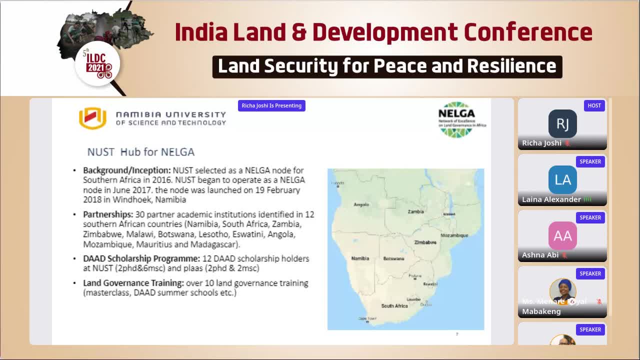 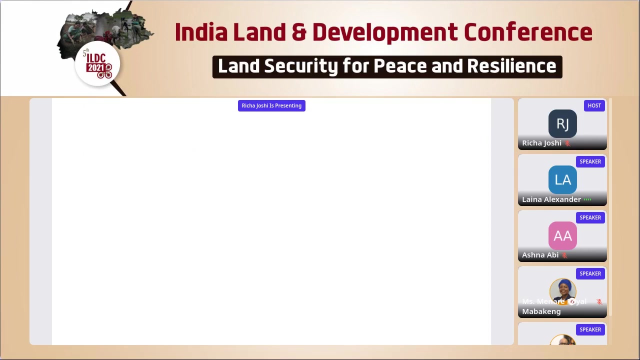 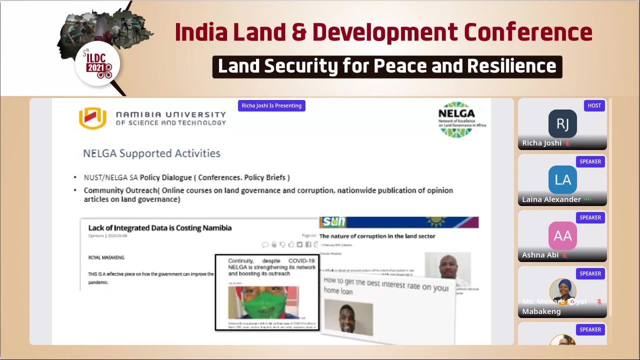 We have two PhD students and six masters Land governance training. There's been over 10 land governance training. We're in the. This was done via master classes in DAAD summer schools. Now below are the supported activities by NELGA: 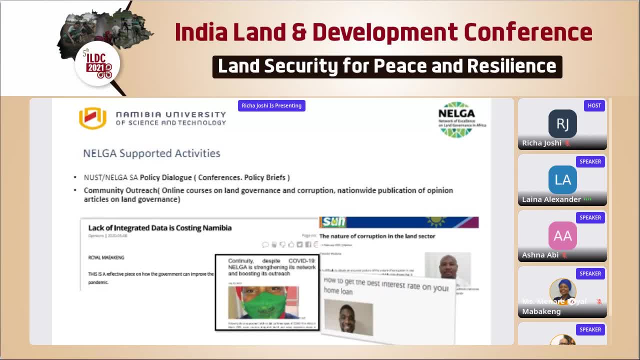 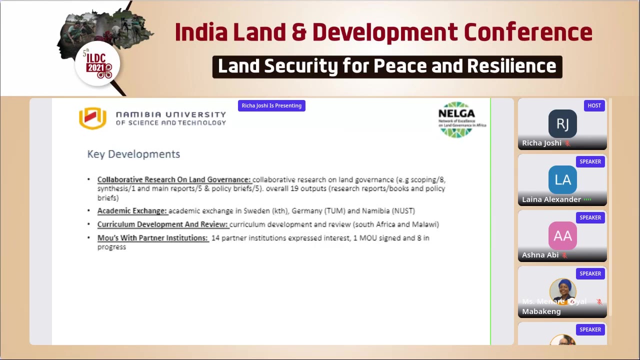 There's been community outreach programs that were done through online class and online classes on land governance, corruption, nation work. There have also been publications and articles that were published on land governance in local newspapers. Next slide: Key development between NAST and NELGA. 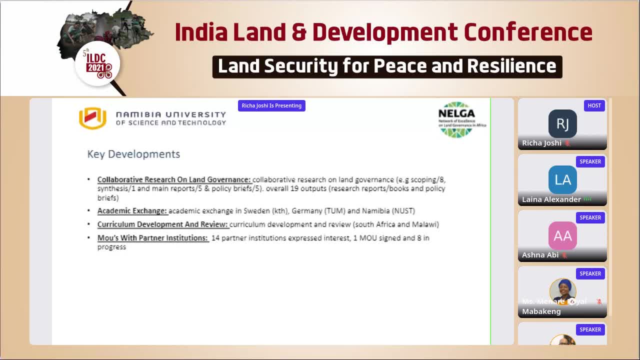 There's been collaborative research on land governance. Academic exchange is where the university has had other teams exchange students from Sweden in Sweden, uh Germany and and uh Namibia. curriculum development and review between South Africa and Malawi. they've also uh been memorandum of understanding between 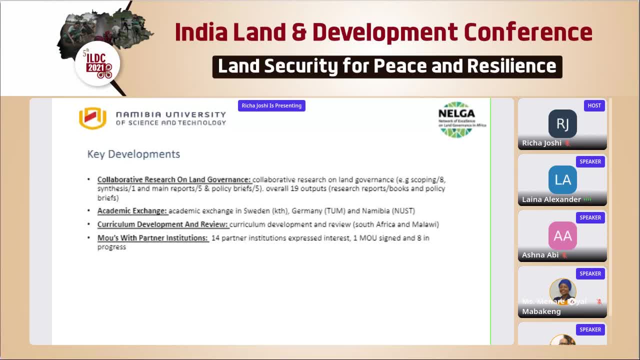 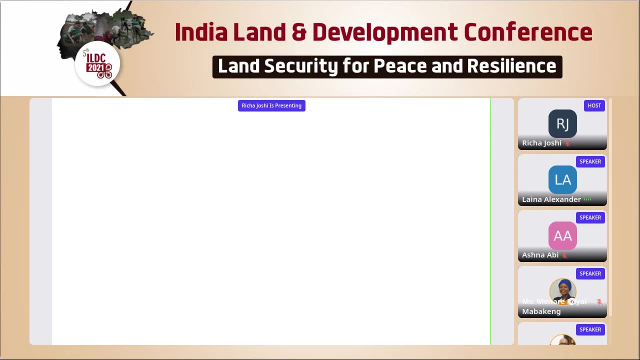 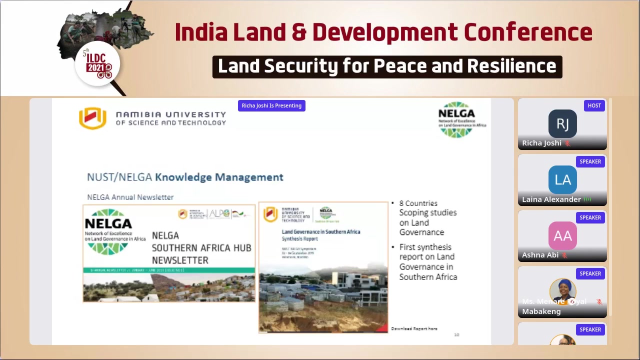 um other partner institutions, where 14 partner institutions expressed their interest, however, one only one memorandum of understanding was signed and the other eight are in progress. okay now, below here is the NELGA annual newsletter. um, they have been on eight. eight countries scoping studies on land governance and then the first synthesis report on land governance in southern 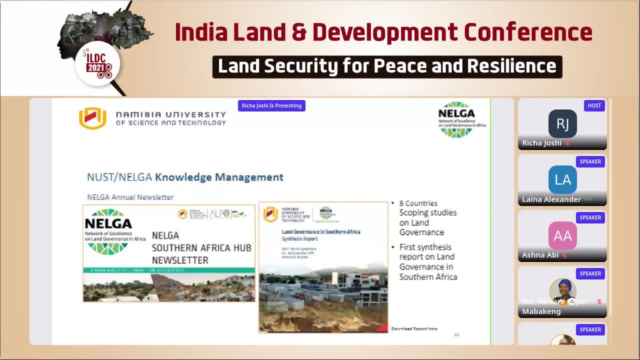 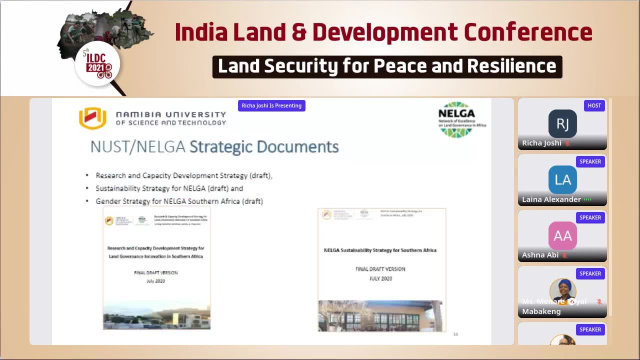 Africa, which will be launched at the conference that I'll I'll later I'll later discuss next slide. so NERST and NELGA have um conducted, have done a few studies and these are the, the, the documents that were basically that out, the outcomes of these studies. where there's 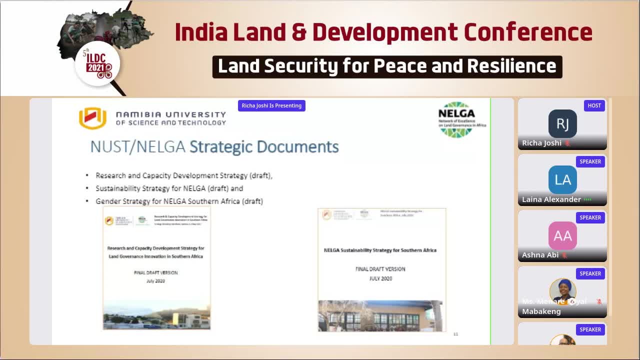 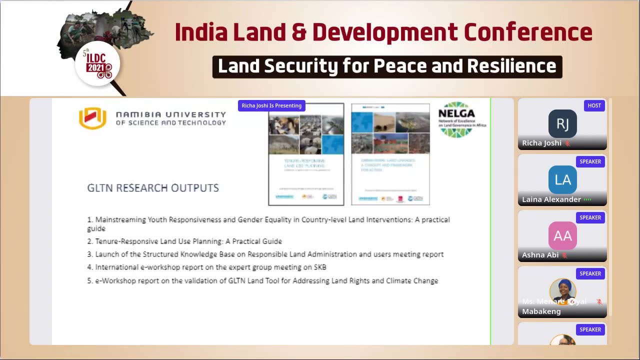 a draft on research and capacity development strategy, another draft on sustainability strategy for NELGA and, lastly, the gender strategy for NELGA. southern Africa. NERST has also worked with uh, JLTN and uh. the following are the outputs or the documents that we're. 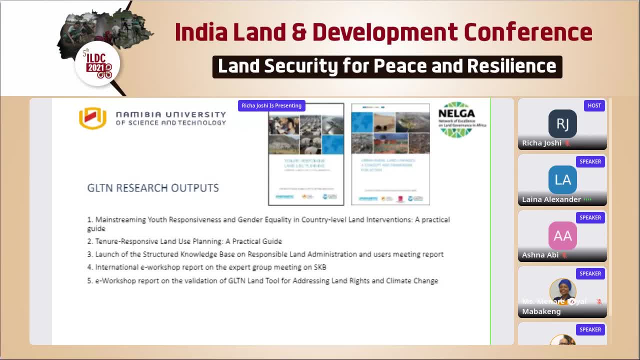 that were produced from this partnership. we have the mainstreaming uh, youth responsiveness and gender equality, and count on country level land interventions is a practical guide. and secondly, there is a tenure responsive language planning, which is also a practical guide. and the third is the launch of the. there was a report on the. 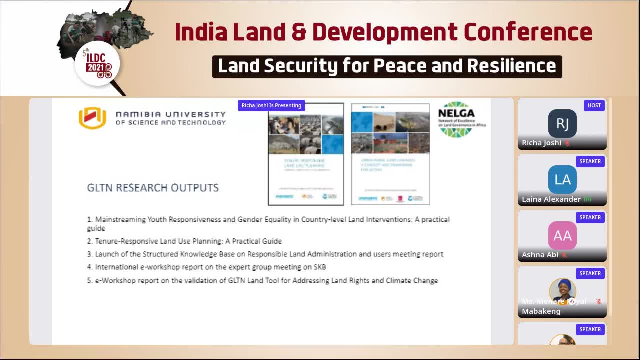 on the launch of, on the launching of the structured knowledge based on responsible land administration, which was um, which was launched by NERST in august, and then there's been also an international a report on the international e-workshop with regards to struck, the structured knowledge base, and uh. 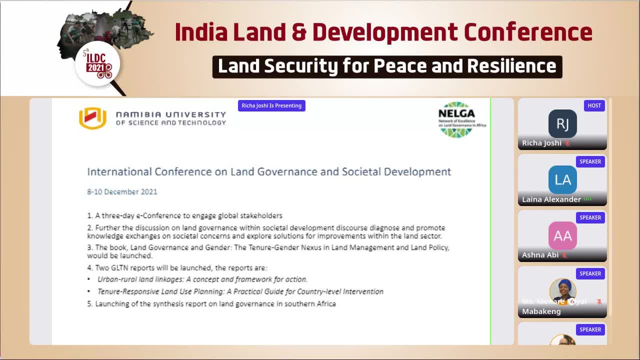 currently, NERST is busy organizing a conference that is in con, in collaboration with the Hansa Ito foundation. this conference will be on the will be on from the 8th to the 10th of december this year. so this what this conference is all about. 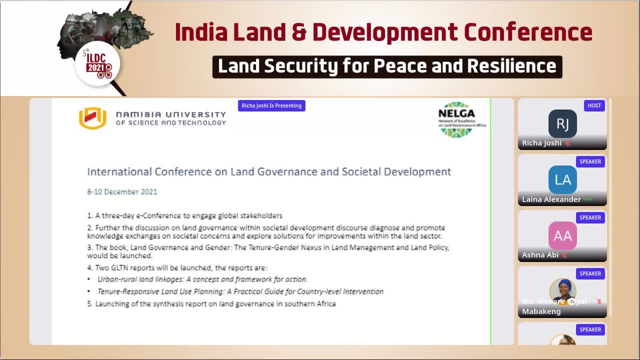 is to engage global stakeholders and also to further the discussion on land governance within societal development discourse and also promote knowledge exchanges on social concerns and explore solutions in order to improve, to to improve certain things in the land sector. now, in this, in this conference, there's a lot of work to be done in the field of land governance, so we're going to 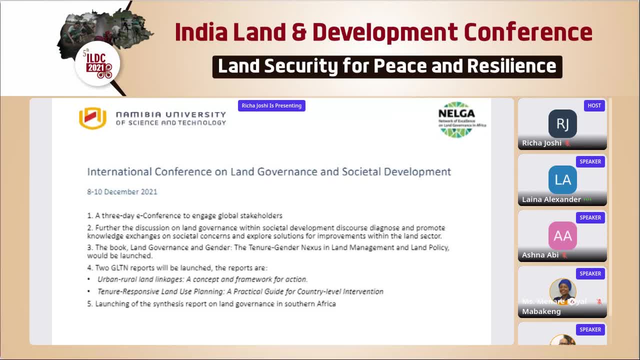 also be the launching of the book that is, on the 10, the land, land governance and gender, the 10-year agenda nexus in land management and land policy, which um was was written by our professor Chibu and um. there'll also be the launching of the two JLTN reports. 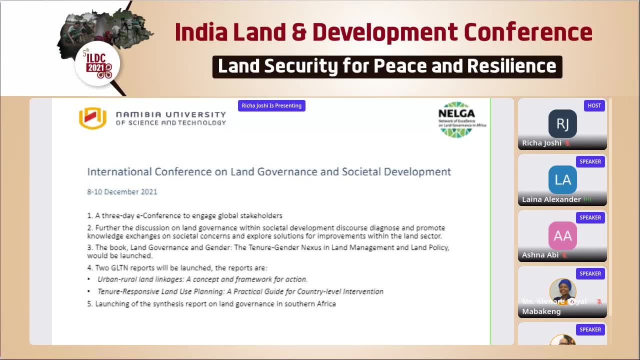 one on urban- rural land linkages: a concept and framework for action. and, lastly, the 10-year agenda on land governance in southern africa, which is a practical guide for country level intervention, and there will also be the launching of the synthesis report on land governance in. 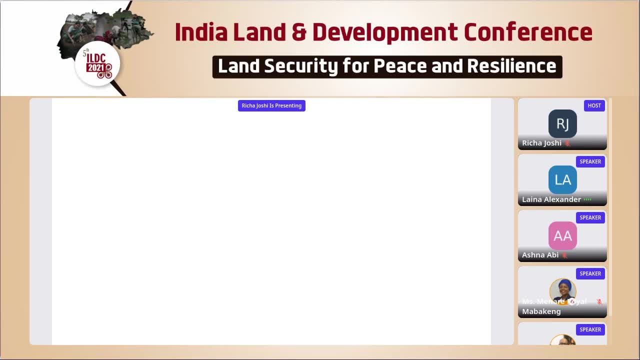 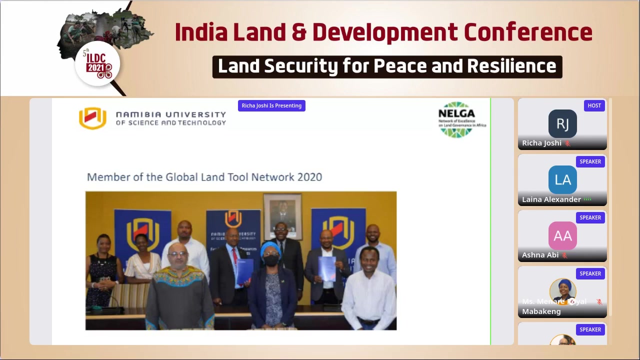 southern africa. yes, so this is the, the book that will be launched during the conference that is, that you are currently preparing for, and then, actually in the next few weeks, we will also be available for Q&A. so you can be sure that you are cukur and we will be back on time to have this conversation. 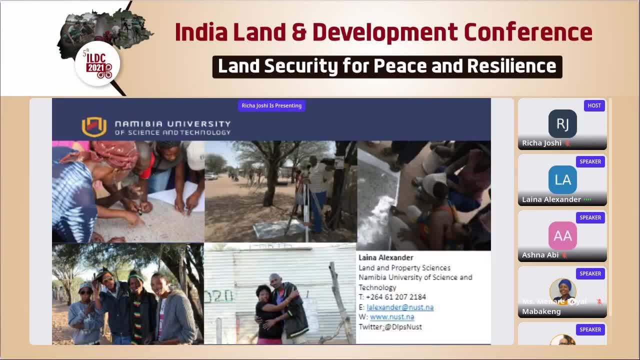 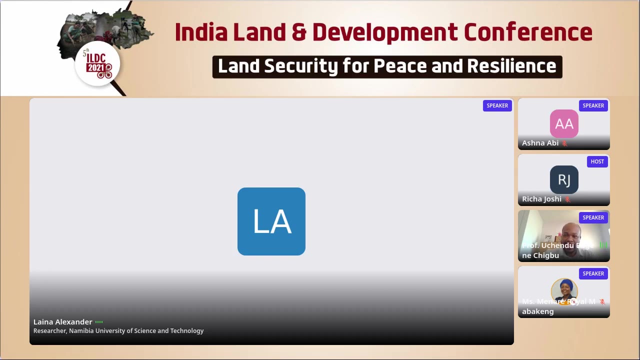 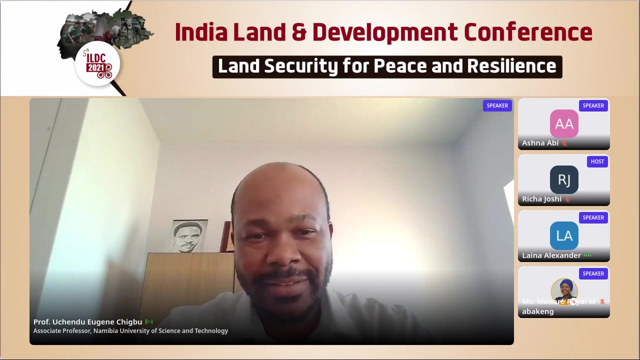 okay, in the picture below, these are the members of the JLTN network from the university, from the namibia university of science and technology. thanks very much, uh. thanks very much, liner and um. I just want to say um, for those who are not conversant with some of the um, the terminologies and abbreviations, um the gltn she was talking. 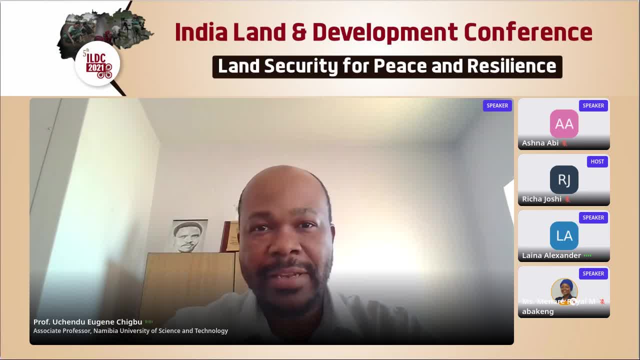 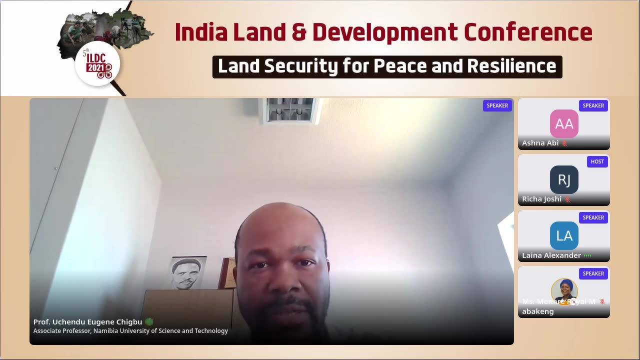 about is the global lantern Network, which is hosted by the UN habitats and, yeah and uh, nelga is a network of excellence in lands on land governance in Africa, which is um an African Union endorsed um continental Network um specifically put in place to improve the capacity in terms of Lance land management, land policy, land governance and land administration. 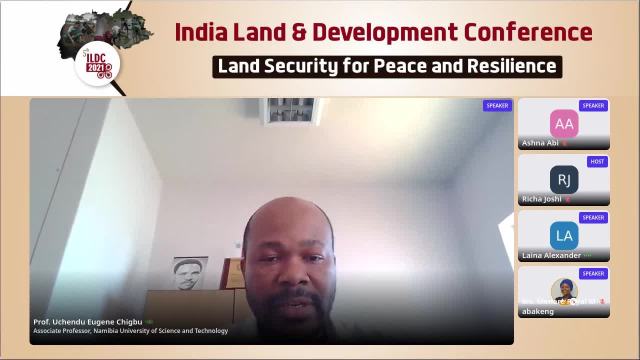 and within this uh, within this Network, you have about um five regional clusters within the, within the continent of Africa and within the southern part of Africa. Nost is the hub or the node, I also like to call it, which means that Nost is the headquarters for land governance, capacity building and activities here in southern Africa. now, um. 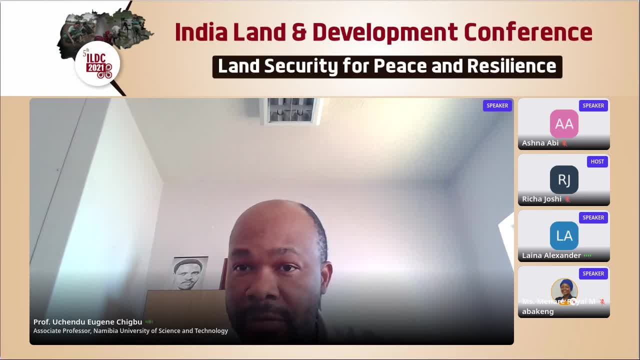 thank you, Lena. um, I left a message. anyone who wants to ask a question can always leave a message in the chat and we will continue. I will continue. we delve straight into the tenor- responsive land use planning, which liner mentioned just before she closed our presentation, but would make out ample time for any discussions or emerging issues that will arise afterwards. so 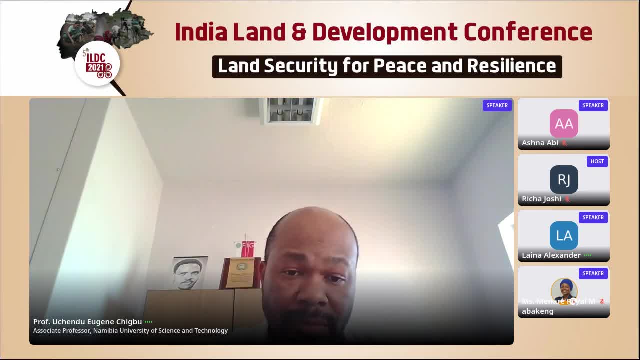 with that, um, I would move on to present the next parts of the next presentation in this session. I'm waiting for my script, my screen, to be shared. please let me know when you can see my screen, thank you, thank you, I'm still waiting. sorry for that, but this is pretty slow. 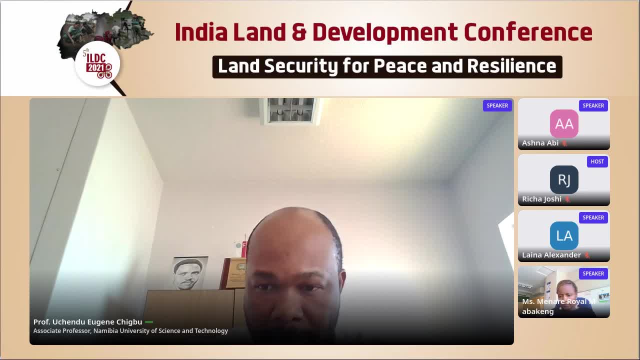 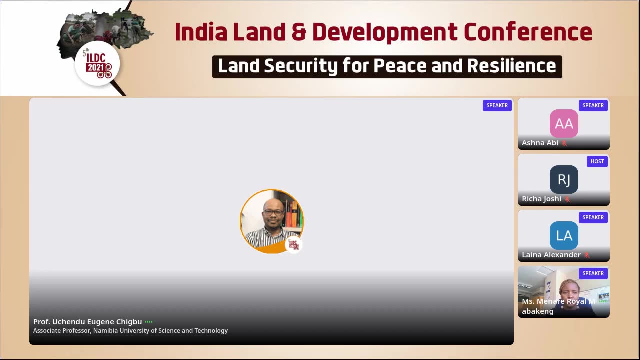 foreign, foreign, the slow you. I'm not sure you have my presentation, do you? uh? sir, I don't have. can you please, uh send, uh, send me the email address. I'm doing that. you do you have that of my colleague, Miss Royal, you can you? you? you? 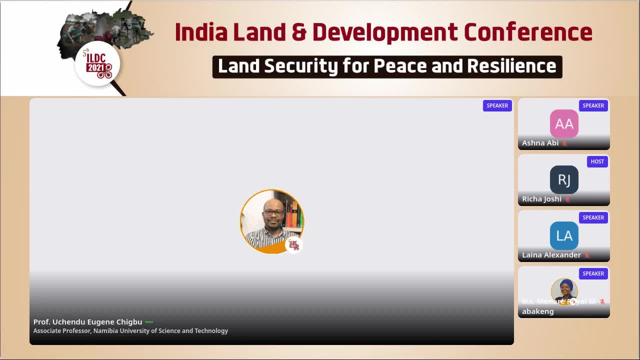 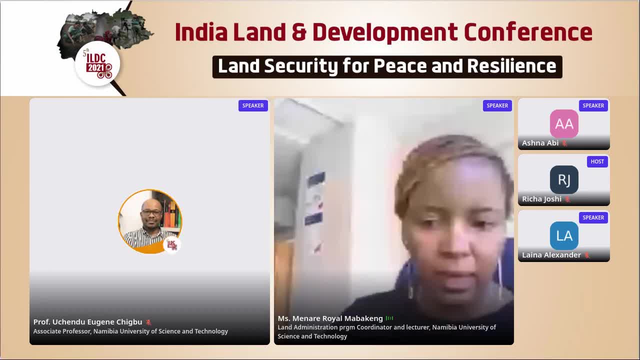 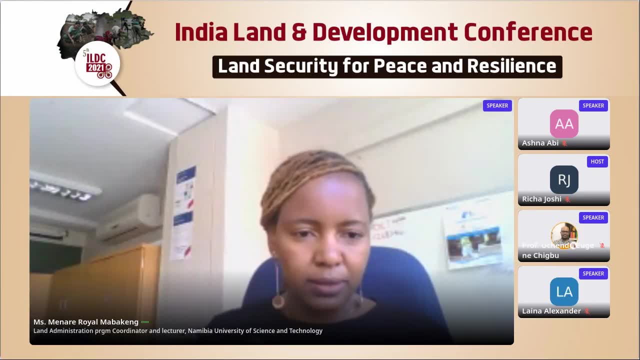 if, if, if, if, if i may uh go ahead with my, if i may uh go ahead with my, if i may uh go ahead with my presentation, presentation, presentation, um, i'm sure it will sort of link well in together with yours, sort of link well in together with yours. 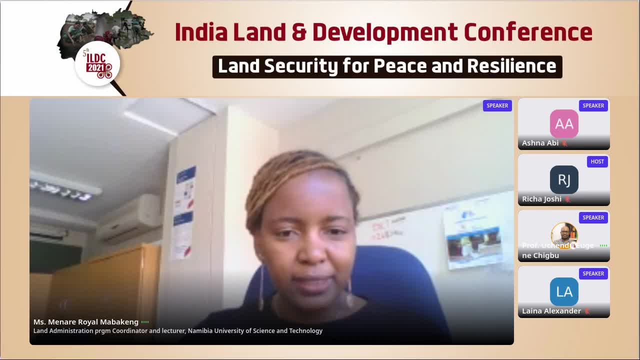 sort of link well in together with yours, once the technical issues um, once the technical issues um, once the technical issues um are addressed. you can go on, but i've seen the. you can go on, but i've seen the. you can go on, but i've seen the presentation. 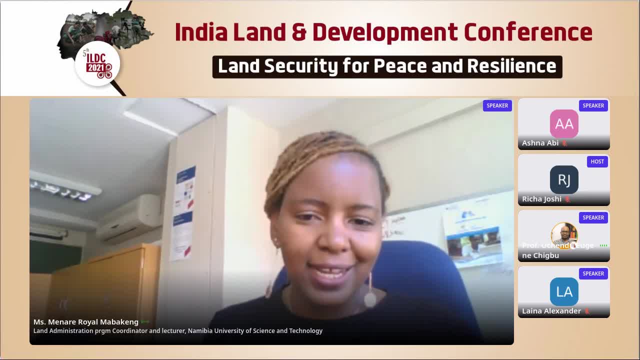 okay, um, the disadvantage of this is that, okay, um, the disadvantage of this is that, okay, um, the disadvantage of this is that i can't see, i can't see, i can't see. the audience, the audience, the audience, but the audience can see me, so just let 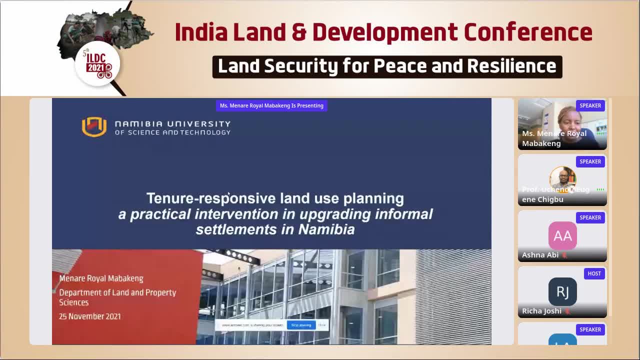 but the audience can see me, so just let but the audience can see me, so just let me know if you can see my presentation um. i have shared my screen. can you see my um? i have shared my screen. can you see my um? i have shared my screen. can you see my presentation? 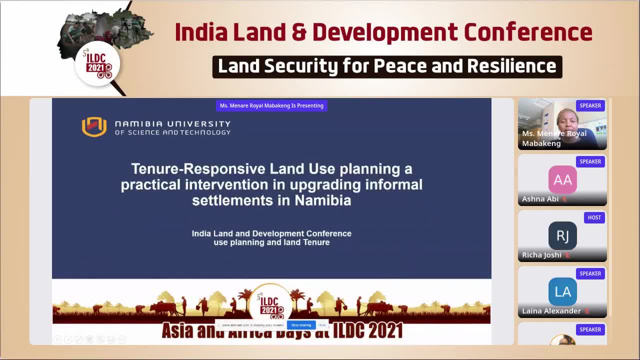 yes, i can, yes, i can, yes, i can, okay, okay, okay, all right, so um, today i'm going to speak all right, so um, today i'm going to speak all right, so um, today i'm going to speak about tenure, about tenure, about tenure: responsive land use planning: a practical 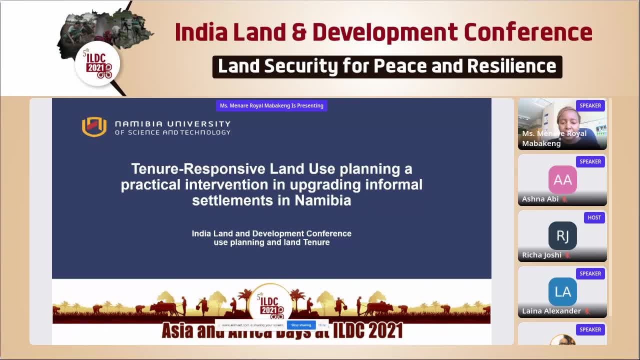 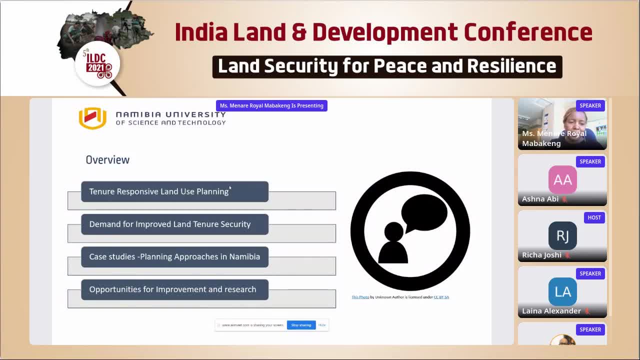 so just to start off the conversation, i so just to start off the conversation, i would want to, would want to, would want to. i'm going to do a brief overview in terms. i'm going to do a brief overview in terms. i'm going to do a brief overview in terms of what is senior responsive language. 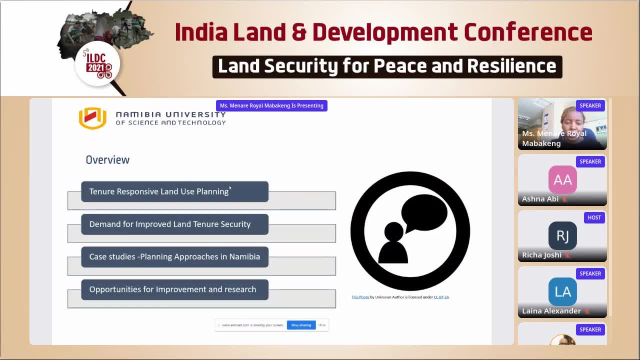 of what is senior responsive language, of what is senior responsive language: planning, planning, planning. uh, from my perspective, i'm mostly uh. from my perspective, i'm mostly uh. from my perspective, i'm mostly informed by, informed by, informed by the material that has been produced, by the material that has been produced by. 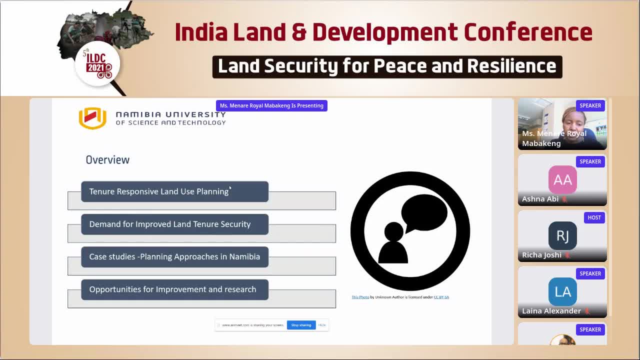 the material that has been produced by the global land tool network, the global land tool network, the global land tool network, and led by professor chiku here who's, and led by professor chiku here who's, and then going into some of the planning. and then going into some of the planning. 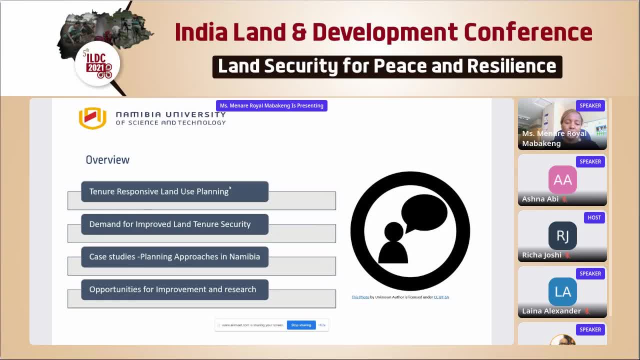 and then going into some of the planning approaches, specifically approaches, specifically approaches specifically towards um or related to informal towards um or related to informal towards um or related to informal settlement upgrading, settlement, upgrading, settlement, upgrading here, and then i'll close off the here and then i'll close off the. 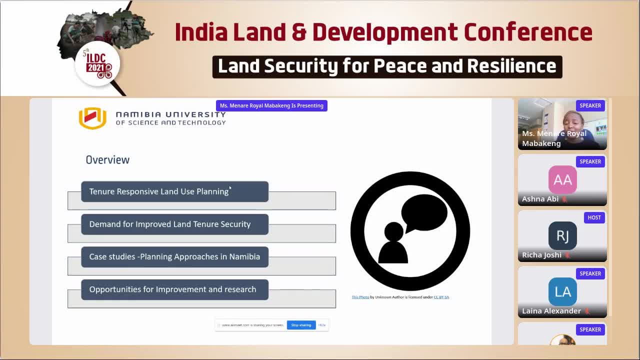 here and then i'll close off the presentation presentation. presentation with opportunities for improvement and with opportunities for improvement and with opportunities for improvement. and research, research, research in what we can do as an institution and in what we can do as an institution, and in what we can do as an institution, and then also as a country. 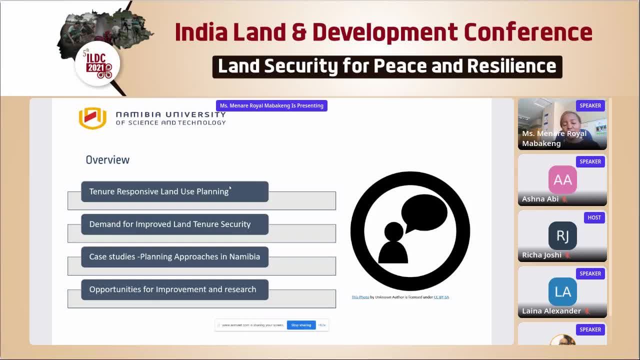 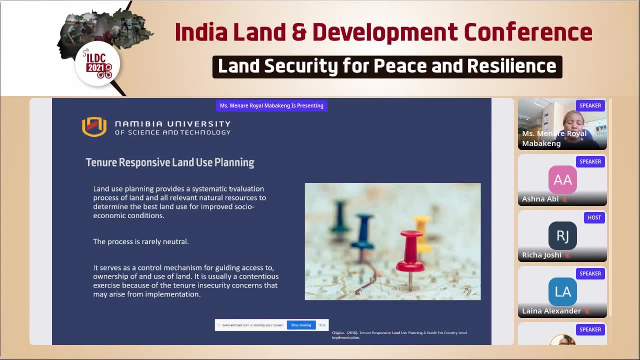 then also as a country, then also as a country in promoting um tenure responsive land, in promoting um tenure responsive land, in promoting um tenure responsive land use planning, use planning, use planning. so itania responsive land use planning. so itania responsive land use planning. so itania responsive land use planning. um comes as an intervention, um or at 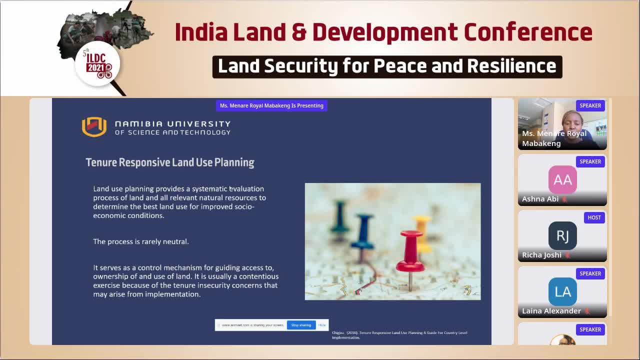 um comes as an intervention, um or at. um comes as an intervention, um, or at least, as least, as least as as a term and a concept that has been as a term and a concept that has been as a term and a concept that has been proposed by the global rental network. 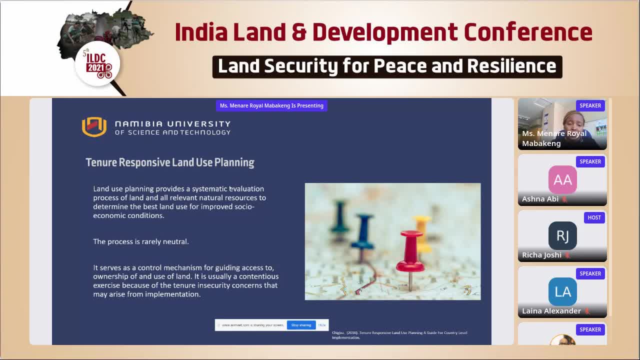 proposed by the global rental network. proposed by the global rental network. and is adopted and implemented uh in: and is adopted and implemented uh in. and is adopted and implemented uh in various countries, various countries, various countries, as we most, as all of us, would know land, as we most, as all of us, would know land. 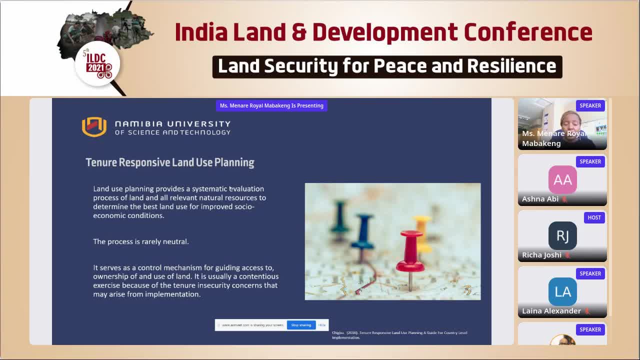 as we most, as all of us would know, land use planning provides a systematic use planning. provides a systematic use planning, provides a systematic evaluation process, evaluation process, evaluation process of land and all relevant natural of land and all relevant natural of land and all relevant natural resources. resources. 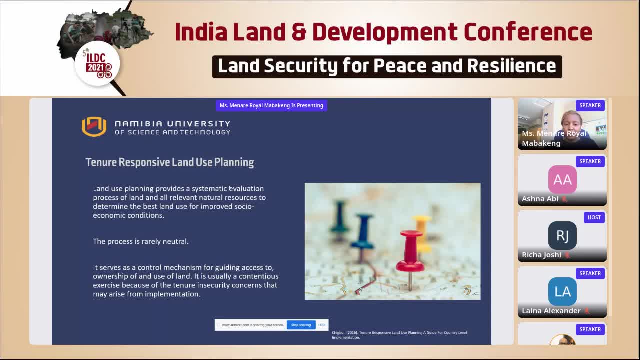 resources to determine the best land use for. to determine the best land use for, to determine the best land use for improved socioeconomic conditions- improved socioeconomic conditions, improved socioeconomic conditions. but then this process is really neutral. but then this process is really neutral. but then this process is really neutral because you always have to decide. 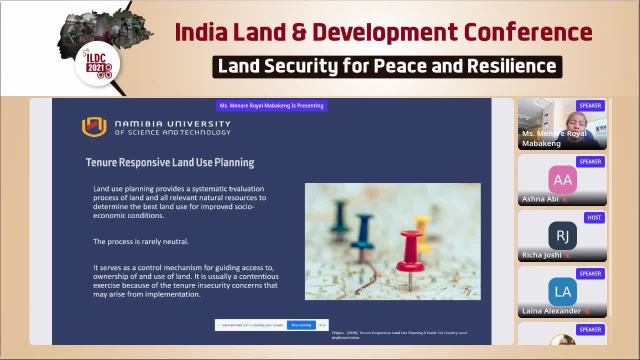 because you always have to decide. because you always have to decide what would be the best option for um the? what would be the best option for um the? what would be the best option for um the community? the best option for the local community, the best option for the local. 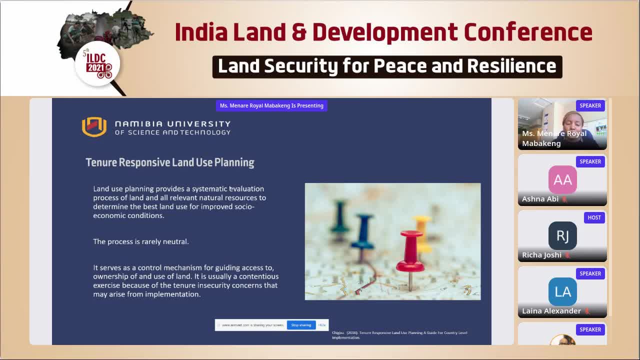 community. the best option for the local council, council, council. or the best option that whoever has the, or the best option that whoever has the, or the best option that whoever has the control, control, control of the planning um teams to be the best of the planning um teams to be the best. 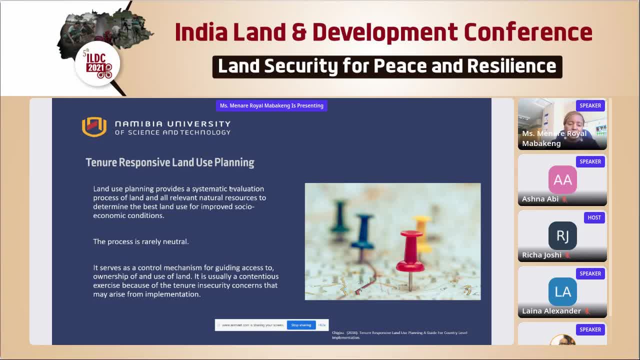 of the planning um teams to be the best. so in most time there will be a cost. so in most time there will be a cost. so in most time there will be a cost benefit: where you benefit, where you benefit, where you, where one um party would lose or another. 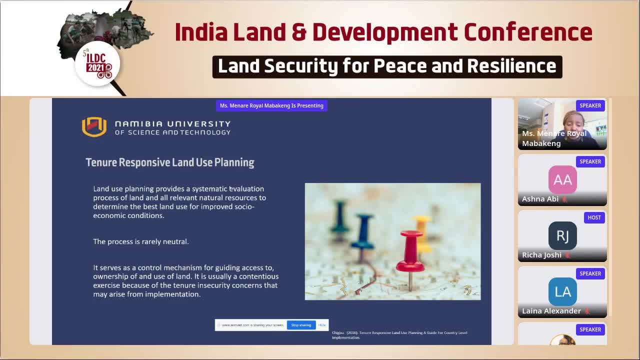 where one um party would lose or another. where one um party would lose or another, one would gain. one would gain, one would gain. land use planning serves as a control. land use planning serves as a control. land use planning serves as a control. mechanism for guiding, mechanism for guiding. 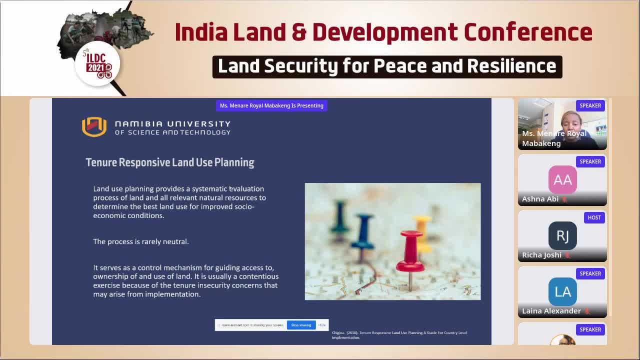 mechanism for guiding access to ownership of and use of land. access to ownership of and use of land. access to ownership of and use of land, and it is usually a contentious exercise. and it is usually a contentious exercise. and it is usually a contentious exercise because of the tenure insecurity. 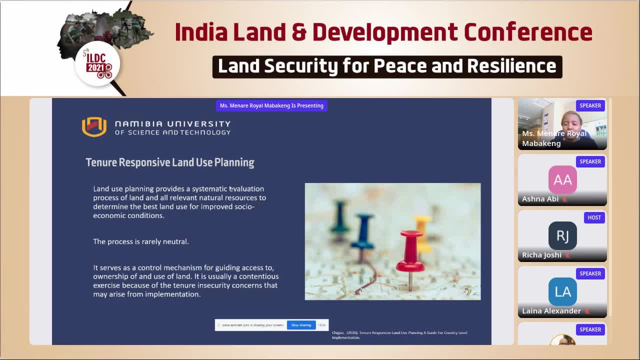 because of the tenure insecurity, because of the tenure insecurity concerns that may arise from its concerns, that may arise from its concerns that may arise from its implementation, implementation, implementation, and this we have observed in our and this we have observed in our and this we have observed in our research, that 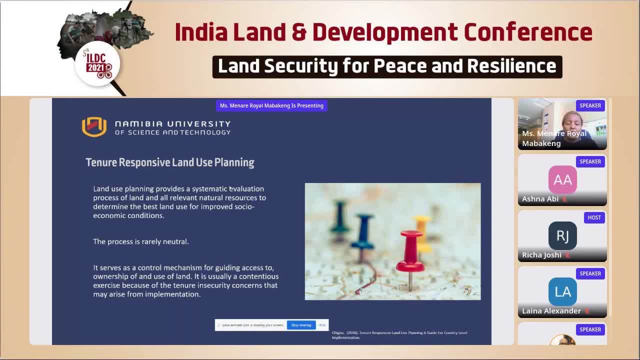 research that research that when there is a proposal to upgrade, or when there is a proposal to upgrade, or when there is a proposal to upgrade or plan a specific area- plan a specific area, plan a specific area- it does raise this concern around tenure. it does raise this concern around tenure. 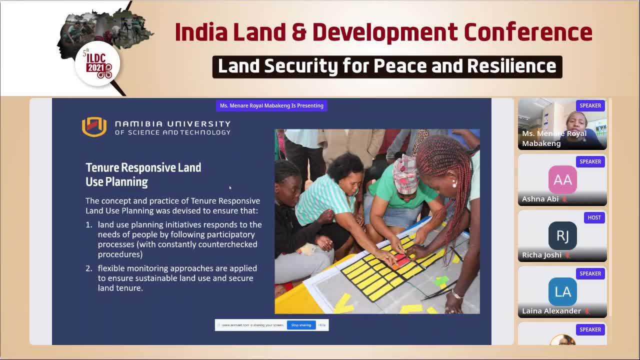 it does raise this concern around tenure, insecurity, insecurity, insecurity, so what what? the concept of tenure so what? what? the concept of tenure so what? what? the concept of tenure? responsive land use friend planning. responsive land use friend planning. responsive land use friend planning brings as a solution especially to the 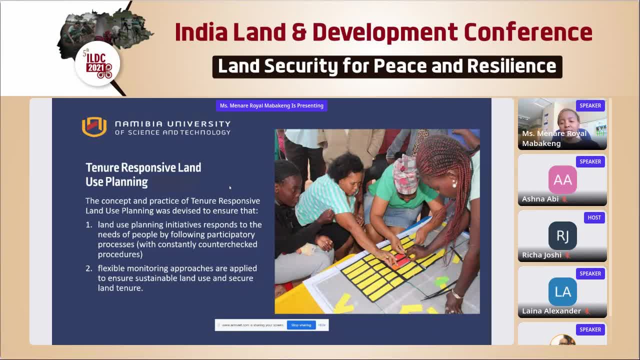 brings as a solution, especially to the, brings as a solution especially to the aspect of tenure insecurity, aspect of tenure insecurity, aspect of tenure insecurity. that seems to be very common in most, that seems to be very common in most, that seems to be very common in most informal settlements. 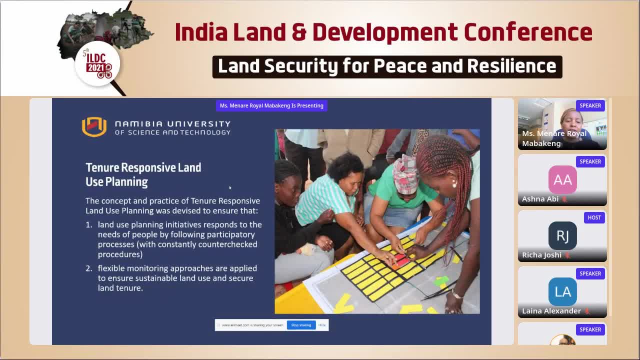 informal settlements. informal settlements: is that it it it provides or ensures? is that it it provides or ensures? is that it it provides or ensures that land use planning, that land use planning, that land use planning initiatives respond to the needs of the initiatives, respond to the needs of the. 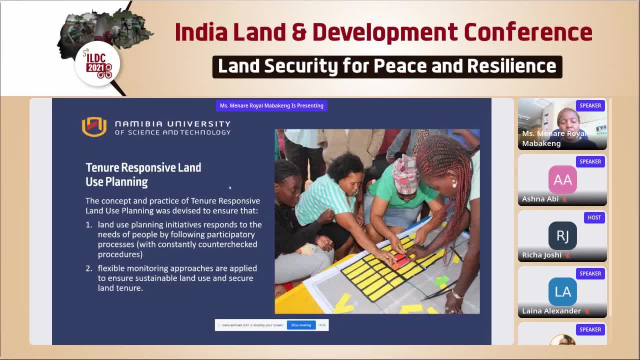 initiatives respond to the needs of the people, people, people by following a participatory process, by following a participatory process, by following a participatory process which is constantly counted, which we've, which is constantly counted, which we've, which is constantly counted, which we've constantly counter checked procedures. 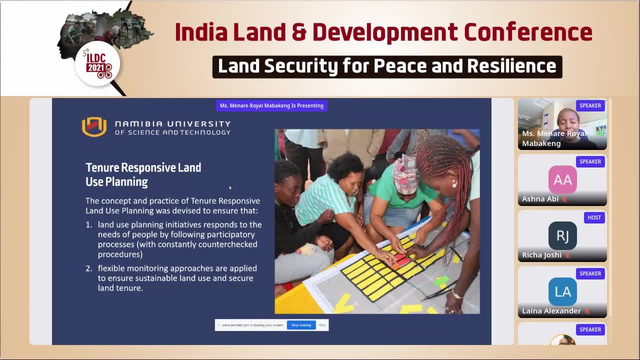 constantly counter checked procedures. constantly counter checked procedures. what we have seen uh at least in my, what we have seen uh at least in my, what we have seen uh at least in my experience, and a colleague of mine uh experience and a colleague of mine uh experience and a colleague of mine uh within the faculty, also did mention that 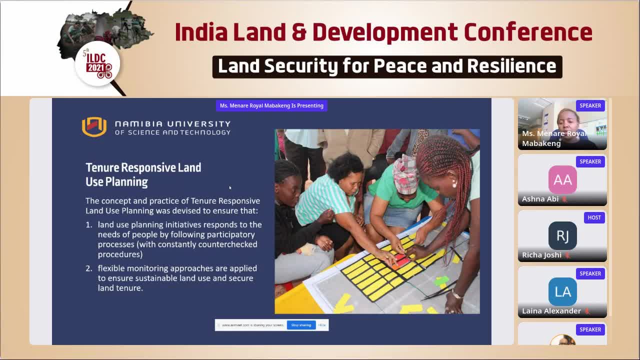 within the faculty also did mention that within the faculty also did mention that it is not something that is well, it is not something that is well, it is not something that is well received, received, received when um, at least from our observation, when um, at least from our observation. 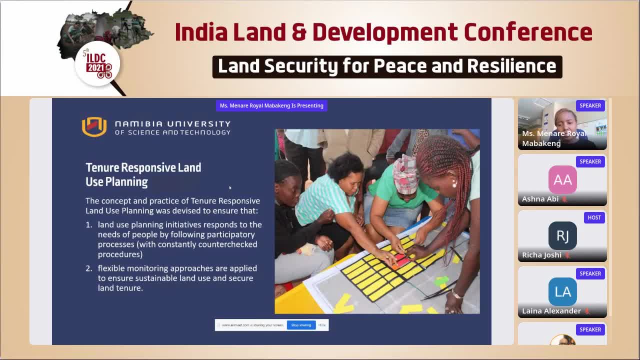 when? um, at least from our observation, mine specifically, having worked in this mine, specifically having worked in this mine, specifically having worked in this sector for the past 10 years, sector for the past 10 years, sector for the past 10 years- is that when you, when, when there is 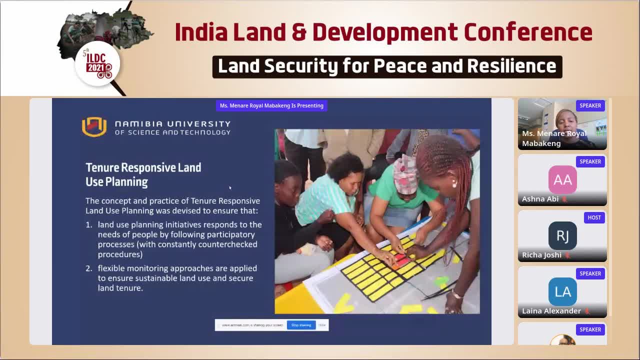 is that, when you, when, when there is? is that when you, when, when there is planning for informal settlements, planning for informal settlements, planning for informal settlements? there is a, an approach where there is a, an approach where there is a, an approach where planning is uh, or at least town planners. 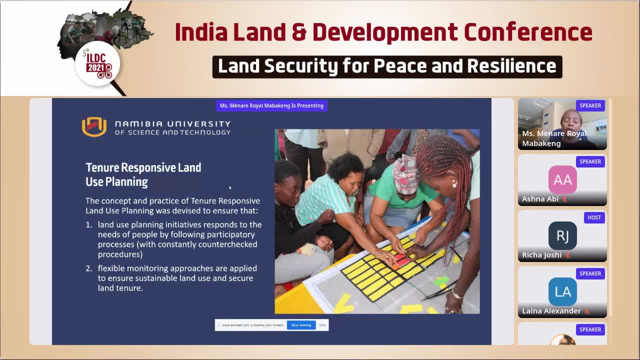 planning is uh, or at least town planners planning is uh, or at least town planners from. from, from my view. get to plan for from from from my view. get to plan for from from from my view. get to plan for people rather than with people. so what? people rather than with people, so what? 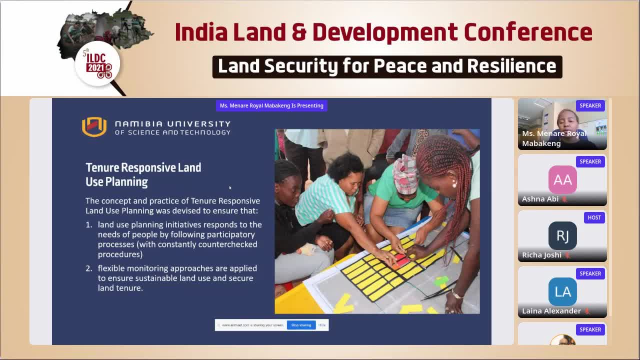 people rather than with people. so what? tenure- responsive land use planning. tenure- responsive land use planning. tenure- responsive land use planning brings forward, is a different approach. brings forward is a different approach. brings forward is a different approach. where the planning is with the with the. where the planning is with the with the. 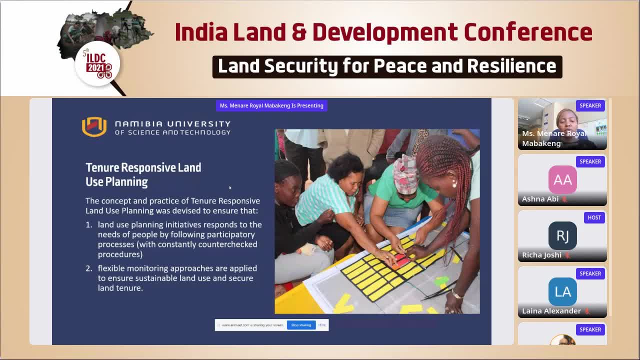 where the planning is, with the, with the people, people, people. tenure responsive land use planning also. tenure responsive land use planning also. tenure responsive land use planning also provides, provides, provides flexible monitoring approaches that can flexible monitoring approaches that can flexible monitoring approaches that can be applied in any project in order to 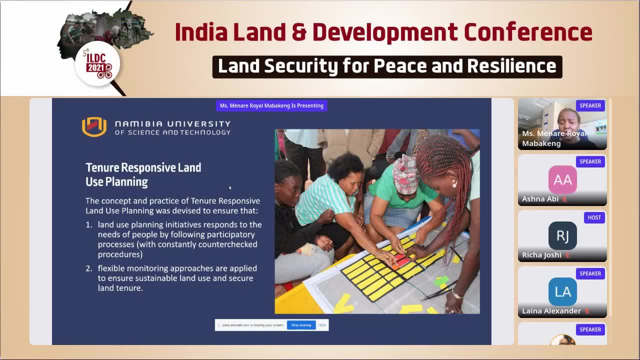 be applied in any project in order to be applied in any project in order to ensure, ensure, ensure sustainable land use and then also secure sustainable land use, and then also secure sustainable land use and then also secure land tenure, land tenure, land tenure. when we, when we look at uh land use, 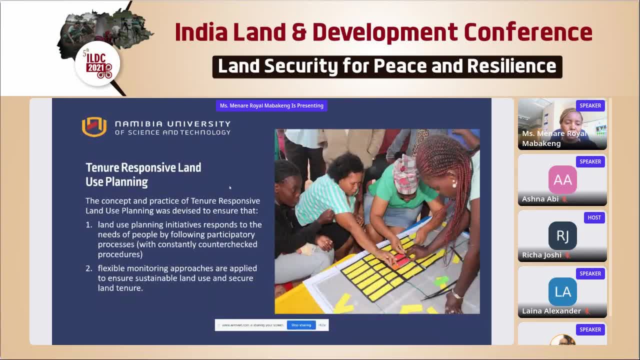 when we, when we look at uh land use, when we, when we look at uh land use, planning approaches, planning approaches, planning approaches: uh within um within most urban centers, uh within um within most urban centers, uh within um within most urban centers, and especially in namibia, although, 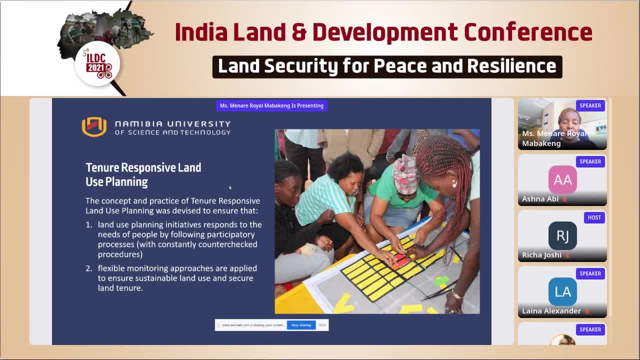 and especially in namibia, although, and especially in namibia, although- there's currently a shift, there's currently a shift. there's currently a shift uh to ensure that we have uh participatory uh, to ensure that we have uh participatory uh, to ensure that we have uh participatory approach. uh approaches is that: 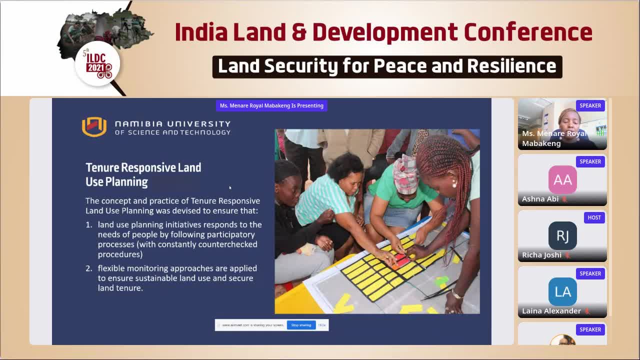 approach, uh approaches. is that approach, uh approaches? is that planning is always seen from the point. planning is always seen from the point. planning is always seen from the point of um restructuring the settlement of um restructuring, the settlement of um restructuring, the settlement for the community, rather than with the 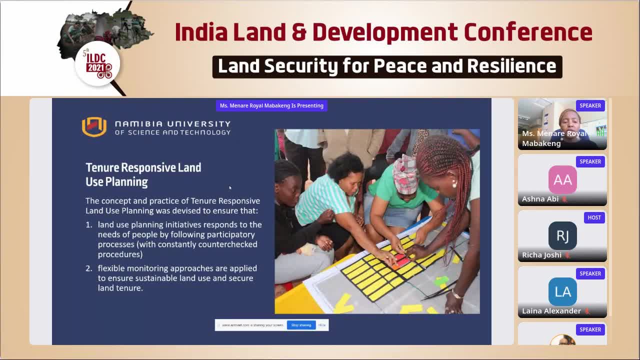 for the community rather than with the. for the community rather than with the community. community community. where the focus is now on the, where the focus is now on the, where the focus is now on the availing of our services and then also availing of our services and then also. 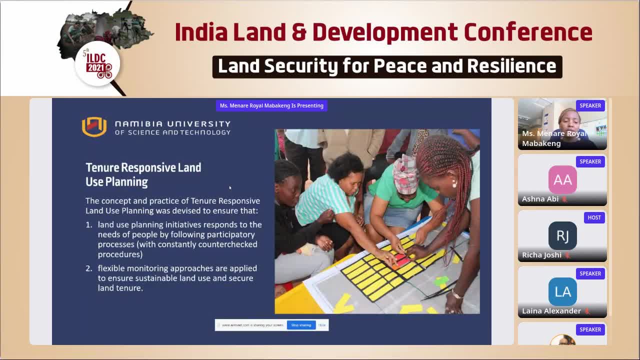 availing of our services. and then also the, the, the. you're just ensuring that you have a, you're just ensuring that you have a, you're just ensuring that you have a proper layout, proper layout, proper layout, um. in order to ensure that you have um, in order to ensure that you have more roads and access ways for. 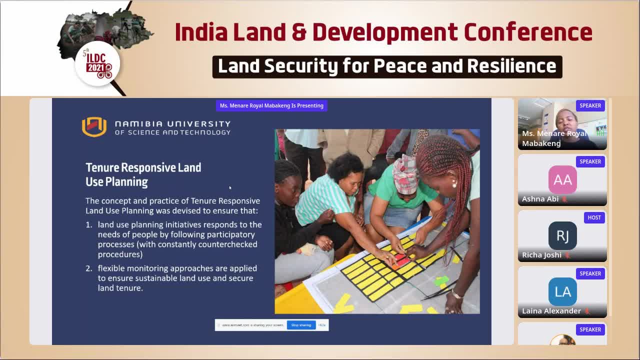 more roads and access ways for more roads and access ways for, for the community, however this, this for the community, however this, this for the community, however this, this planning approaches don't necessarily planning approaches, don't necessarily planning approaches don't necessarily always put, always put, always put the security of tenure of inhabitants at. 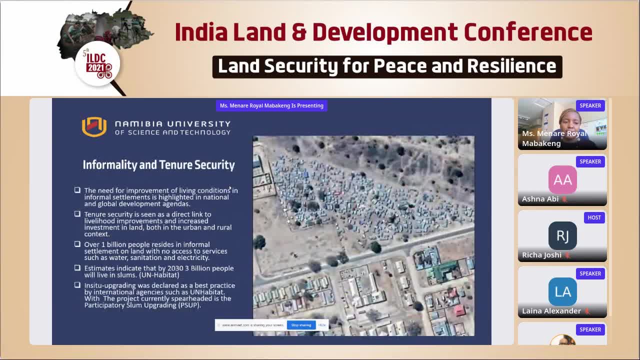 the security of tenure of inhabitants at the security of tenure of inhabitants at the center, the center, the center. so what do we have as experiences within? so, what do we have as experiences within? so what do we have as experiences within the media, the media, the media. there is a need for improvement of living. 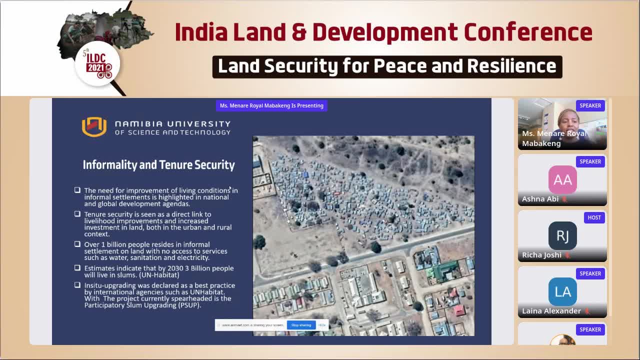 there is a need for improvement of living, there is a need for improvement of living conditions and informal settlement conditions and informal settlement conditions and informal settlement. and this is highlighted in national and, and this is highlighted in national and, and this is highlighted in national and global agendas. if we look at the uh, the, 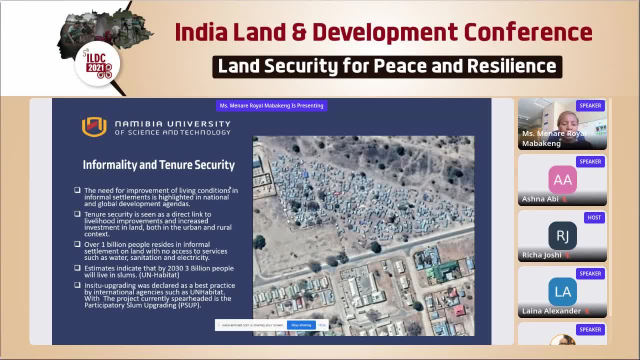 global agendas. if we look at the uh- the global agendas. if we look at the uh- the sustainable development goals- sustainable development goals, sustainable development goals. they are, there are specific objectives, they are, there are specific objectives, they are, there are specific objectives that do that, do that, do focus on um ensuring that there is an 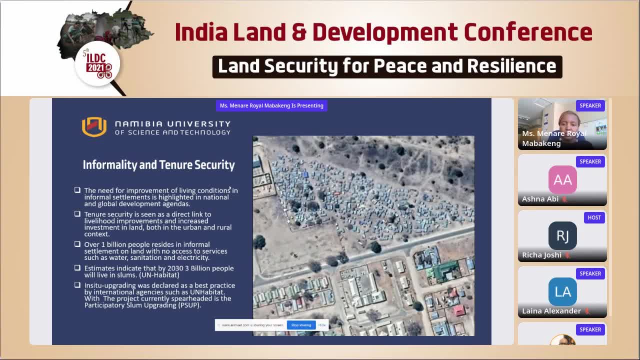 focus on um ensuring that there is an focus on um, ensuring that there is an improvement of, improvement of, improvement of of living conditions and reduction of of living conditions and reduction of of living conditions and reduction of poverty, which are most poverty, which are most poverty, which are most of the time linked, which is linked to um. 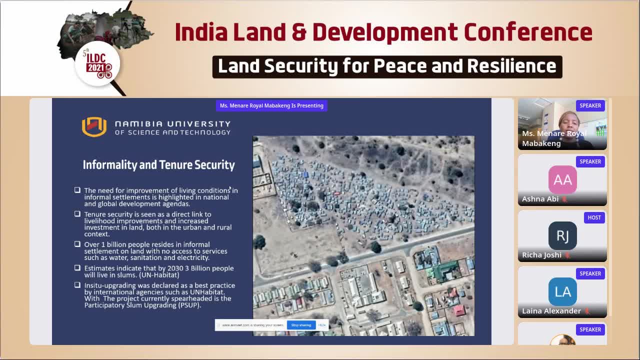 of the time linked which is linked to um. of the time linked which is linked to um. security of tenure, security of tenure, security of tenure. and because tenure security is seen as a and because tenure security is seen as a and because tenure security is seen as a direct link to the improvement of. 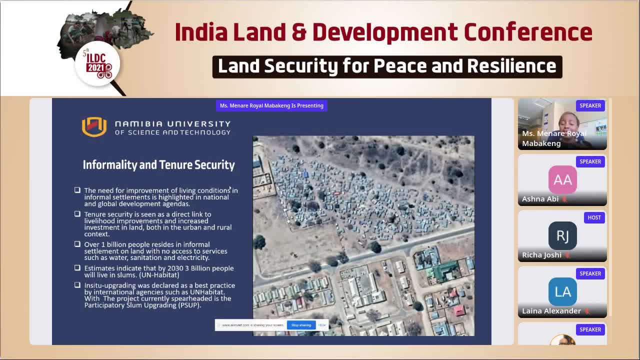 direct link to the improvement of, direct link to the improvement of livelihoods, livelihoods, livelihoods. because when you have uh an increase in, because, when you have uh an increase in, because when you have uh an increase in tenure security, tenure security, tenure security, you would have an increase in uh. 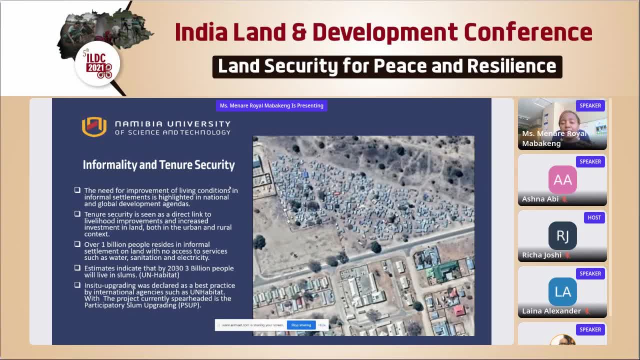 you would have an increase in uh. you would have an increase in uh investments. if you are talking from a investments, if you are talking from a investments, if you are talking from a rural, rural, rural perspective, and then also an improvement perspective, and then also an improvement perspective, and then also an improvement of. 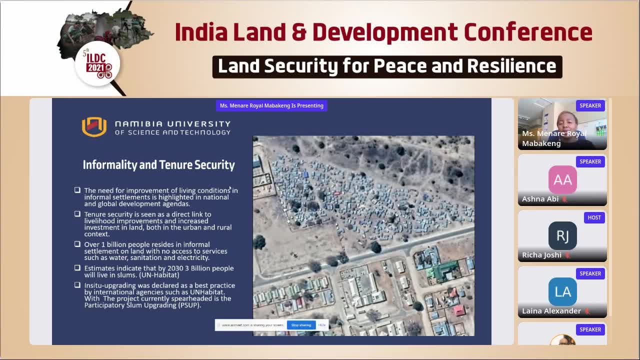 of of structures, if you are speaking from an structures, if you are speaking from an structures, if you are speaking from an urban, urban, urban land perspective, specifically for informal land perspective, specifically for informal land perspective, specifically for informal settlements, when we speak about settlements, when we speak about 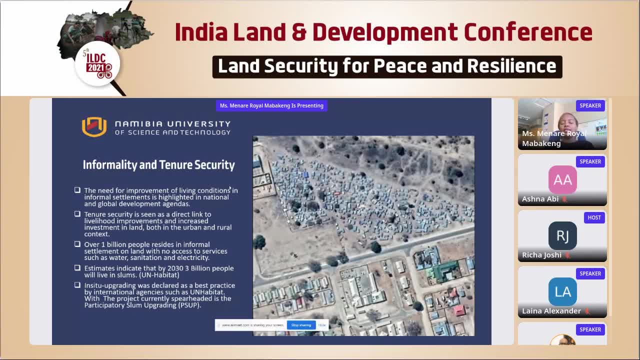 settlements. when we speak about tenure security, we don't necessarily tenure security. we don't necessarily tenure security. we don't necessarily mean that it is the issuing of title d, mean that it is the issuing of title d, mean that it is the issuing of title d because tenure security can be perceived. 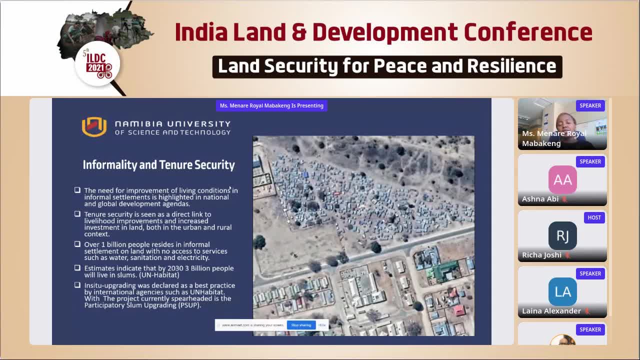 because tenure security can be perceived. because tenure security can be perceived um, as we have seen in research, but then um, as we have seen in research, but then um, as we have seen in research, but then tenure security is always highest when. tenure security is always highest when. 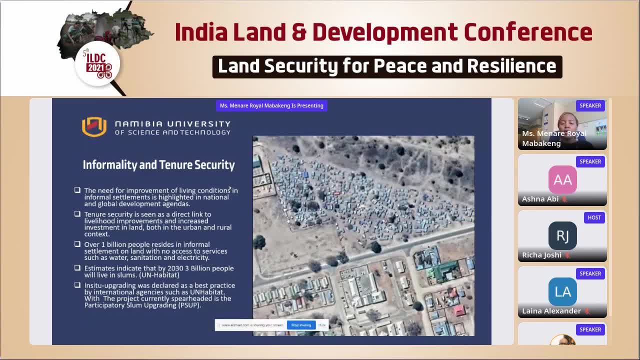 tenure security is always highest when there is there is there is a high buy-in, or at least a promotion. a high buy-in or at least a promotion. a high buy-in or at least a promotion of um reduction of evictions from from of um reduction of evictions from from. 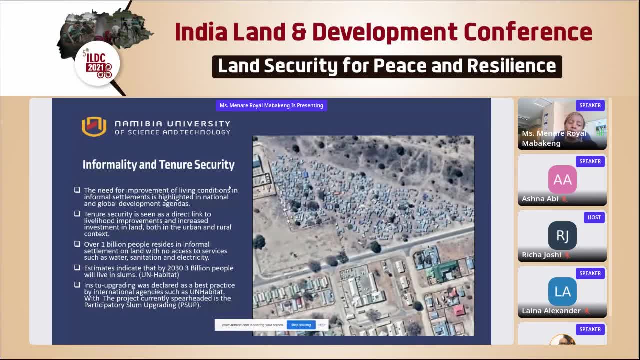 of um reduction of evictions from from that from the government, that from the government, that from the government. we we know that currently, at least from we. we know that currently, at least from we. we know that currently, at least, from the last estimates that were reported, the last estimates that were reported. 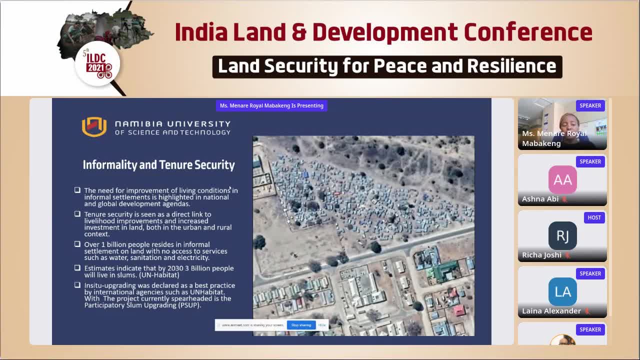 the last estimates that were reported, these are over 1 billion people, that these are over 1 billion people, that these are over 1 billion people that reside in informal settlements, reside in informal settlements, reside in informal settlements if we don't change our approaches. if we don't change our approaches. 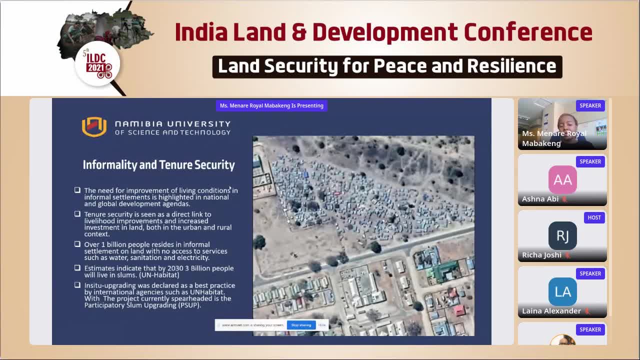 if we don't change our approaches, this, this number would increase by 3. this, this number would increase by 3. this, this number would increase by 3 billion, billion, billion. by 2030: what we see and and also what. by 2030: what we see and and also what. 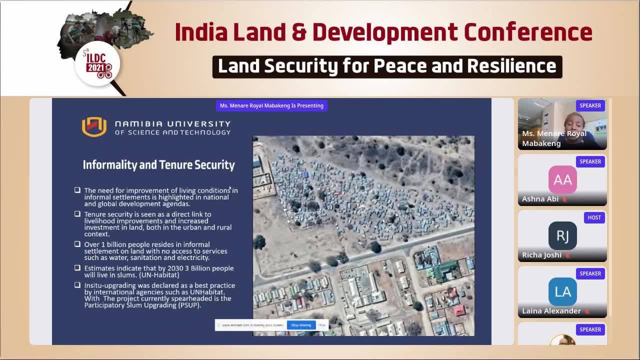 by 2030. what we see and and also what has been um identified by, has been um identified by. has been um identified by you inhabited and also promoted by the you inhabited and also promoted by the you inhabited and also promoted by the global lento network. 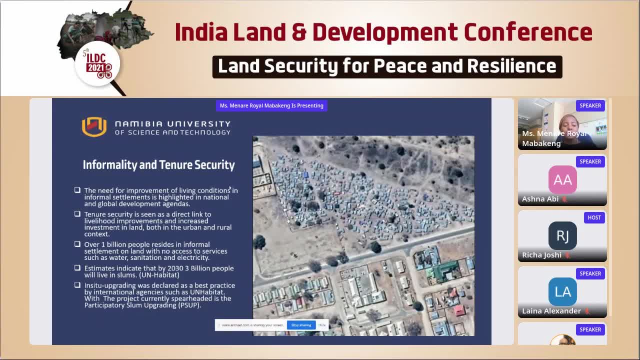 global lento network. global lento network is the aspect of uh in-situ upgrading, is the aspect of uh in-situ upgrading, is the aspect of uh in-situ upgrading which has been seen as a best practice. which has been seen as a best practice. 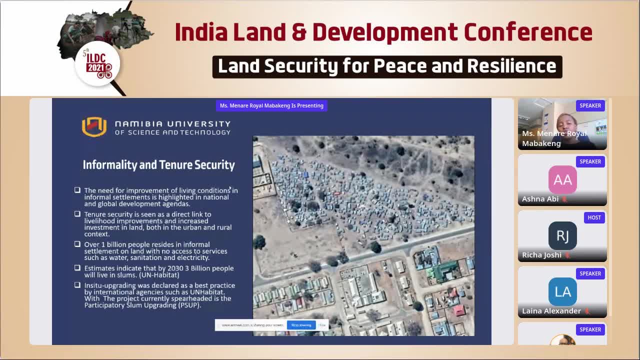 which has been seen as a best practice that can address the concerns of that, can address the concerns of that, can address the concerns of communities, communities, communities, because you address one, the needs of, because you address one, the needs of, because you address one, the needs of um, of inhabitants, with, with, uh. 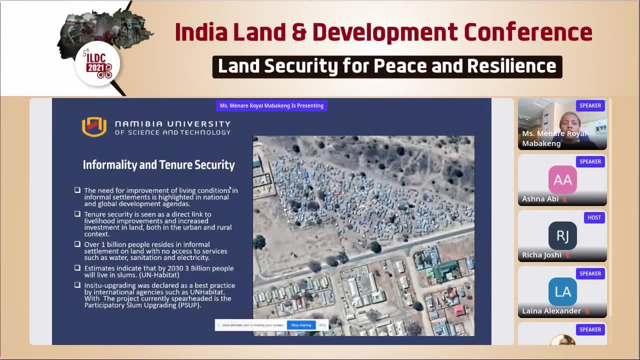 um of inhabitants with with uh, um of inhabitants with with uh, the the level of uh insecurity that they the the level of uh insecurity that they, the the level of uh insecurity that they are experiencing, are experiencing, are experiencing. you also start addressing what is their. you also start addressing what is their. 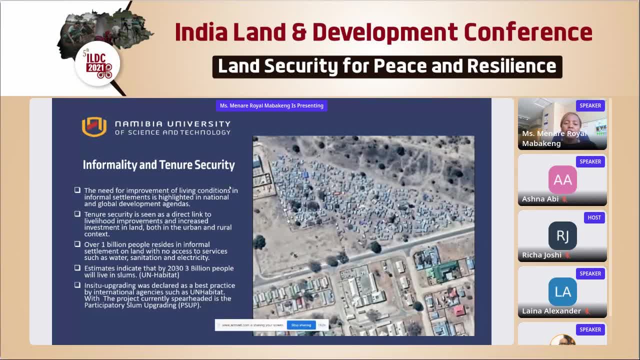 you also start addressing what is their development priorities. development priorities, development priorities because when you, when you have, because when you, when you have, because when you, when you have, approaches that focus, approaches that focus, approaches that focus more on um the sort of top-down, more on um the sort of top-down. 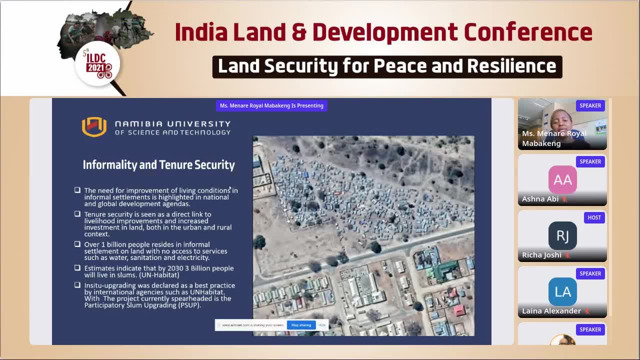 more on um, the sort of top-down approach to planning. sometimes what is approach to planning? sometimes what is approach to planning? sometimes what is implemented in an, implemented in an, implemented in an, won't necessarily come from what the won't necessarily come from what the won't necessarily come from what the community would deem as a priority. 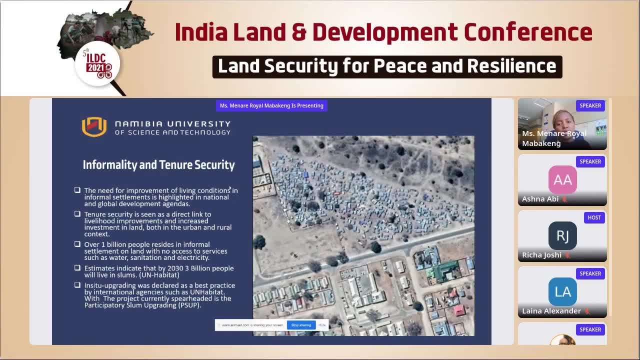 community would deem as a priority, community would deem as a priority and and most projects that we have seen, and and most projects that we have seen, and and most projects that we have seen in research, not only here in namibia, but in research, not only here in namibia, but. 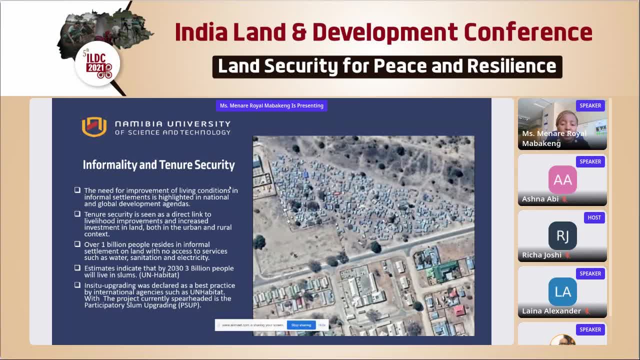 in research, not only here in namibia, but also some other case studies also, some other case studies, also some other case studies that we that we have come across um, that we that we have come across um that we that we have come across um, especially if we have examples um. 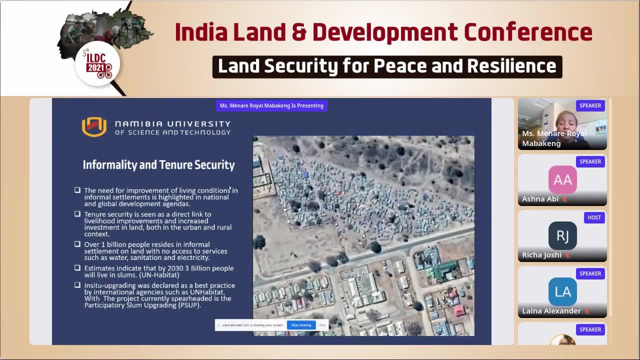 especially if we have examples um, especially if we have examples um some, some examples from south africa, as some, some examples from south africa, as some some examples from south africa as well. well, well, is that you have this um promotion? is that you have this um promotion? is that you have this um promotion of uh. improving the, the layout improving. 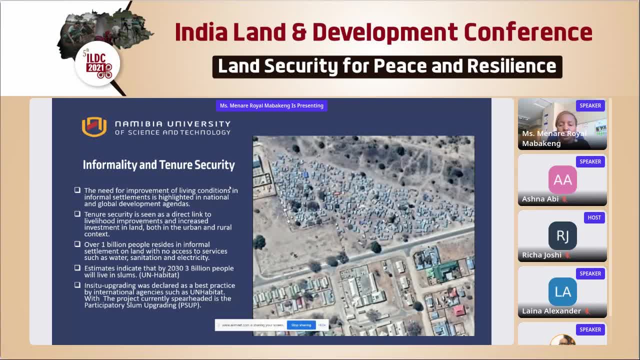 of uh. improving the, the layout, improving of uh. improving the, the layout, improving the access to services, the access to services, the access to services, but then there's not a focus on ensuring, but then there's not a focus on ensuring, but then there's not a focus on ensuring that. 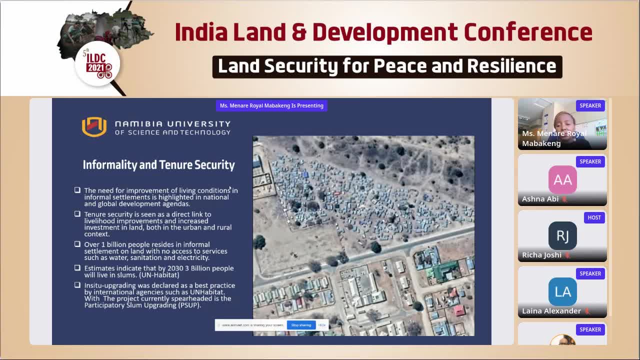 that that there is a high level of tenure security. there is a high level of tenure security. there is a high level of tenure security, and. and we have seen within research that, and. and we have seen within research that and. and we have seen within research that kenya insecurity. 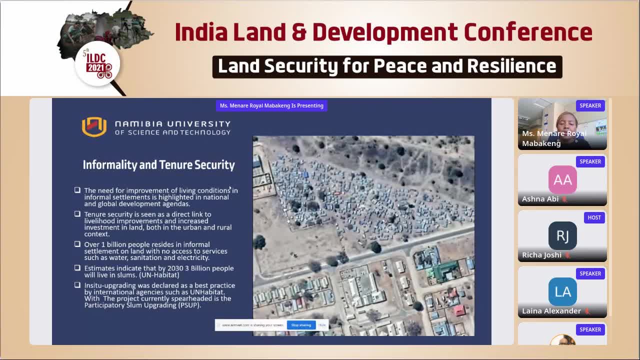 kenya insecurity. kenya insecurity does at least lessen um the people's. does at least lessen um the people's. does at least lessen um the people's participation in in development projects. participation in in development projects, participation in in development projects from our case studies that we have worked. 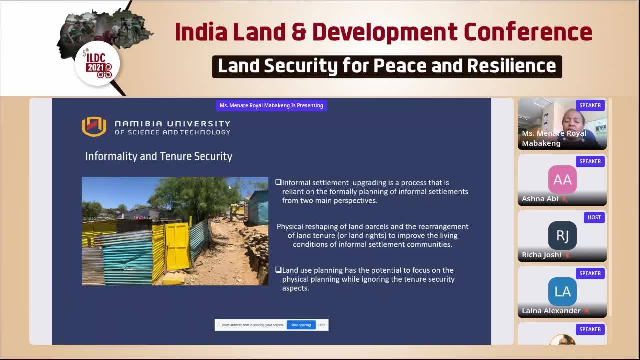 from our case studies that we have worked, from our case studies that we have worked on on on kenya, when we, when we have a proposal, kenya, when we, when we have a proposal, kenya, when we, when we have a proposal within the project to improve the level. 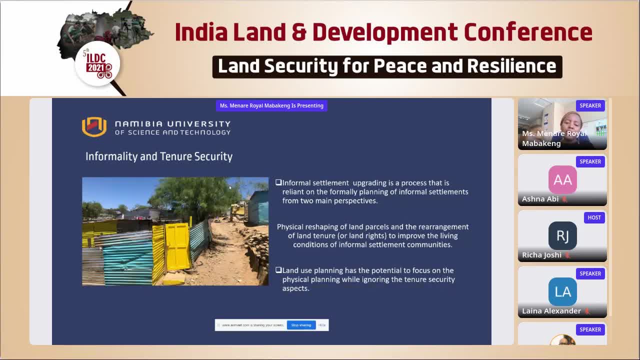 within the project to improve the level within the project to improve the level of tenure security of tenure, security of tenure, security of the community. we have a higher number of the community. we have a higher number of the community. we have a higher number of participation, of participation. 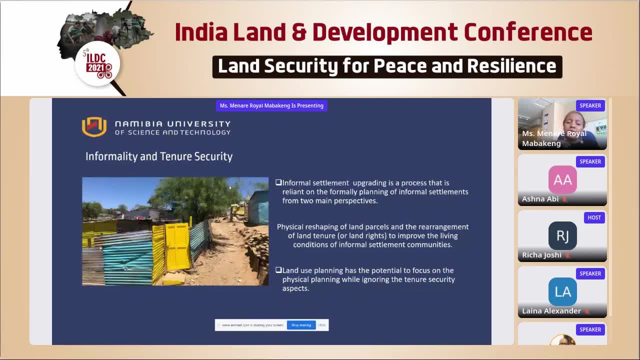 of participation, so within informal settlement upgrading, so within informal settlement upgrading, so within informal settlement upgrading what we have seen as an as an approach, what we have seen as an as an approach, what we have seen as an as an approach within the 10-9 responsive land use. 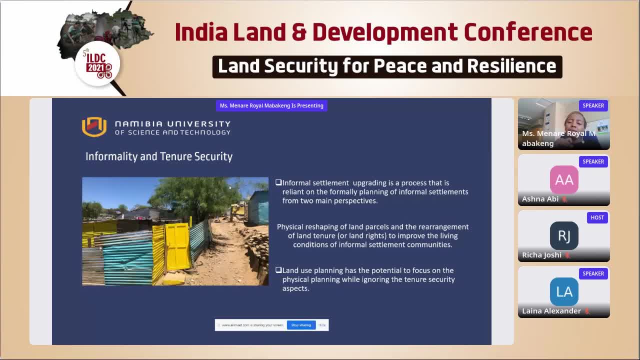 within the 10-9 responsive land use. within the 10-9 responsive land use planning process, planning process, planning process. is that it is? is that it is? is that it is- pardon me the informal settlement, pardon me the informal settlement, pardon me the informal settlement- upgrading process, that is. 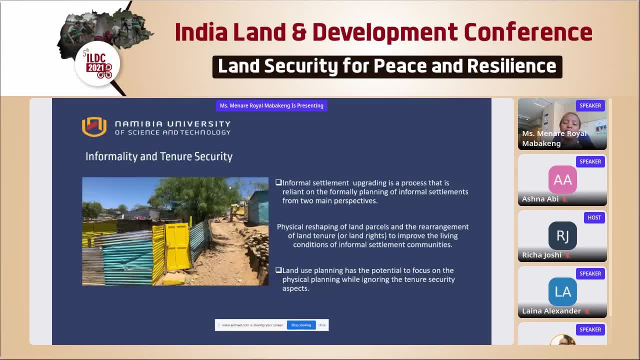 upgrading process. that is upgrading process that is uh reliant on formal uh formally planning, uh reliant on formal uh formally planning, uh reliant on formal uh formally planning of informal settlements, of informal settlements, of informal settlements. mainly focus on on these two main. mainly focus on on these two main. 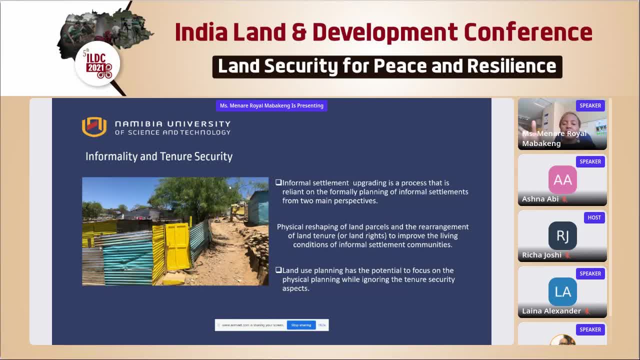 mainly focus on, on these two main perspective and i'll focus on one. which perspective? and i'll focus on one. which perspective? and i'll focus on one, which is the physical reshaping of our land. is the physical reshaping of our land, is the physical reshaping of our land parcels and the rearrangement of the 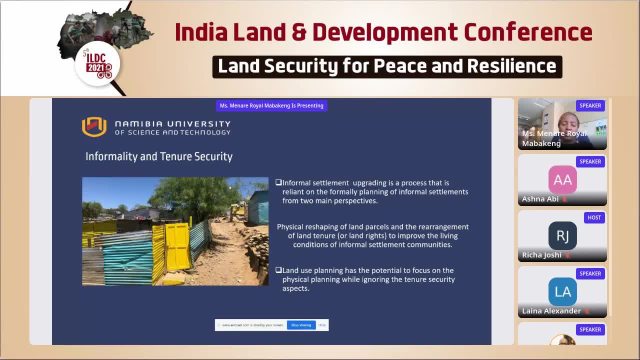 parcels and the rearrangement of the parcels and the rearrangement of the land tenure to improve the living land tenure, to improve the living land tenure, to improve the living conditions of the informal settlement conditions, of the informal settlement conditions of the informal settlement community. like i was saying, when, when. 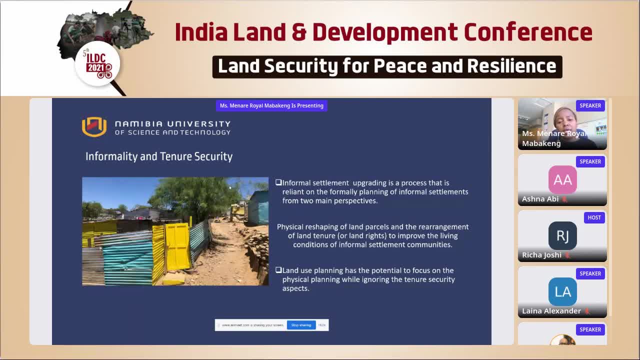 community, like i was saying when. when community, like i was saying when, when there is a clear understanding from a, there is a clear understanding from a. there is a clear understanding from a community, community, community. that they are going to um, they will, that they are going to um, they will. 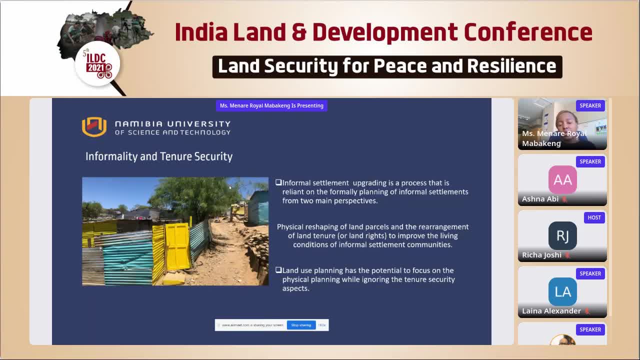 that they are going to um. they will receive, receive. receive. what we say secure land rights within the. what we say secure land rights within the. what we say secure land rights within the informal settlement upgrading process, informal settlement upgrading process, informal settlement upgrading process: there is a higher level of participation. 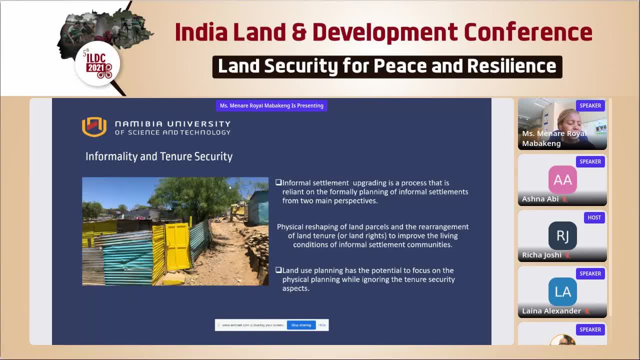 there is a higher level of participation. there is a higher level of participation um in the process of of planning, um in the process of of planning, um in the process of of planning, and we have had quite a few success. and we have had quite a few success. 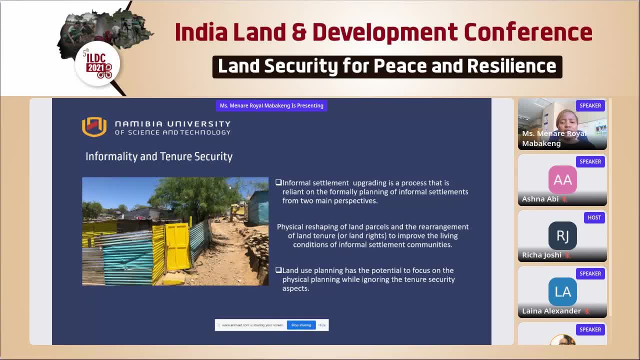 and we have had quite a few success success cases, especially for the last success cases, especially for the last success cases, especially for the last few years where communities have been few years, where communities have been few years where communities have been leading, leading, leading the upgrading projects. so land use, 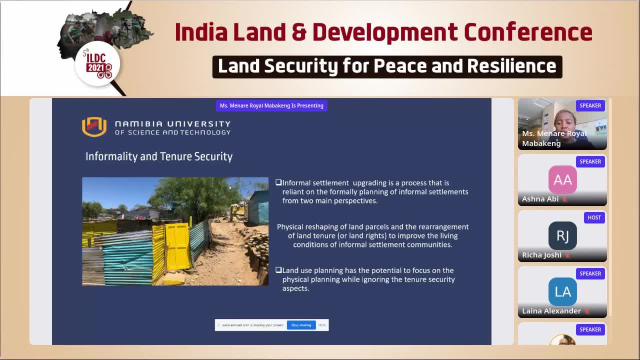 the upgrading projects, so land use, the upgrading projects, so land use planning- has the potential to focus on planning, has the potential to focus on planning, has the potential to focus on the physical planning, the physical planning, the physical planning, while ignoring the tenure aspects, and while ignoring the tenure aspects, and. 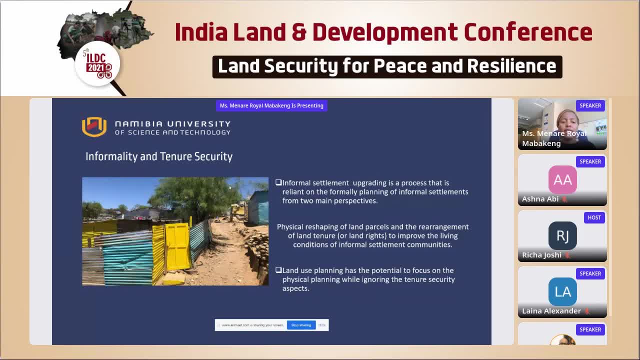 while ignoring the tenure aspects, and from the guide that has been, from the guide that has been, from the guide that has been written by professor chikwu. there are written by professor chikwu. there are written by professor chikwu. there are quite. there are different steps and 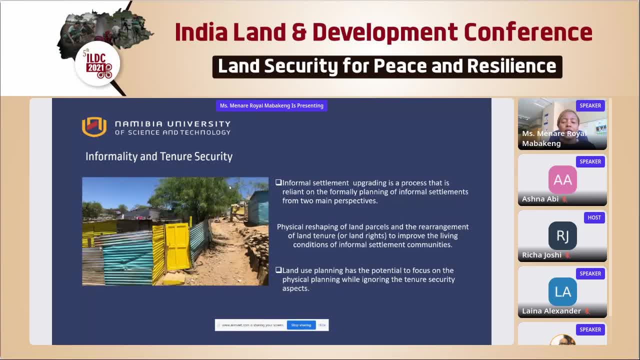 quite there are different steps and quite there are different steps and levels, levels, levels that create a clear understanding on that, create a clear understanding on that, create a clear understanding on how this can change and where how this can change and where how this can change and where planning practitioners and government 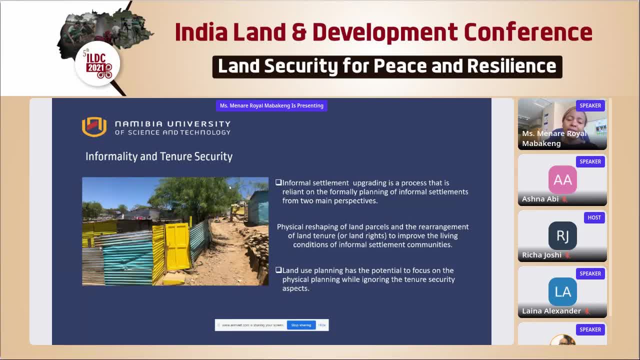 planning practitioners and government planning practitioners and government can start working together with. can start working together with. can start working together with community- not as um community, not as um community, not as um. using top-down approaches to planning. using top-down approaches to planning. using top-down approaches to planning, but focusing on this interactive. 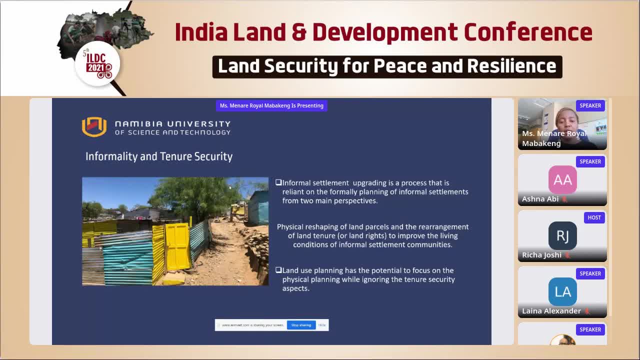 but focusing on this interactive- but focusing on this interactive partnership, partnership, partnership that can create um long-lasting uh, that can create um long-lasting uh, that can create um long-lasting uh projects and bring about projects and bring about projects and bring about, bring improvements faster to bring improvements faster to. 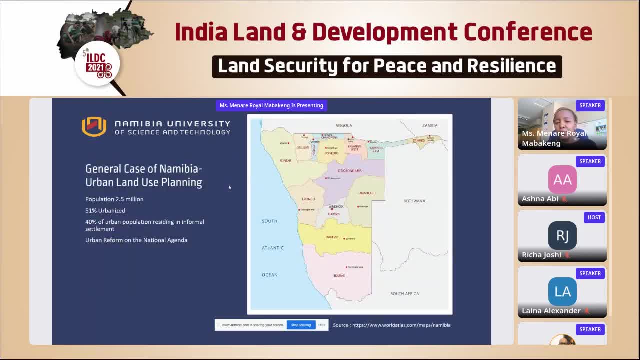 bring improvements faster to communities, communities, communities. so um for those who don't know, so um for those who don't know, so um for those who don't know. namibia, uh with namibia, uh with namibia, uh with. the last population estimates were at. the last population estimates were at. the last population estimates were at about 25, about 25, about 25, 2.5 million. i know for some they would 2.5 million. i know for some they would 2.5 million. i know for some they would say: this is just their neighborhood. 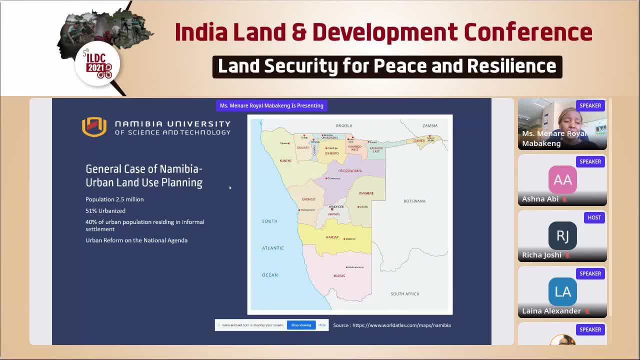 say this is just their neighborhood, say this is just their neighborhood, and what we have seen through the years and what we have seen through the years and what we have seen through the years is that namibia is, is that namibia is, is that namibia is. is going to be about 51 urbanized. 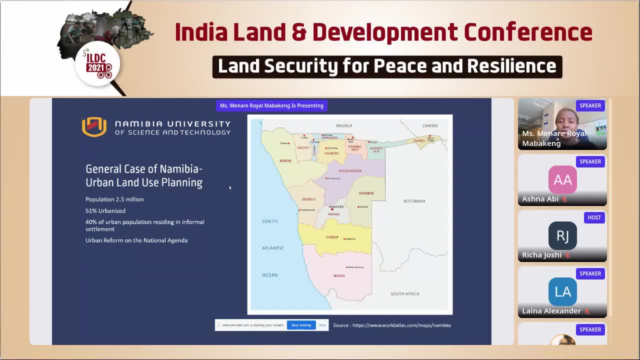 is going to be about 51 urbanized. is going to be about 51 urbanized. right so, where the for the past 20 years. right so, where the for the past 20 years. right so, where the for the past 20 years. the majority of um the, the inhabitants. 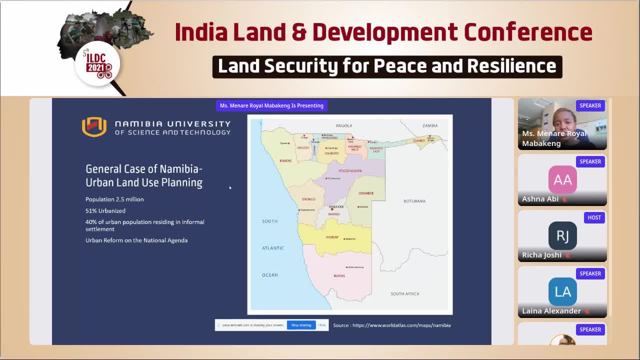 the majority of um the the inhabitants, the majority of um the the inhabitants were residing in were residing in, were residing in rural areas and we are starting to see a rural areas and we are starting to see a rural areas and we are starting to see a shift in this. 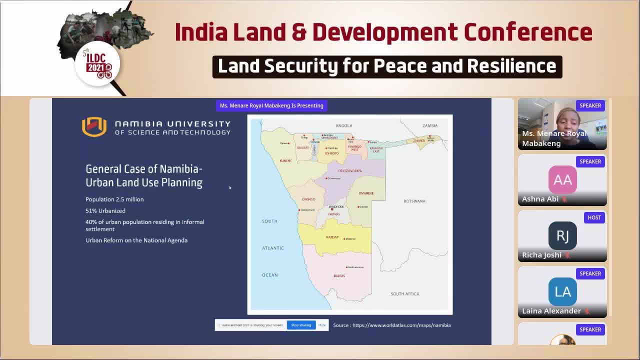 shift in this, shift in this, unfortunately, um. this, unfortunately, um. this, unfortunately, um. this is being met with the um is being met with the um is being met with the um government agenda: uh to improve urban government agenda. uh to improve urban government agenda. uh to improve urban land reform. 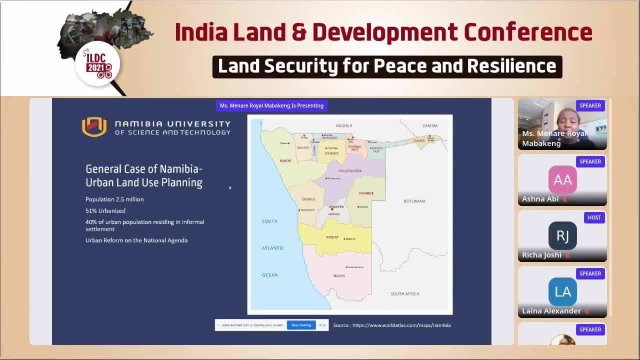 land reform, land reform, um from the 2.5 million uh population, um from the 2.5 million uh population, um from the 2.5 million uh population, we have about 40 percent of our urban. we have about 40 percent of our urban. 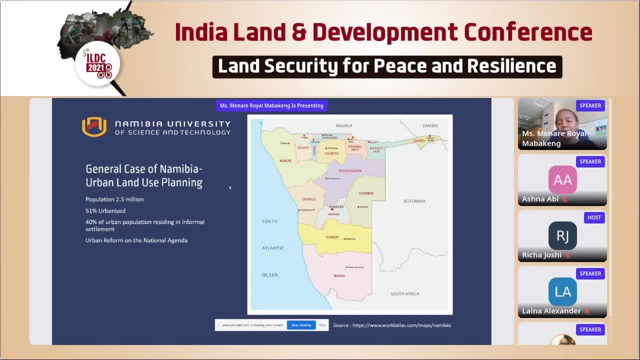 we have about 40 percent of our urban population residing in informal population, residing in informal population, residing in informal settlements, settlements, settlements. so within every namibian that is here, so within every namibian that is here, so within every namibian that is here or that is watching this conference, you 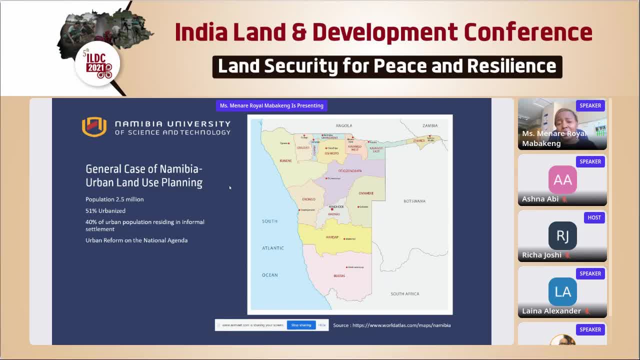 or that is watching this conference, you or that is watching this conference, you would know at least um would know at least um would know at least um, more than five people that are residing, more than five people that are residing, more than five people that are residing in informal settlements. 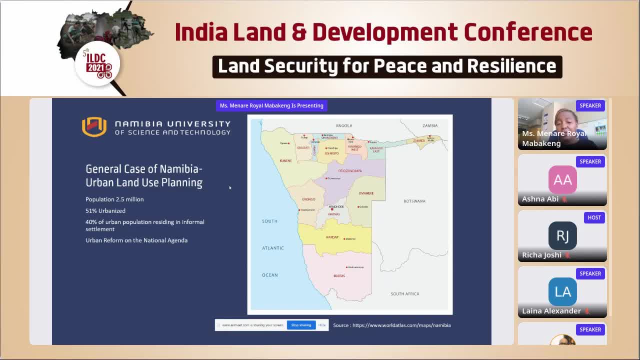 in informal settlements. in informal settlements, they don't have access to secure tenure. they don't have access to secure tenure. they don't have access to secure tenure. they don't have access to um. they don't have access to um. they don't have access to um. individual water connections or. 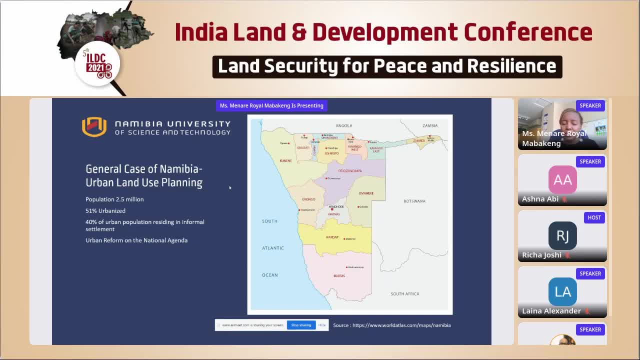 individual water connections or individual water connections or individual um toilets, within their individual um toilets, within their individual um toilets, within their communities, and this communities and this communities and this, this is quite a problem um that many of this is quite a problem um that many of this is quite a problem um that many of the inhabitants are facing. 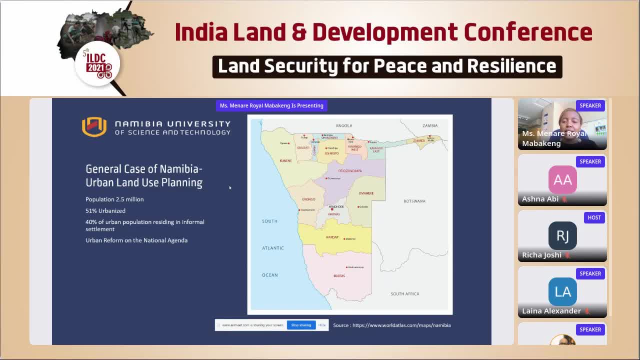 the inhabitants are facing, the inhabitants are facing within the country, but, like i said, there within the country, but, like i said, there within the country, but, like i said, there is there is, this is there is. this is there is this focus, especially from national focus, especially from national. 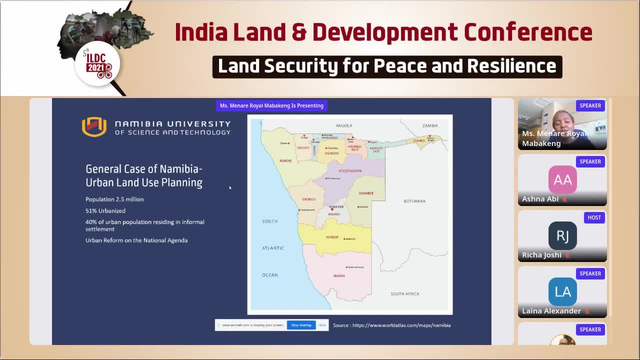 focus, especially from national government and then also in government, and then also in government, and then also in collaboration with some international collaboration, with some international collaboration with some international partners, partners, partners to move towards uh focusing on the on to move towards uh focusing on the on to move towards uh focusing on the on urban land reform. 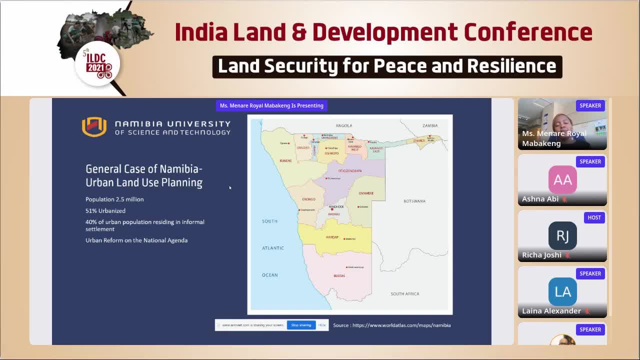 urban land reform. urban land reform: how uh local authorities can start, how uh local authorities can start, how uh local authorities can start focusing their plans on on focusing their plans on on focusing their plans on on upgrading informal settlements and having upgrading informal settlements and having upgrading informal settlements and having governments support them directly. 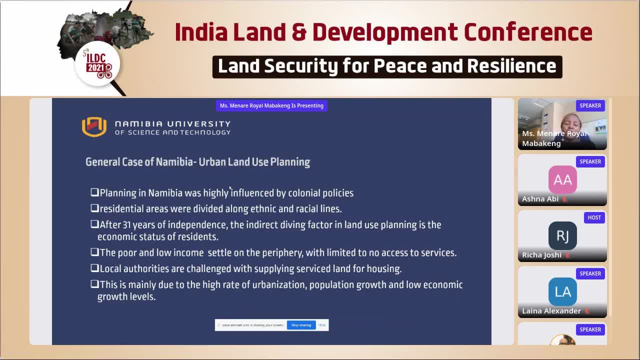 governments support them directly. governments support them directly. so further on, so further on, so further on. when we, when we look at plan in namibia, when we, when we look at plan in namibia, when we, when we look at plan in namibia, and how the and how the. 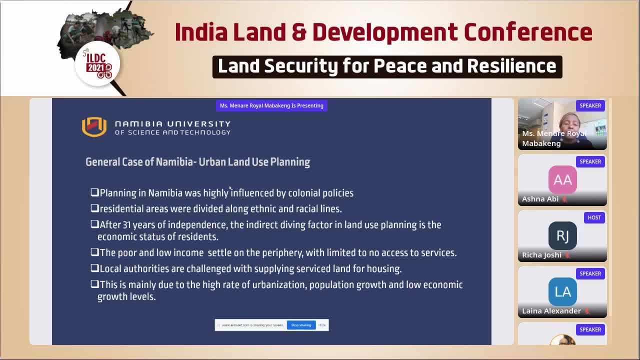 and how the the emergence of informal settlements um the emergence of informal settlements um the emergence of informal settlements um have become a challenge. is that planning have become a challenge? is that planning have become a challenge? is that planning in namibia was highly influenced by? in namibia was highly influenced by? 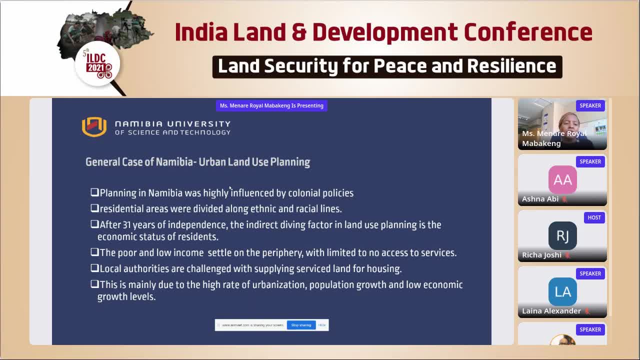 in namibia was highly influenced by colonial policies, like most countries. colonial policies, like most countries, colonial policies, like most countries. we have residential areas that were. we have residential areas that were. we have residential areas that were divided along ethnic and racial lines, divided along ethnic and racial lines. 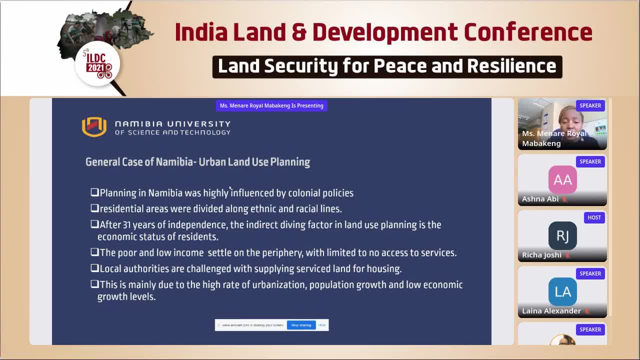 divided along ethnic and racial lines, and then after independence, after 31, and then after independence, after 31, and then after independence, after 31, years of independence, years of independence, years of independence. the indirect dividing factor that we have, the indirect dividing factor that we have, the indirect dividing factor that we have seen in land use planning, is the. 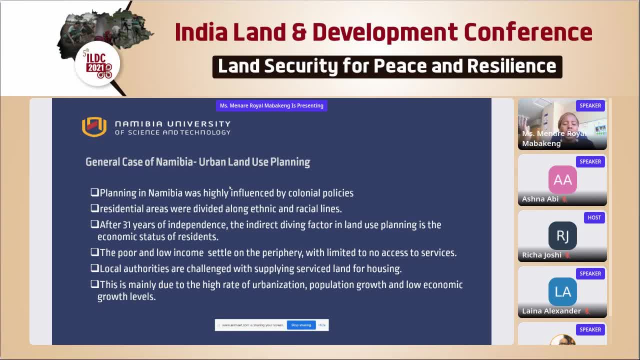 seen in land use planning is the seen in land use planning is the economic status of residence, where you economic status of residence, where you economic status of residence, where you have the poor and low income, um have the poor and low income, um have the poor and low income. um settling on the periphery with limited to. 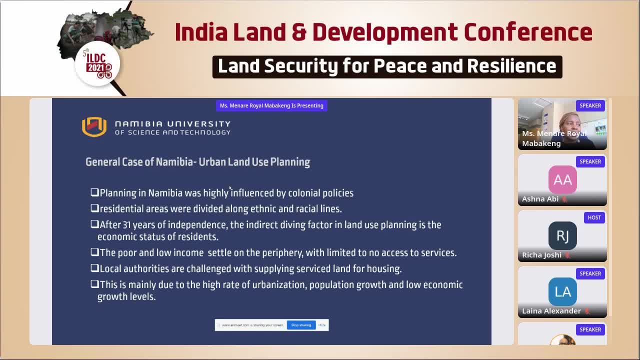 settling on the periphery, with limited to settling on the periphery with limited to no access to services, no access to services, no access to services. and then you have these challenges that, and then you have these challenges that, and then you have these challenges that local authorities are faced with. 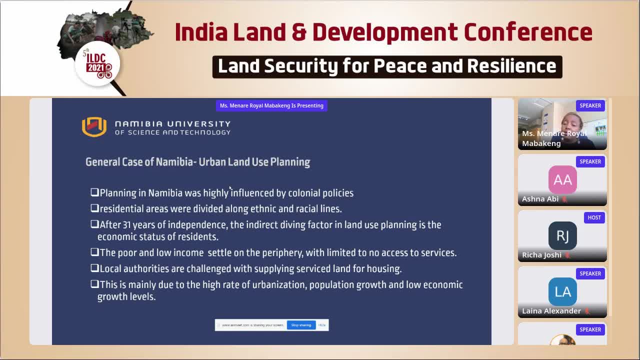 local authorities are faced with. local authorities are faced with with supplying service land: uh at the low. with supplying service land, uh at the low. with supplying service land, uh at the low cost, cost cost and then also at a high speed, uh to meet, and then also at a high speed, uh to meet. 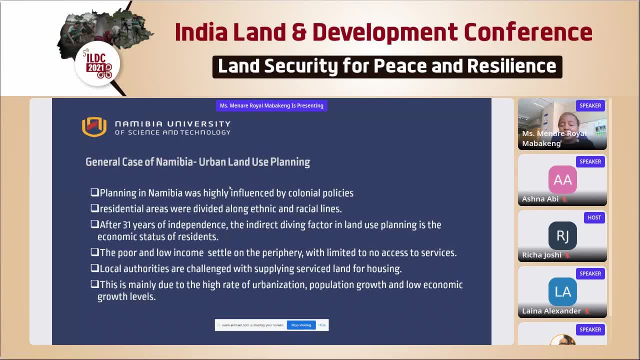 and then also at a high speed, uh, to meet the current demands, the current demands, the current demands, and, and this, this is, this is a challenge, and and this, this is, this is a challenge, and and this, this is this is a challenge. that i, that i, that i, we have observed local authorities, um, 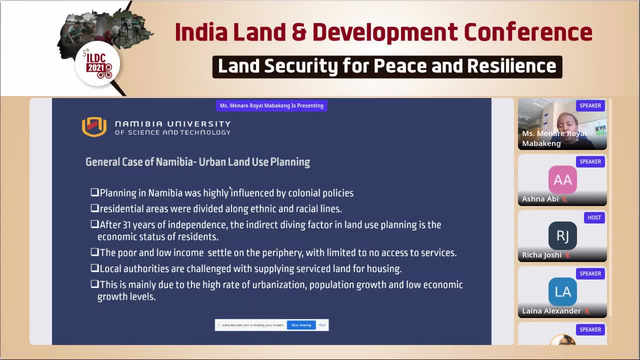 we have observed local authorities, um, we have observed local authorities um are taking on and and willing to look, are taking on and and willing to look, are taking on and and willing to look forward to forward, to forward to um collaborative solutions, uh with. um collaborative solutions, uh, with. 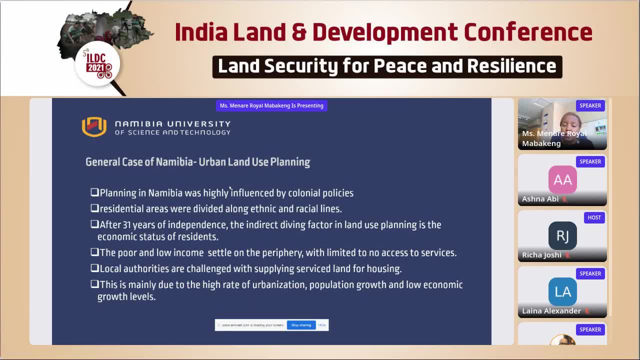 um collaborative solutions uh with the, the university, and then also with the, the university, and then also with the, the university, and then also with um the public and private sector. uh one um the public and private sector. uh one um the public and private sector. uh one of. 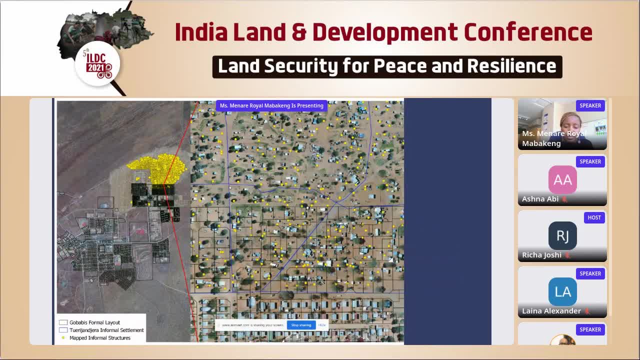 of of the leading uh projects that we have had, the leading uh projects that we have had, the leading uh projects that we have had and that i said and that i said and that i said is um. one of our leading examples is of is um. one of our leading examples is of. 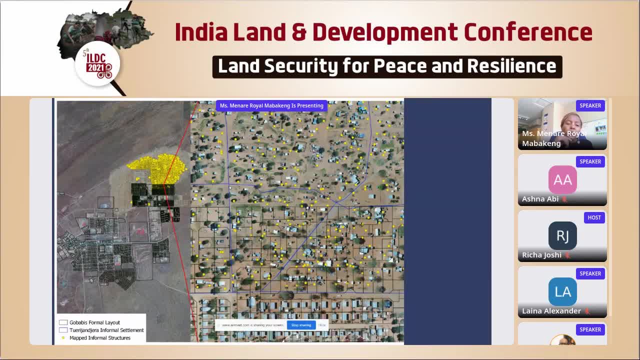 is um. one of our leading examples is of this uh informal settlement. this uh informal settlement, this uh informal settlement we've seen. we've seen. um hubab is one we've seen. we've seen. um hubab is one we've seen. we've seen. um hubab is one of the 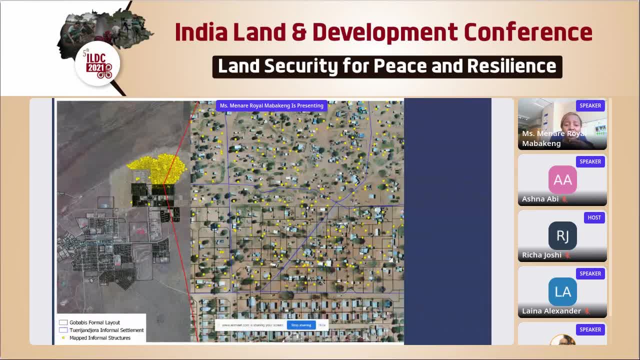 of the, of the, the one of the the regional capitals in the one of the the regional capitals in the one of the the regional capitals in in namibia, in, in namibia, in, in namibia, in, in the mahaka region. what we see here in in the mahaka region, what we see here. 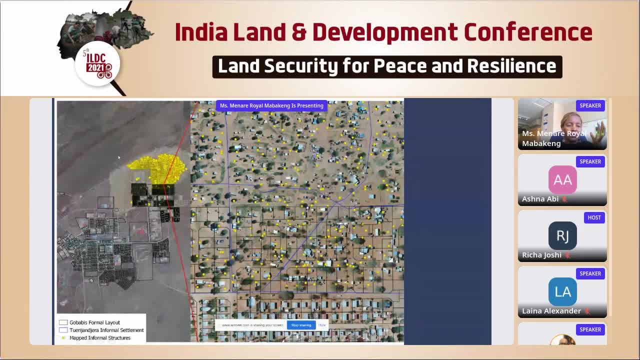 in in the mahaka region. what we see here, this is this is: this is um simple diagram or layout of an entire, um simple diagram or layout of an entire, um simple diagram or layout of an entire town, town, town. so what we see? the majority of the 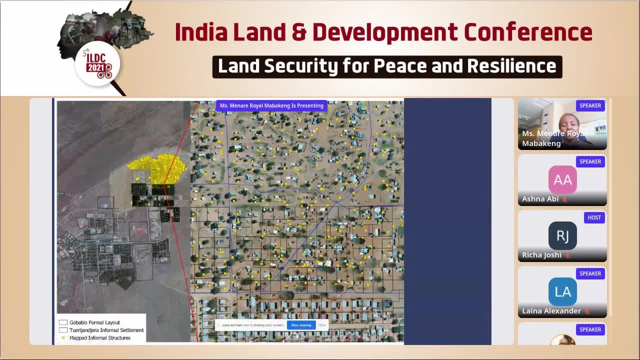 so what we see? the majority of the. so what we see: the majority of the inhabitants within the town are residing inhabitants within the town are residing inhabitants within the town are residing in informal settlements, in informal settlements, in informal settlements. so every time there is a proposal or at 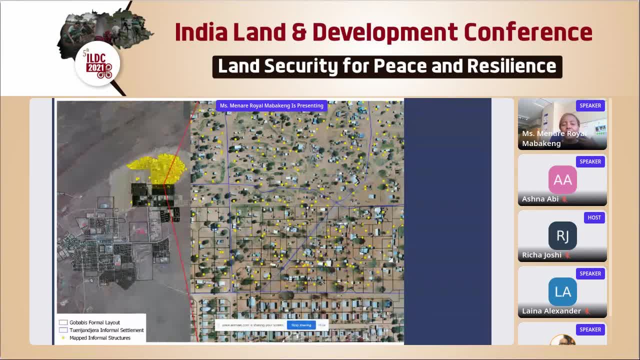 so every time there is a proposal, or at so every time there is a proposal or at least a discussion, least a discussion, least a discussion- to upgrade the area, you will see that. to upgrade the area, you will see that. to upgrade the area, you will see that there would be. 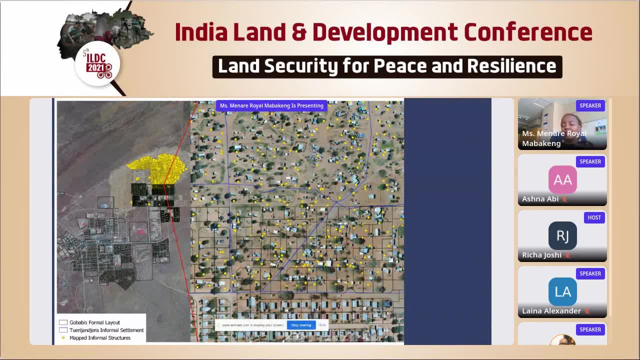 there would be. there would be an increase in the number of inhabitants, an increase in the number of inhabitants, an increase in the number of inhabitants overnight, overnight, overnight. and we see that the the solution to, and we see that the the solution to and we see that the the solution to managing the growth of informal. 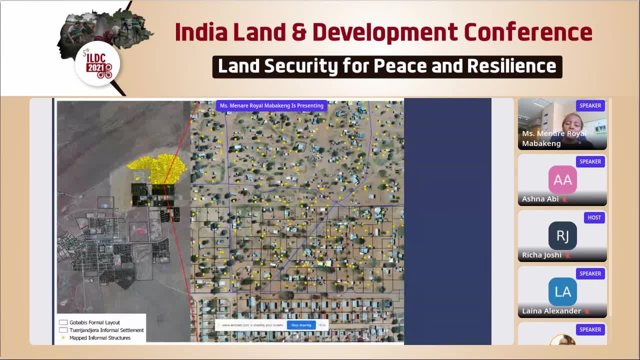 managing the growth of informal, managing the growth of informal settlements, settlements, settlements, and then also ensuring that our upgrading and then also ensuring that our upgrading and then also ensuring that our upgrading projects are sustainable and can bring projects are sustainable and can bring projects are sustainable and can bring about effective. 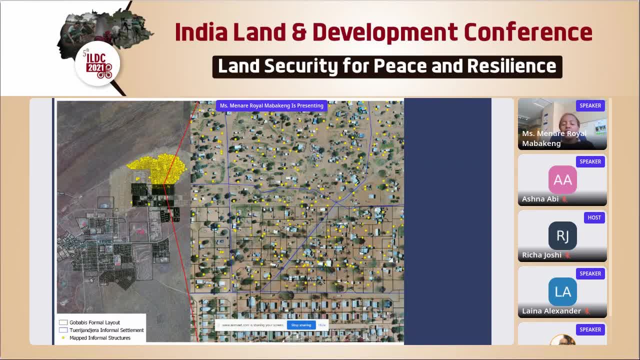 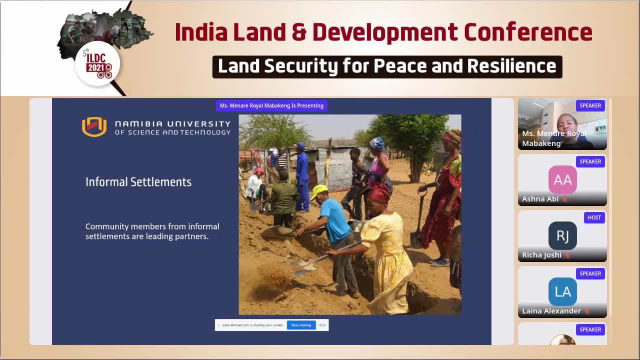 about effective, about effective- at least tangible results for communities, at least tangible results for communities, at least tangible results for communities- is to work on this, is to work on this, is to work on this collaborative partnership, seeing collaborative partnership, seeing collaborative partnership, seeing communities, communities, communities not as as beneficiaries of upgrading. 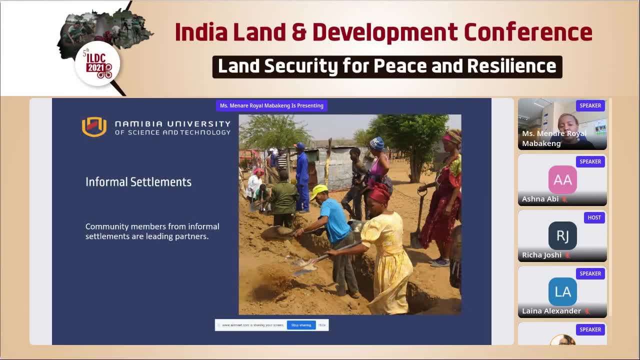 not as as beneficiaries of upgrading, not as as beneficiaries of upgrading projects, projects, projects, but as contributors uh to upgrading so, but as contributors uh to upgrading so, but as contributors uh to upgrading so, the project that we have worked on, the project that we have worked on, the project that we have worked on in in collaboration with the sheikh, 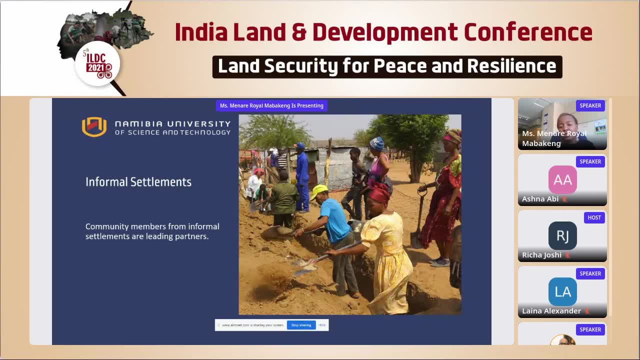 in in collaboration with the sheikh in in collaboration with the sheikh dwellers federation of namibia. dwellers federation of namibia. dwellers federation of namibia, which is also affiliated to slum dwellers, which is also affiliated to slum dwellers, which is also affiliated to slum dwellers international. 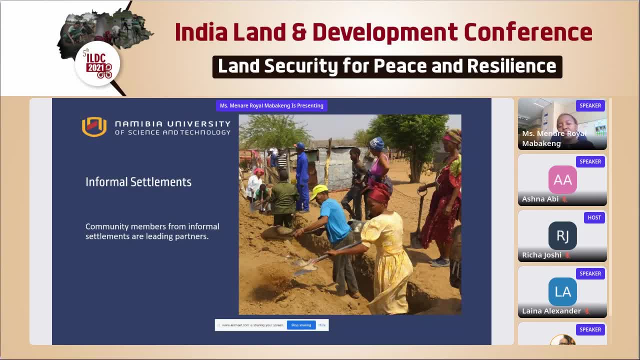 international. international is the one where the focus is on building, is the one where the focus is on building, is the one where the focus is on building capacity of informal settlement capacity of informal settlement capacity of informal settlement residence residence, residence around settlement design around settlement, design around settlement design, and then also the installation of 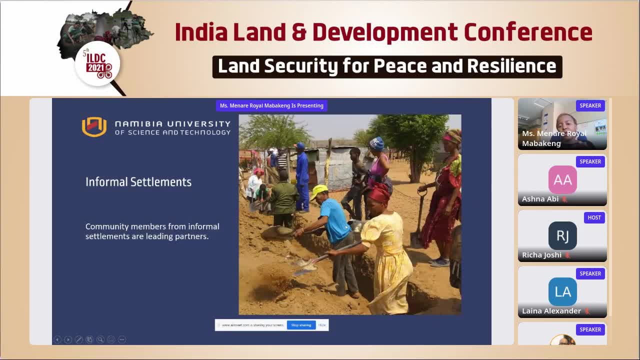 and then also the installation of and then also the installation of infrastructure. so what you see here is a infrastructure. so what you see here is a infrastructure. so what you see here is a group of group of group of community members that contributed or at community members that contributed or at. 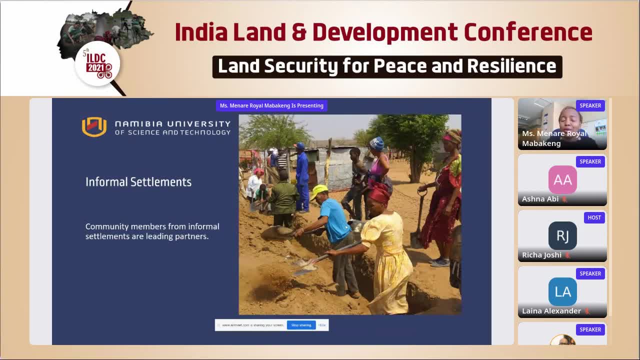 community members that contributed, or at least, least least that we're working on the project um. to that we're working on the project um. to that we're working on the project um to install: install. install uh sewer and water reticulation within an: uh sewer and water reticulation within an. 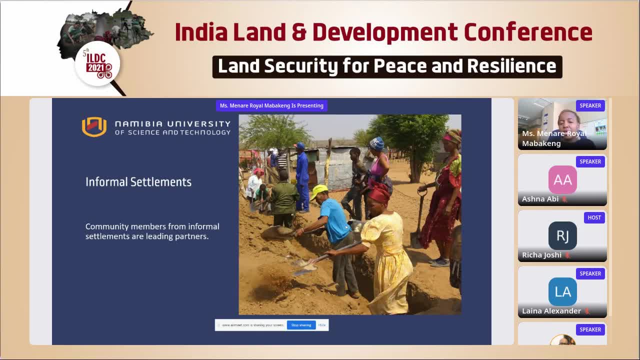 uh sewer and water reticulation within an informal settlement, informal settlement, informal settlement within this process is well received within this process, is well received within this process, is well received, especially like i would emphasize i, especially like i would emphasize, i, especially like i would emphasize, i think, throughout this discussion. 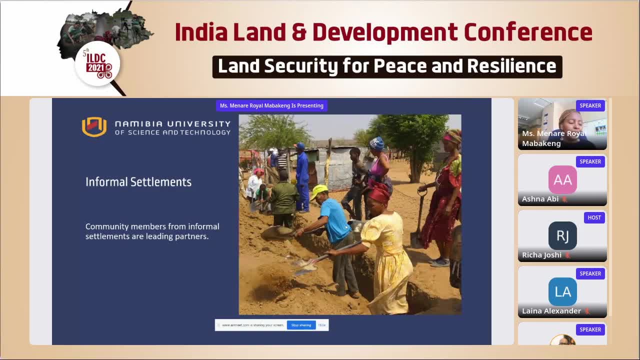 think throughout this discussion, think throughout this discussion, when community members are seen as, when community members are seen as when community members are seen as partners, partners, partners, not as beneficiaries, and in this case i not as beneficiaries and in this case i not as beneficiaries, and in this case i would emphasize: 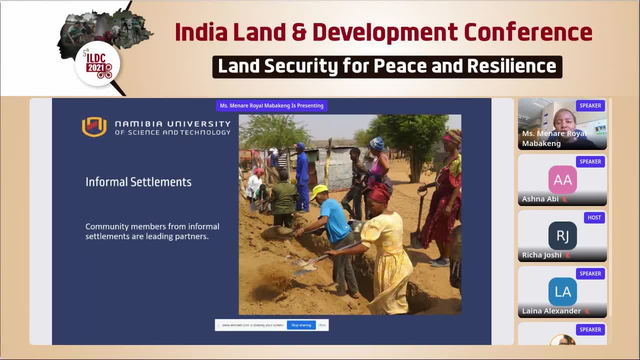 would emphasize. would emphasize that when, when we speak about community, that when, when we speak about community, members from informal settlement being members from informal settlement, being members from informal settlement being seen as partners, seen as partners, seen as partners is is to say, when you are designing your. 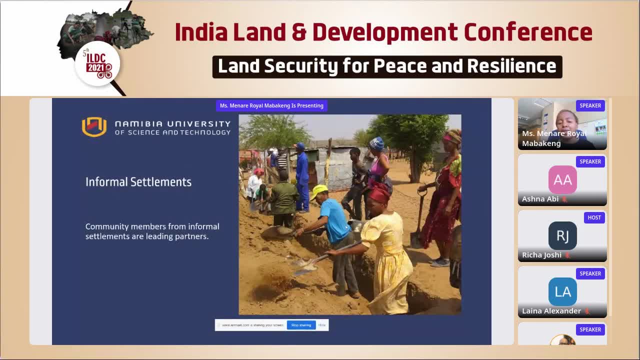 is, is to say when you are designing your, is is to say when you are designing your project for for informal settlement project, for for informal settlement project, for for informal settlement, upgrading, or you are planning upgrading, or you are planning upgrading or you are planning your area. you don't only consult them. 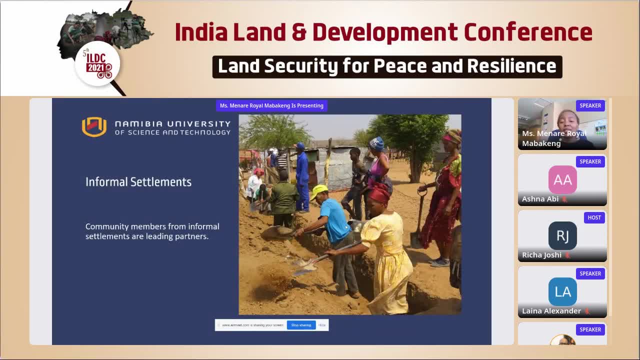 your area. you don't only consult them. your area. you don't only consult them when you have the idea or when the when you have the idea or when the when you have the idea or when the picture is clear on what you want to, picture is clear on what you want to. 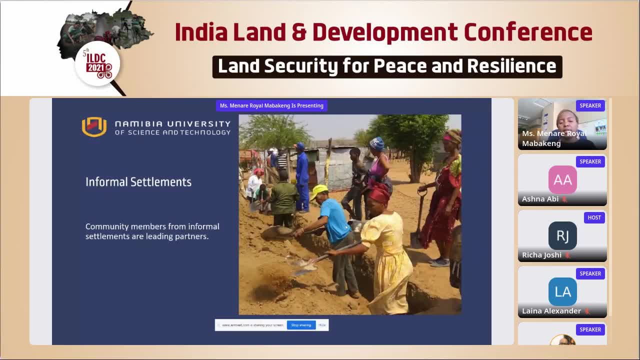 picture is clear on what you want to implement, implement, implement. you start consulting them from the, you start consulting them from the. you start consulting them from the beginning within your project design, beginning within your project design, beginning within your project design, and, and we see that as this being um- 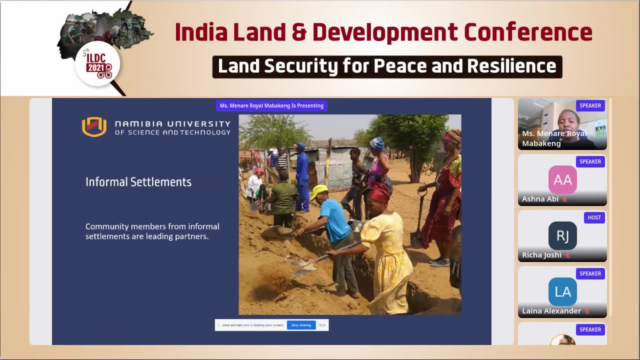 and- and we see that as this being um, and, and we see that as this being um- a proper way of of not only ensuring a proper way of, of not only ensuring a proper way of of not only ensuring that the projects get implemented in, that the projects get implemented in. 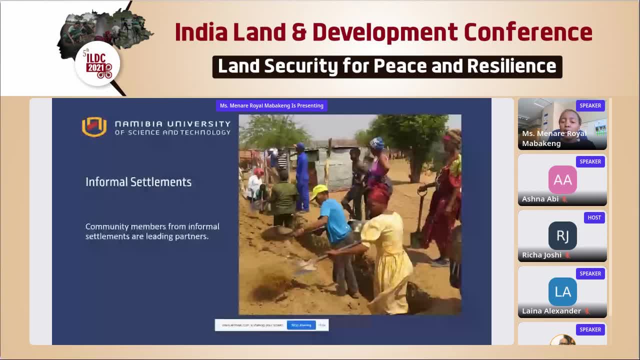 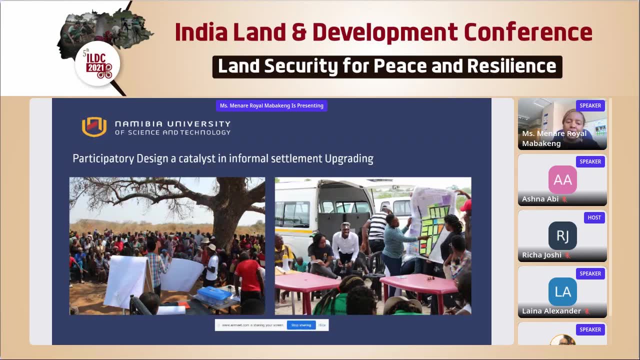 that the projects get implemented in time, but then there is also a higher time. but then there is also a higher time, but then there is also a higher increase in owning the project outputs. increase in owning the project outputs, increase in owning the project outputs, so so, so, within the, the, the participatory design, 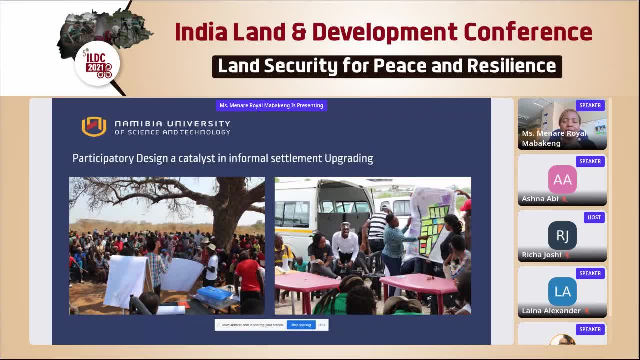 within the, the, the participatory design. within the, the- the participatory design, what we see as, as, as, as as a catalyst, in what we see as, as as, as, as a catalyst, in what we see as, as, as, as a catalyst in the upgrading of informal settlements. 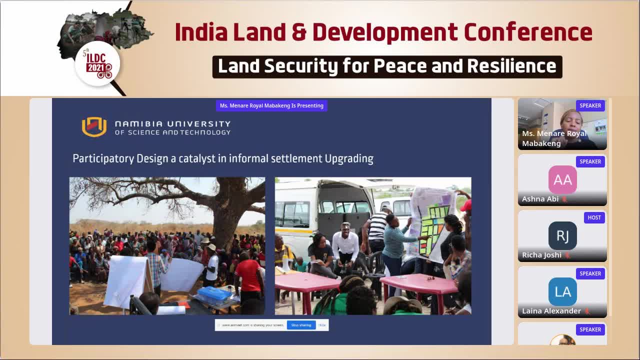 the upgrading of informal settlements, the upgrading of informal settlements, that it also gets to reduce the. that it also gets to reduce the. that it also gets to reduce the- what we call the misinformation that, what we call the misinformation that, what we call the misinformation, that sometimes community members um 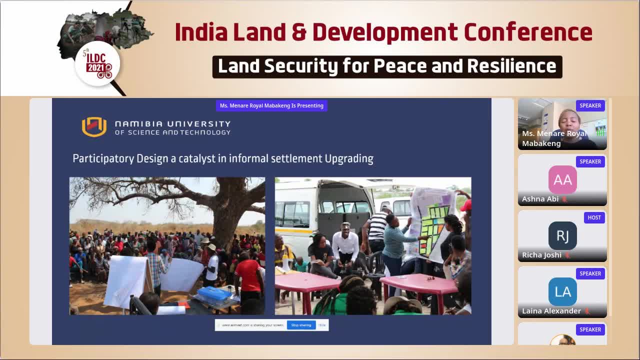 sometimes community members, um, sometimes community members, um are victims of, if i should say because, are victims of, if i should say because are victims of, if i should say because when, when you have upgrading projects, when, when you have upgrading projects, when, when you have upgrading projects, do you have this emergence of um. 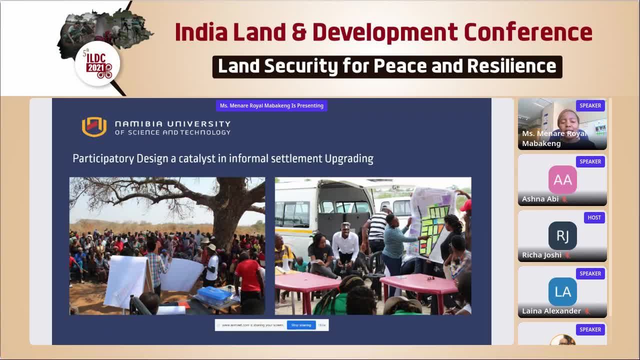 do you have this emergence of um? do you have this emergence of um, ideas that can also be influenced by ideas that can also be influenced by ideas that can also be influenced by either the political discussions within, either the political discussions within, either the political discussions within an area. 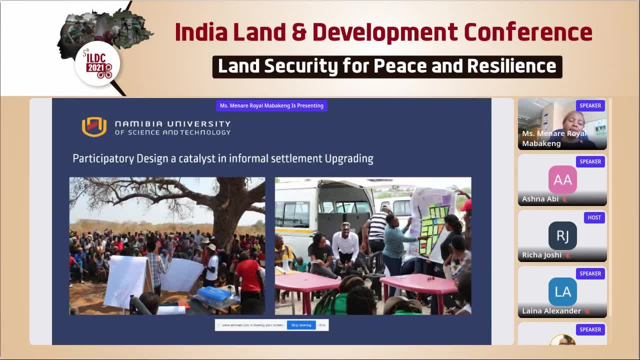 an area or some of the um, some at some agendas of um, of elite people within within a community. so participatory design allows community members to come to the table and provide their views and also ask questions on how they can contribute and then also how they're going to benefit from. 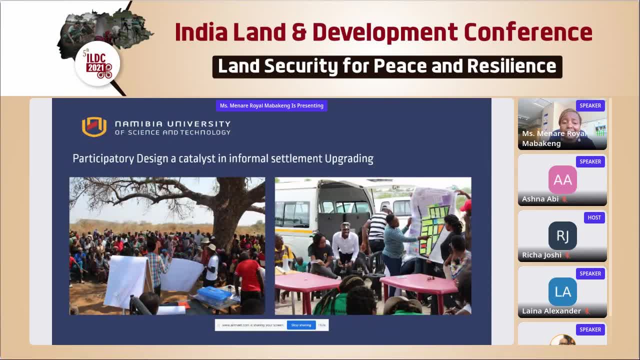 the from the project. what this also does is it brings, it brings about um a reduction in, in mistrust. uh, because what we see mostly when, when you bring, or at least when there are proposals for, for upgrading or any projects, there's always a suspicion about who will benefit and who will. 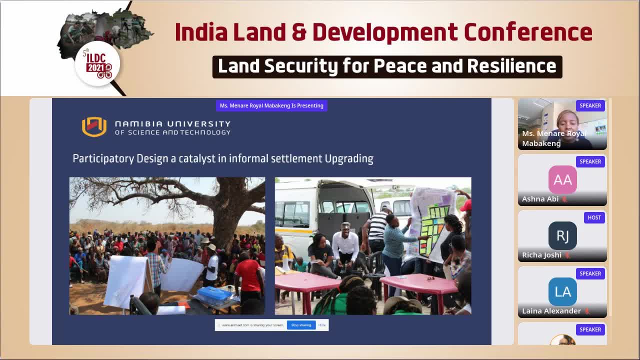 be excluded. so when you have a participatory design process within your planning, it allows this interactive discussion and then everybody within the project is seen as equal. you don't see in the design process everybody is being seen as equal and um, at least in the design process. 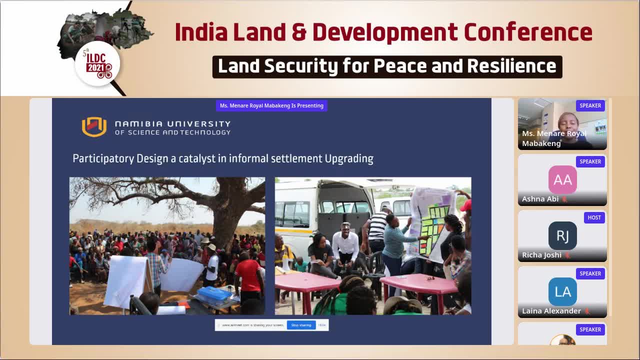 so you're not either a result of the existing design process, which maybe were created by the NGO, or from the university as solution providers, community members now also start seeing themselves as as what we call um designers of their own space, and also see themselves as as as contributors to the final project. 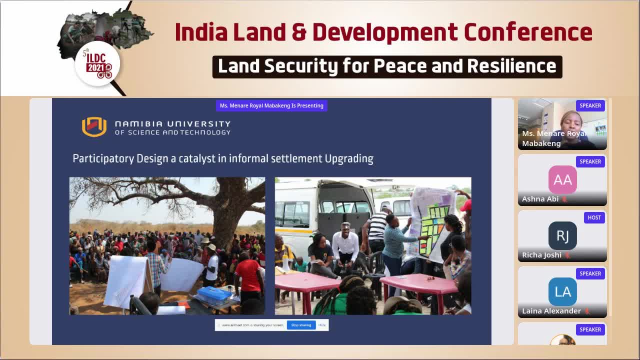 What we see is that when you constantly have projects that can be delayed, sometimes by funding, and you don't have a participatory process in place, it gets to reduce, let's say, the number of community members that will come to meetings and then also community members that are willing to participate. 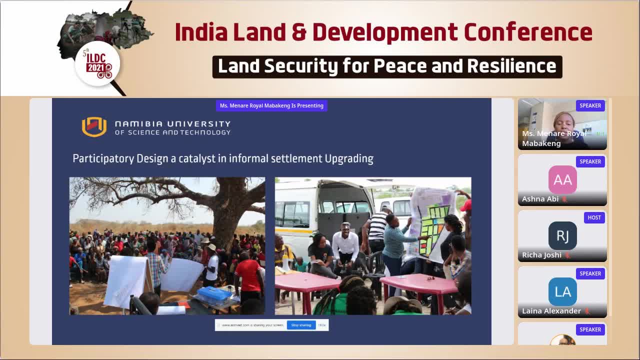 Because we have seen across the years that there has been proposals to improve informal settlements, but then the improvements sometimes end up at the installation of water points or communal toilets And then when you come again as a team to propose or at least initiate an upgrading project, there gets to be a reduced interest because sometimes not all projects deliver according to the way. 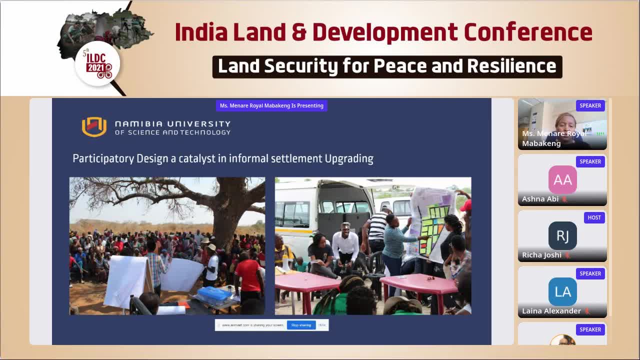 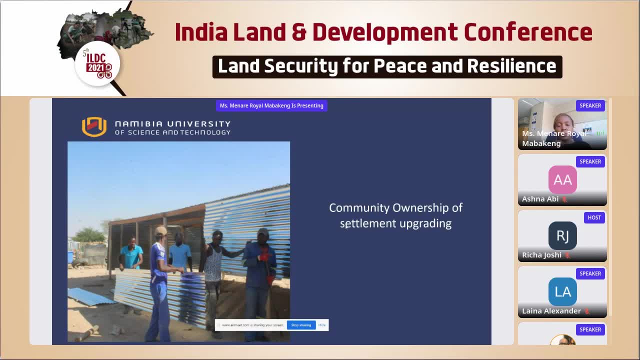 They, at least the objectives, were presented to the community. So participatory design helps reduce what we call development fatigue. And then, when communities own the or at least are part of the informal settlement upgrading process, it also reduces this resistance that we sometimes do experience or do get during upgrading projects where there will be a refusal, for example, for households to 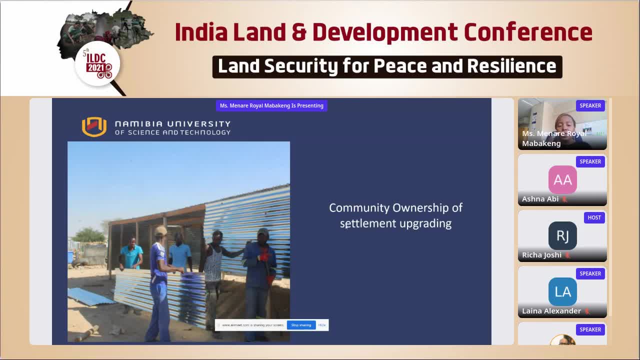 Esto obstacles lo libres que refrigeratoran los demuelle? for what reason break down their structures? i would put a note here that I think the I would put a note here that I think the I think the advantage that we have. 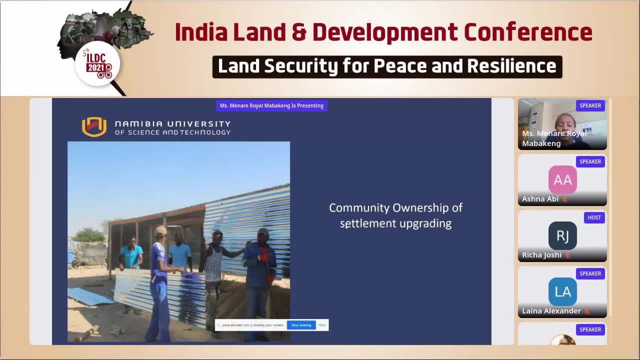 advantage that we have with informal settlements, with informal settlements in Namibia, 表示 compared to other countries. compared to other countries is that is, that majority of are가, the, They are structures informa. structures belong to corrugated iron são, which This also again because is. 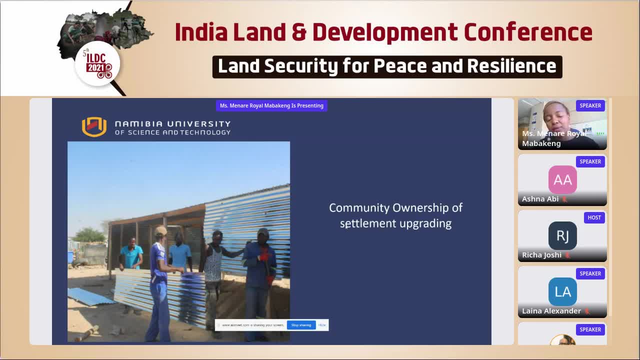 is. it's also And built it's than re-built. Therefore, that that 혹, that we take Dewa more like that. This also affects community members in the sense that they invest quite a lot in maintaining their structures. So there will be resistance when an upgrading or a planning process, an upgrading that results. 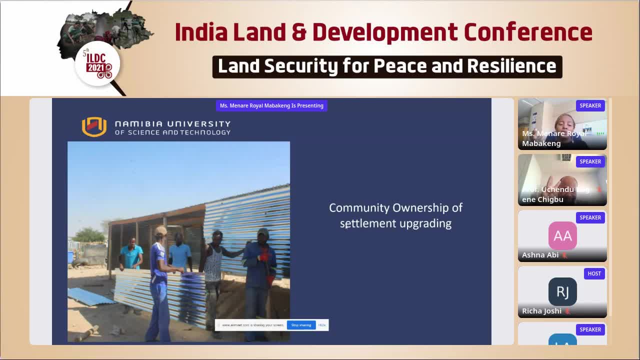 from a planning process that did not include the community comes to a settlement, They will see that they are going to lose a certain level of investments in their structures. But when you have this participatory design process, whatever layout is finalized based on the inputs of the community, you end up having this increased buy-in, even where individuals 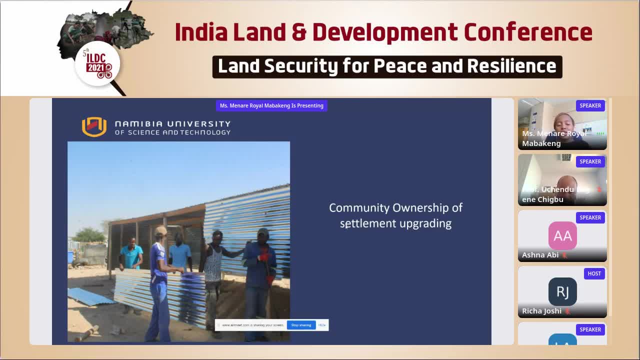 in the community will voluntarily dismantle their structures, and then local authorities do come in and provide additional materials or transport. So what we emphasize within the at least 10-year responsive land use planning, from my own interpretation, is this promotion of having communities being partners within the implementation. 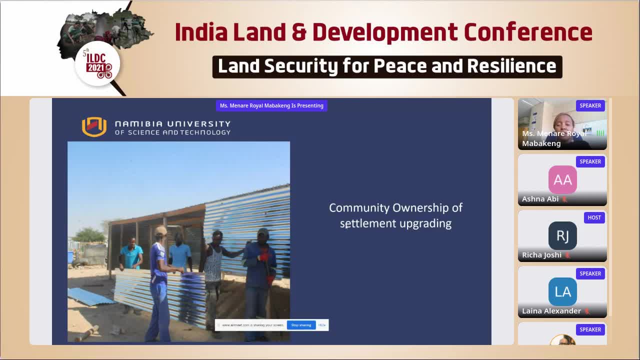 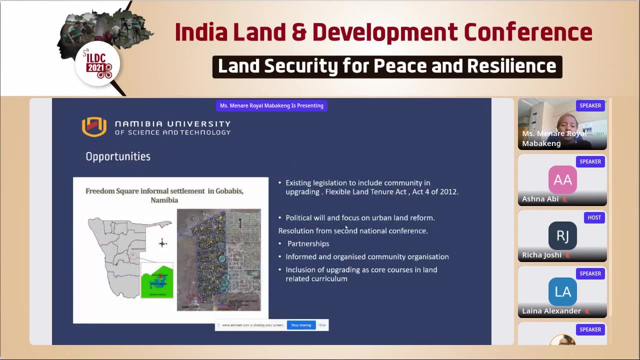 of the design and also the implementation of land use plans, Because this ensures that projects are not only sustainable, But then also sustainable, So that there is a high, increased ownership of the upgrading. So what are the opportunities? Like I mentioned earlier on in the presentation for Namibia, what we have seen is that there 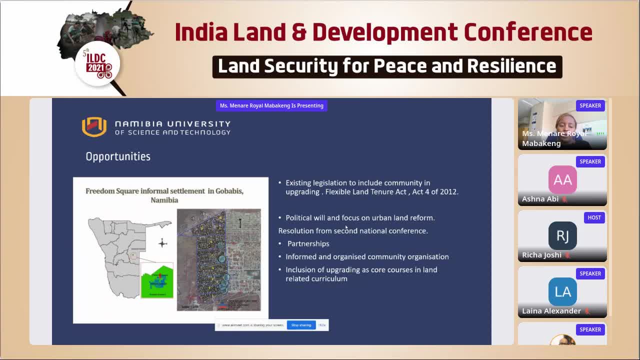 is a focus right now on urban land reform. government investments for the past few years, in terms of finance and then also in terms of projects, have been on rural areas, where the promotion of land use plans have been in place, And then the promotion of communal land registration has been key on the agenda. 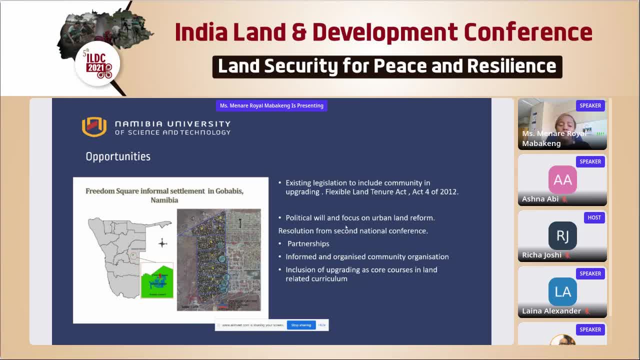 And then also the land reform program that focused on resettlement of previously disadvantaged Namibians on farms where there is a promotion on agricultural activities. So that has been a focus of government and it still is a priority. But what we have seen, especially from the second national land conference, is this promotion. of land use plans And I think it's a very important thing, And I think it's a very important thing, And I think it's a very important thing. But what we have seen, especially from the second national land conference, is this promotion. 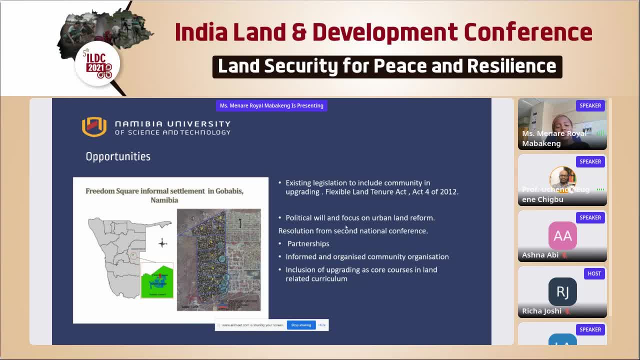 of urban land reform, where there is an ongoing discussion around the proposal of new policies that are going to support the improvement of living conditions and informal settlements. Local authorities are looking at having clear structure or at least upgrading policies within their councils, And then there is also an increase inettitude. 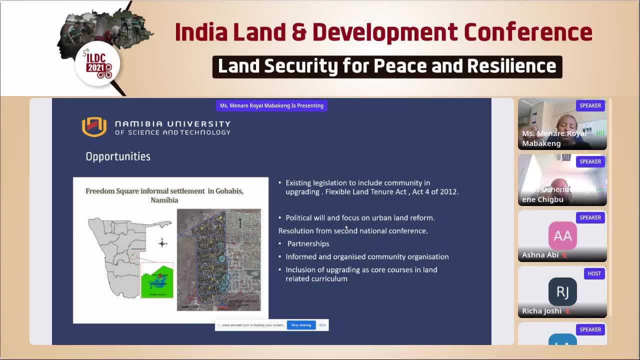 support from private sector in the construction of housing for communities that are redesigned and replanted. What we see here is- this is one of our- I would say- pilot sites and also success cases from the part of having a community of about 1,000 households. How many hectares was this? 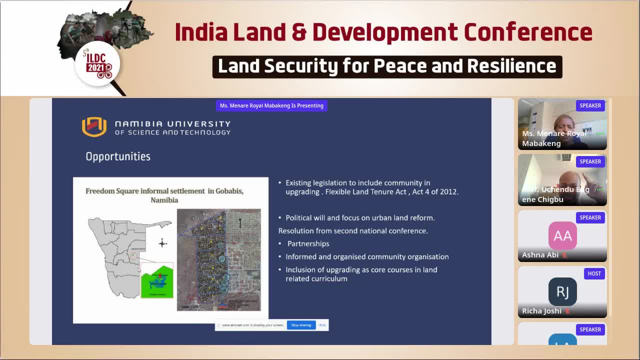 I think about, if I say I don't know if it was 60 to 50 hectares, having to have a whole settlement redesigned and each individual household having to receive a title to their land. So what we see as opportunities, yes, is the existing legislation that 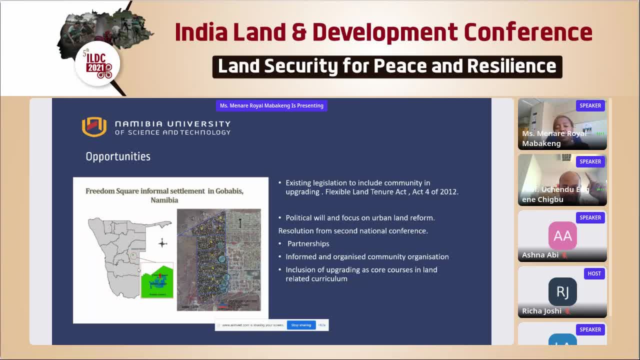 promotes the inclusion of community in upgrading And for Namibia, at least as a test case, we have the flexible land tenure act for 2012,. although the discussions right now are that, how many minutes? I'm rounding up? You were already done five minutes ago. 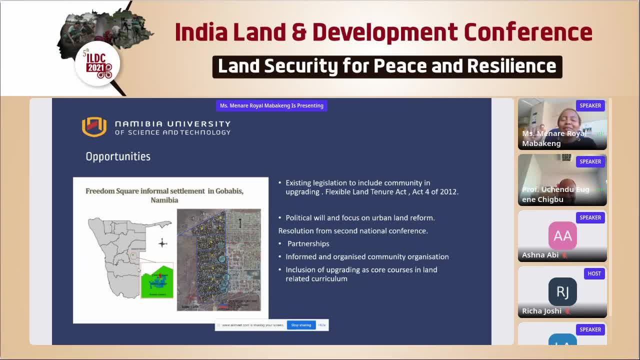 Sorry, Sorry, Sorry. Okay, I'm rounding up. Okay, what we have seen is that there's this existing legislation of the flexible land tenure Act four of 2012 that promotes the flexible land rights that local authorities, in collaboration with national government, can issue to communities. So you start from a standard. 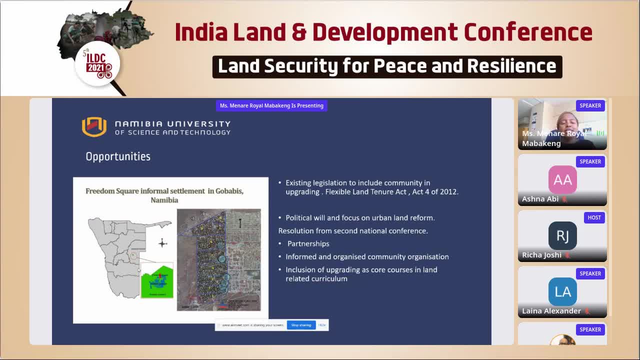 title for a block of land that has not, that is not planned, and then you move to a landhold title when the community has planned the area and what is registered is the entire block instead of the individual subdivisions that are measured with the use of a technical land. 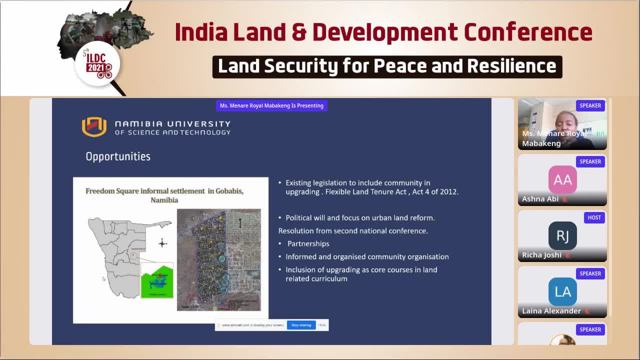 surveyor rather than a professional land surveyor, and this reduced costs, at least from our observations. What we see is that there is also political will, and I emphasized this previously, that there's a focus on urban land reform, there's an increase in partnerships and the Namibia. 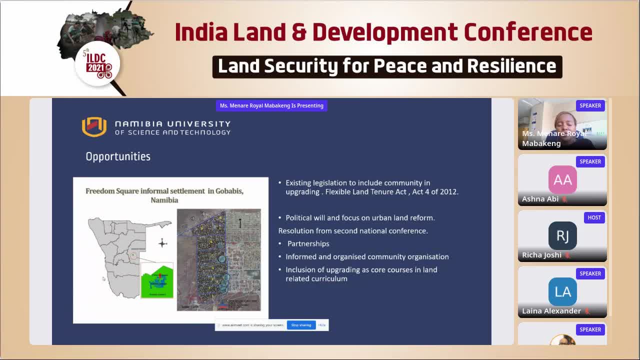 University of Science and Technology is quite at the center of that, where we are promoting informal settlement upgrading within our curriculum, where we are also promoting the design studios, with students from town planning and architecture interacting with the communities directly, and there is also this informed and organized community organization from the community-based 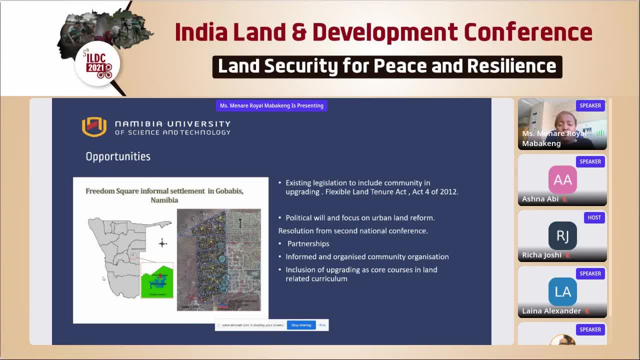 organization And also from individuals in the informal settlements themselves. So inclusion of upgrading has become a core of courses within our curriculum, like I mentioned, not only within the department of land and property sciences, but within the faculty of natural resources in general. So, ladies and gentlemen, that's all that I had to share with you. 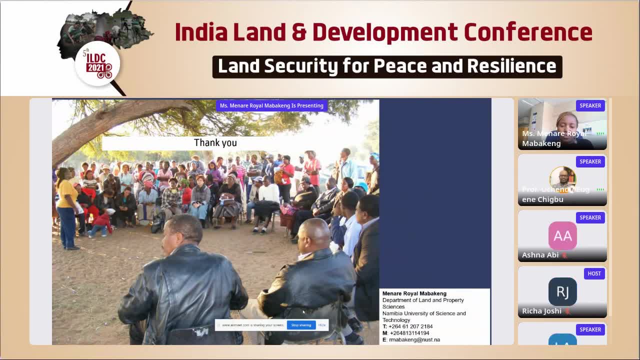 today. Thank you so much for your attention and yes, we are welcoming questions and I know now, if all these questions are answered, we will be able to answer them in the next few minutes. If all is sorted, Professor Chiku will go a bit more into Kenya: responsive land use planning. Thank you, 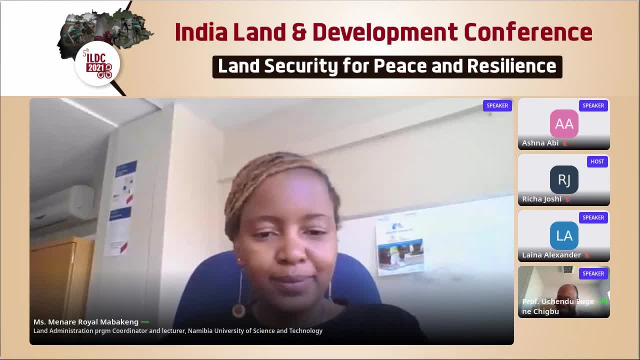 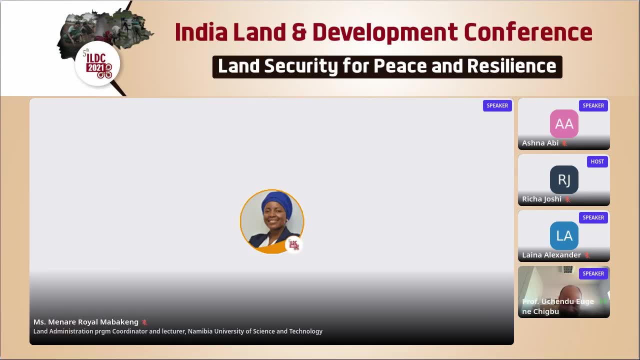 Okay, thank you, Royo, and thank you everyone for listening. That was quite an interesting presentation and also she just saved me from the embarrassment of not being able to, you know, load my presentation. But the plan was for us to go from general to specific, but now it appears. 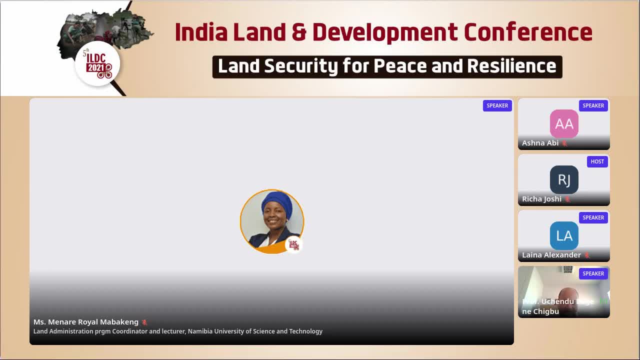 we are moving from specific to general, because what Royo has just presented to you is the underground application of tenure responsive land use planning, as has been done here in Namibia, And what I'm supposed to actually present to you- or I should have presented before Royo- is the practical guide on how to do tenure responsive land use planning. 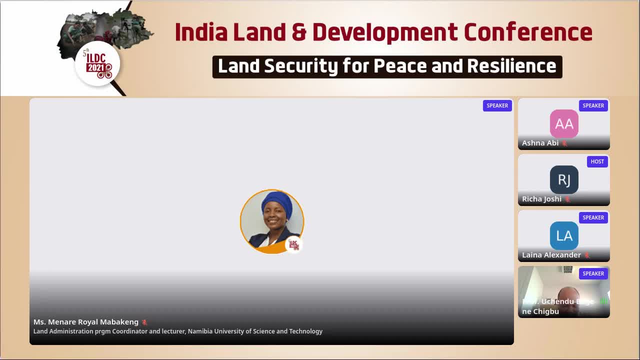 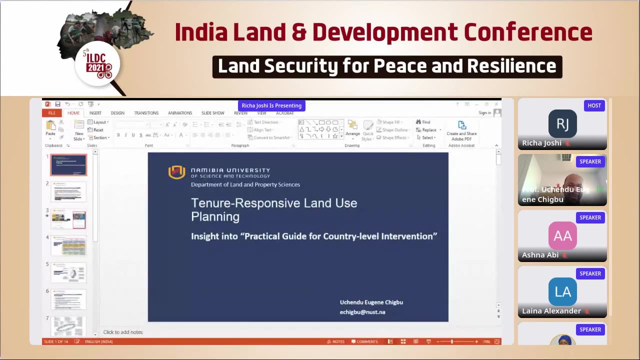 So now she's already on, you know, revealed all the secrets and unveiled all the puzzles, So I would take mine pretty snappy and see if we can have time to have a one on one discussion, if any. So on that basis, I will be speaking on tenure: responsive land use planning. 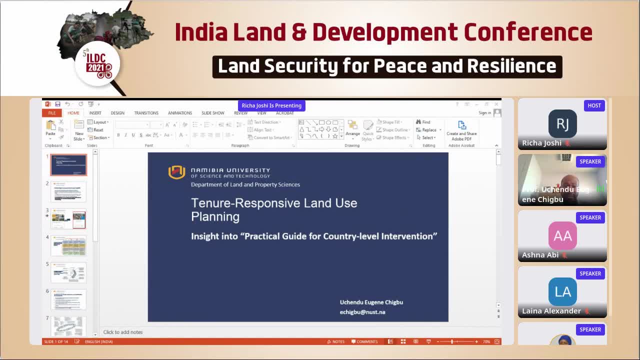 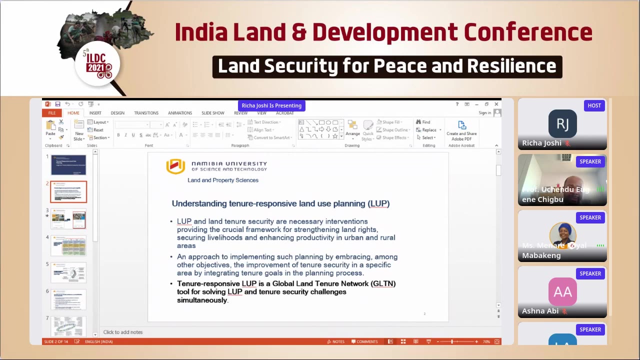 giving you an insight into how into the practical guide for country level implementation. Next slide, please, Emm the my my understanding can. can you please, uh, put it in powerpoint mode? i'm not actually the one doing that is joshi, joshi, can you? 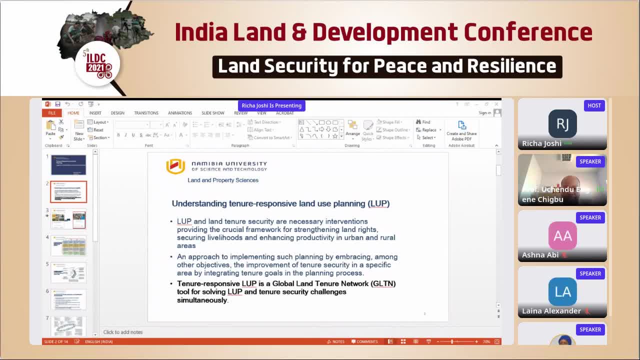 i wonder because, hello, if you pull it, put it in full screen. yeah, for now it's not supporting the full screen. it doesn't okay, yeah, okay, so then we move on. so, um, first of all, i would like to present an understanding of tenor responsive languages planning, and i think that quite a lot of people 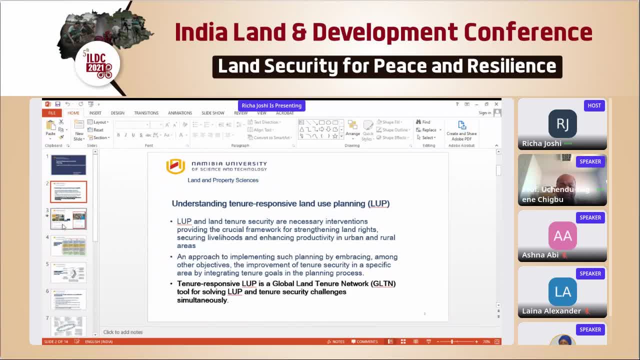 here- at least i see in the audience a few of them um have been part of this um starting from the technical university of munich down to the namibia university of science and technology. and just to clarify that, the technical university of munich and the namibian university of science and technology, 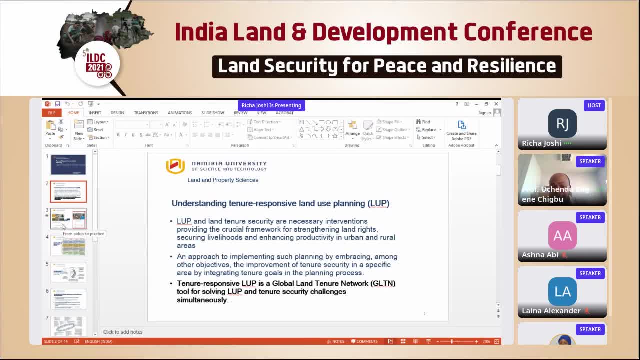 are both, um you know, global land to network partners, and so the work on general responsive language planning is a global land to network partnership task, which is um a multi-stakeholder work, but usually it will be led by one university, and so the technical university of munich initially led. 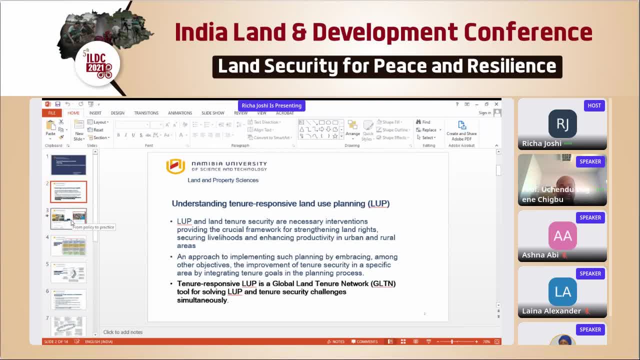 the policy guide, and the namibian university of science and technology has recently- this year- led in a global land to network partnership, and so i think this is a very important part for us, because it is a very important role for us to be able to work on the physical and the 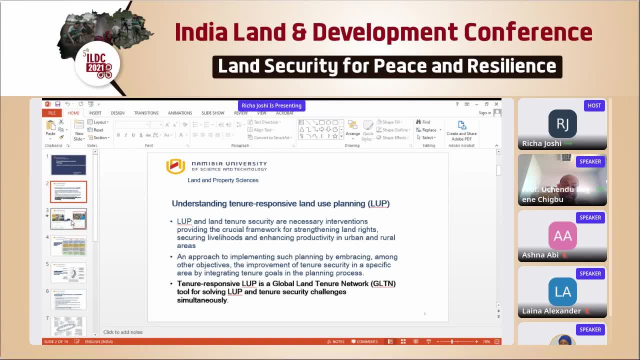 related works of that work. so i think that is a very important factor in um in in providing the practical guide. so the whole idea of tanner responsive language planning itself is that um a focus is now being put on planning when it comes to land uses in terms of stability, location and and so on and so forth. it's an intervation that we 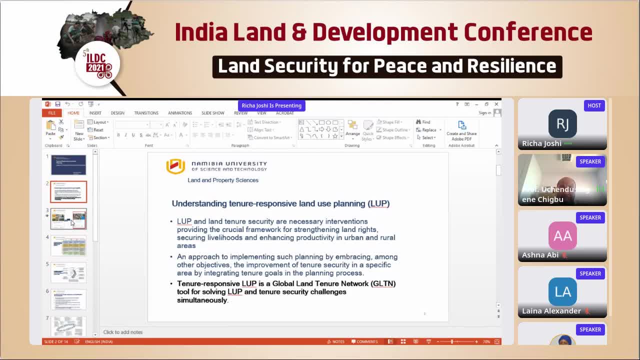 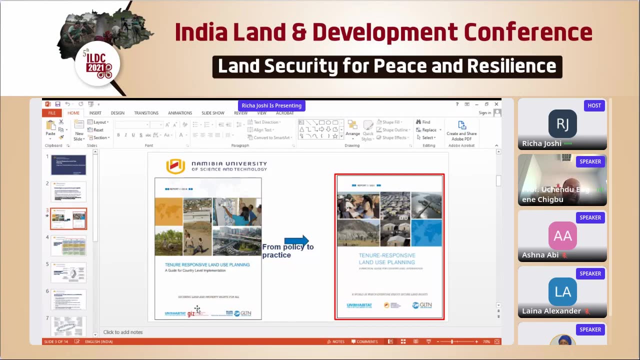 that focuses on the crucial framework for strengthening land rights. so it's a rights-based all about and, of course, with the intention, the objective of, you know, transforming, uh, very critical bad situations in terms of living conditions towards securing livelihoods and enhancing productivity. so, um, the slide you're looking at itself is a transformation. 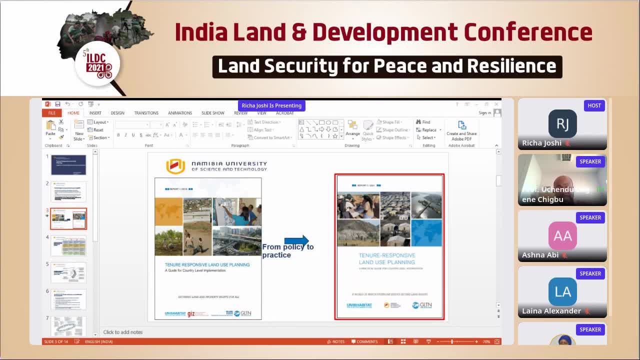 that is, what you see on the left, is the first policy document, which was led by the technical university of munich in germany and then leading to the current one that i'm presenting to you now, which is the uh practical guide. so there's been an evolution in terms of the concepts. 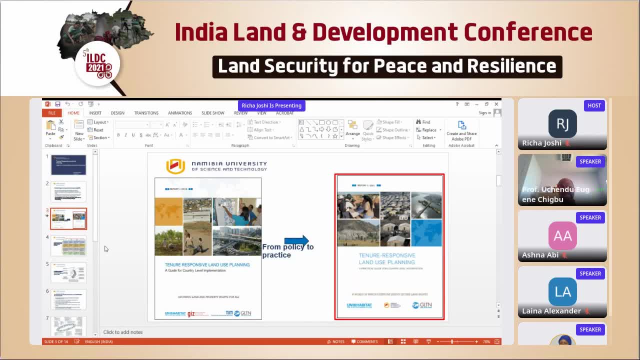 and you know, and policy frame and discourse now towards the practical guide, and this practical guide is what my colleague, uh, lina alexander was talking about- will be launched at some point, um, you know, um, by next month, and that's what i want to give you, the insight. 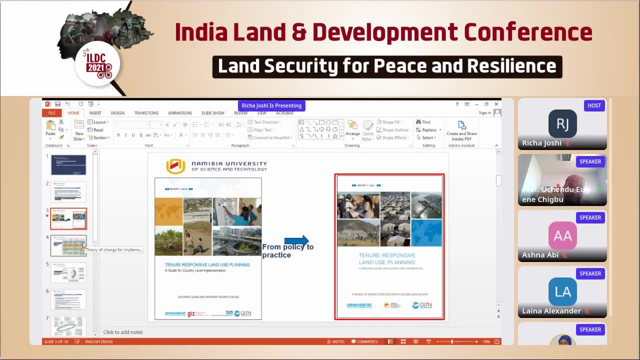 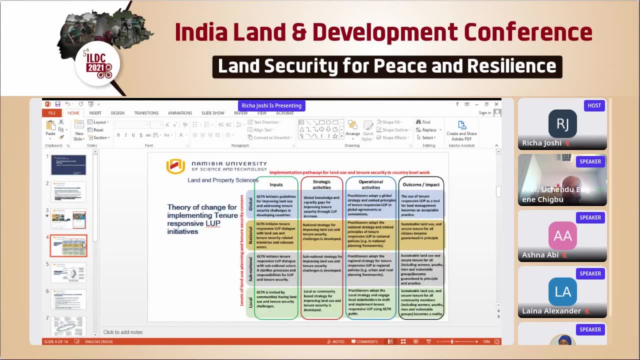 um, you know i want to give you an inside information on it. so next slide, please. so the basic, um, the foundation of the whole idea as a practice, in terms of, in terms of what i'm talking about, is that um tenor responsive languages planning allows for. 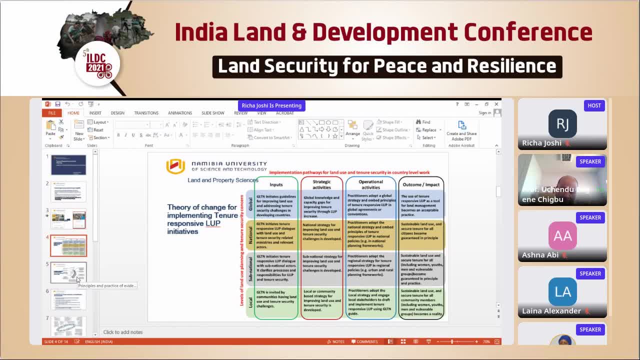 a theory of change in which, um, you know, levels of land use planning have very serious kind of roles that they have to play, but these rules are channeled towards tenor improvement, but the entire idea itself is a measure of land use planning and tenor security improvement. so when you go into this guide, the, the theory of change shows. 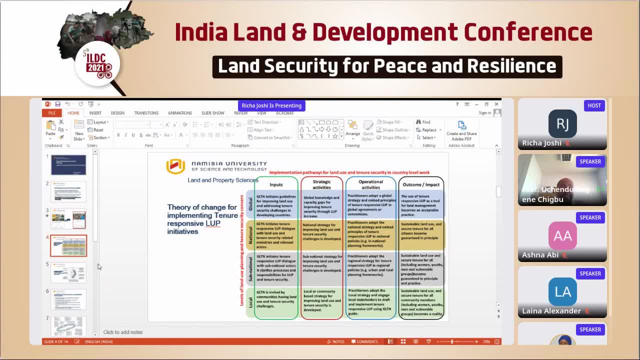 the connections in terms of levels, in terms of roles and activities, strategies, as well as the necessary inputs that actually lead to outcomes and impacts. and i have to say, uh, the the, the guide itself is free, it's available online. if you type in, as i'm talking to you, technology line just planning, you'll get these two guides and you'll see the. 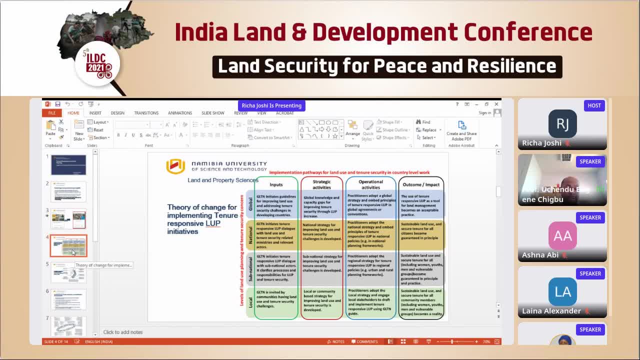 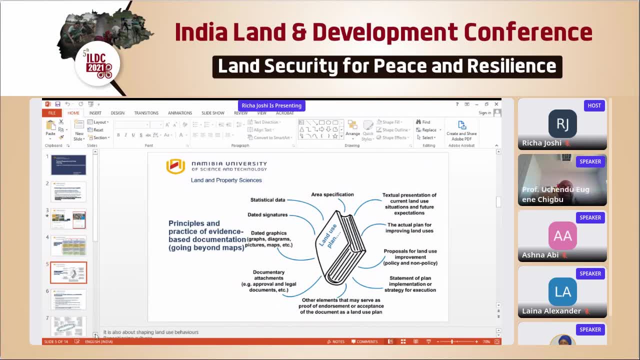 most recent one is 2021, while the previous was 20, uh 16.. so next slide, so the the. what makes tenor responsive land use planning different from other kinds of land use planning? there's a number of different connected planning options, so i'm going to go ahead and see. 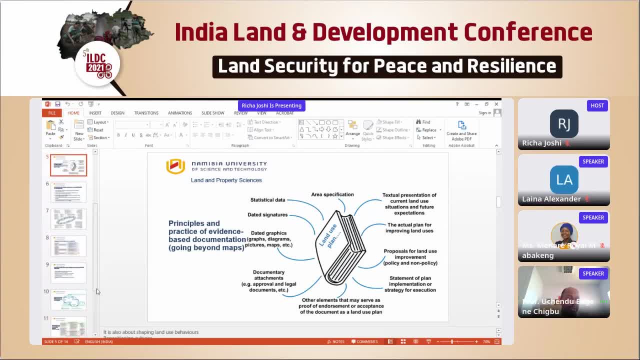 Now, if you were listening to Royo, you must have picked some of these things, but I can express them in a different way. Tenure-responsive land use planning is saying that maps are important, but land use planning and tenure is something beyond map. 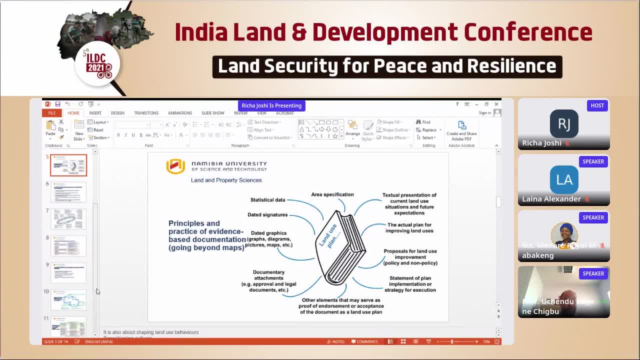 because land use planning and tenure, for it to be sustainable, for it to be efficient, has to rely on human behavior as well. So the human behavioral aspect of tenure, and remember tenure itself, apart from being in terms of periodicity and size of land, 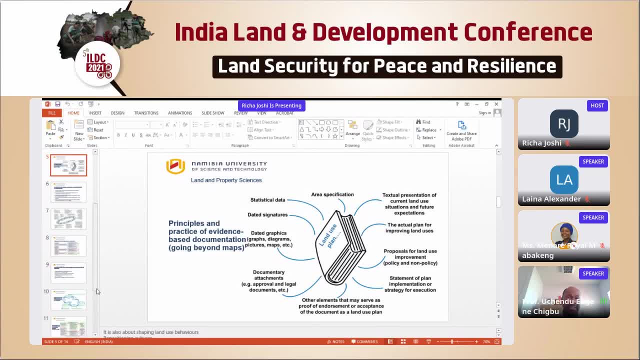 tenure itself. if I put it correctly, tenure security is an issue, is a condition that surrounds ownership, excise of rights, enjoyment of privileges and as well as excise of obligations when it comes to land, And so the tenure-responsive land use planning model. 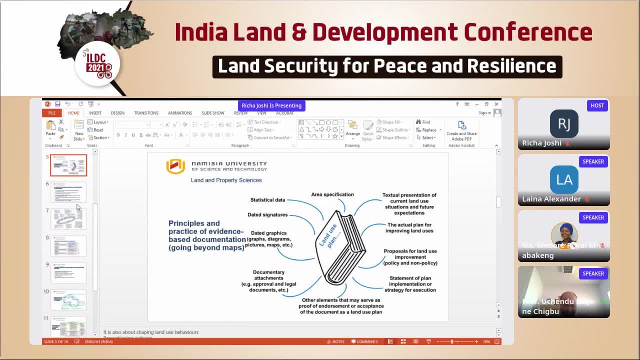 simply says, or tries to portray out there, that digital mapping, statistical data, area specification are all important because they are all part of the documentary evidence that you need to prove either use, possession, ownership or right holding. But it also says that how you deal with a people, 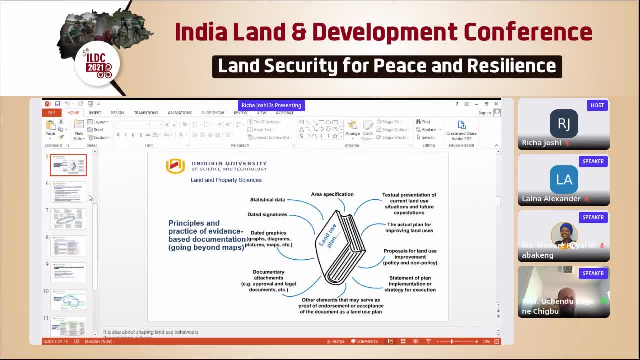 especially when it comes to shaping the land use behavior and how you deal with the land use behavior is very important because the use of land is bounded around a sort of behavior And tenure itself is also linked to cultures, Insecure tenure, of course, in societies where you have high gender imbalance. 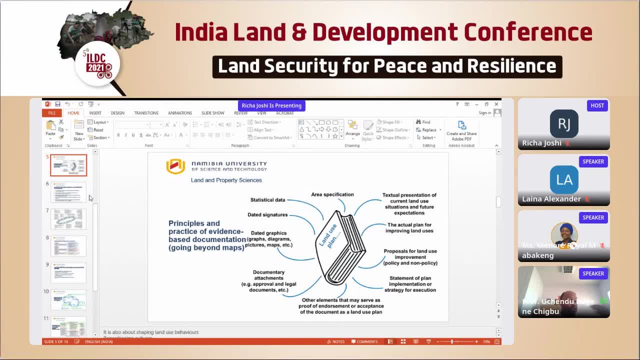 there seems to be insecurity of tenure on one side of the gender, or even in terms of skills when it comes to youth and other vulnerable groups. So it defines land use planning itself not just as a map that shows where map is and what sort of land that is used in terms of stability. 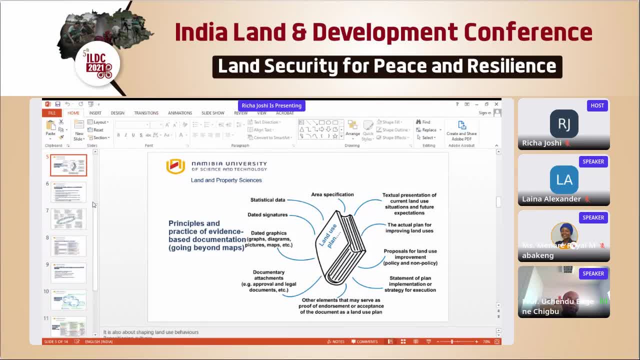 whether it's soil, water, but it's actually saying that it's a compendium of everything, every possible information that you can get in order to a certain provability when it comes to the use, the ownership and the right holding. 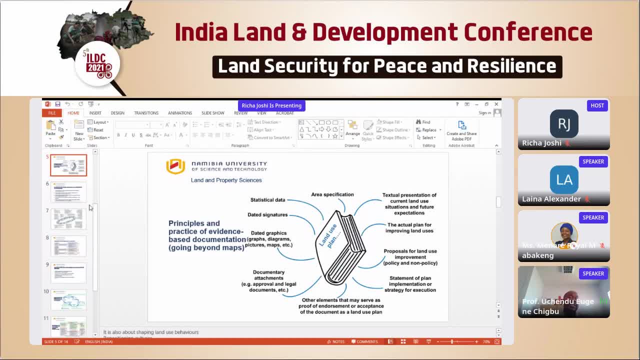 And when it comes to provability, one part of it that makes certain places insensitive and one part of it that makes certain places insecure. And remember, we are within. this is an African day, so I can tell you that when you go and check the pre-index. 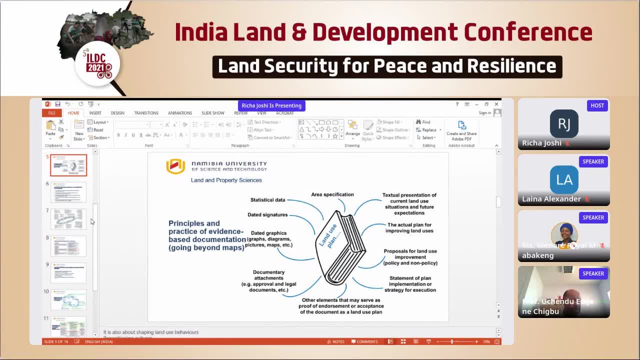 the pre-index data on Africa and probably some parts of a lot, a great part of Asia, you find out that the pre-index assessment last year shows that documentation itself no longer gives security, unlike the theory we have out there And the reason, of course. 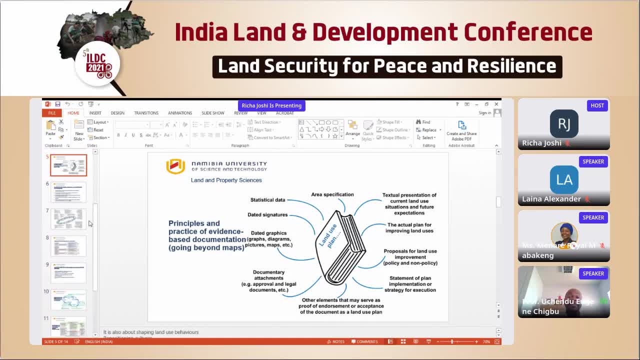 we can't tell us, but the reason from our finding is is because human behavior is part of the entire tenure process, Where you have weak legal framework to actually address conflicts and then you have documentations that are, you know, land data that are well documented. 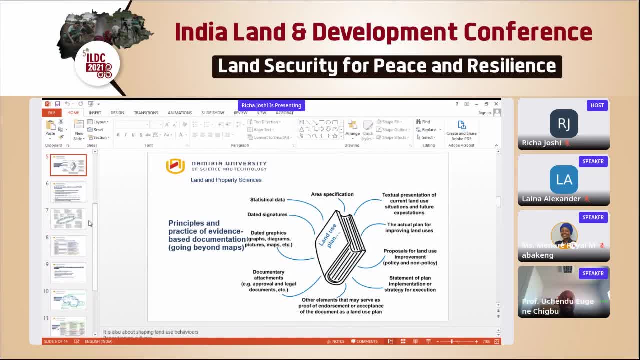 the human behavior part is actually what makes people who hold certificates, who hold deeds and who hold titles secure. Because when a high-ranking person within a community is unable to respect the law and respect the boundaries of your own tenure rights, obviously you feel insecure because the power imbalance would cause problems for you. 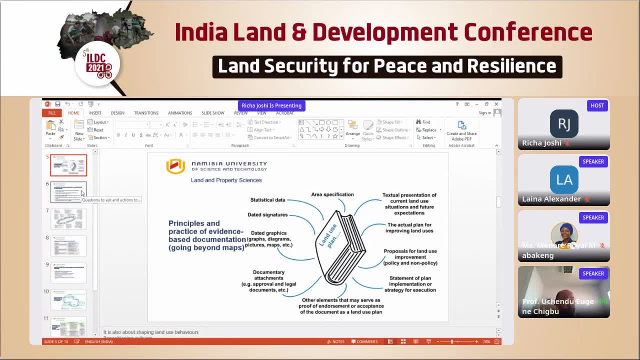 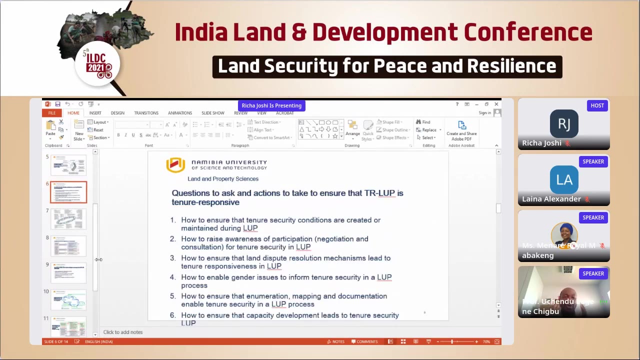 And so the same applies to the common person in the villages, within the informal settlements in the broader CBD area and in rural areas. So behavior matters, And this behavior means that documentation should be something that goes beyond mapping. Next, And what you get in this guide is that it allows for step-by-step approach. 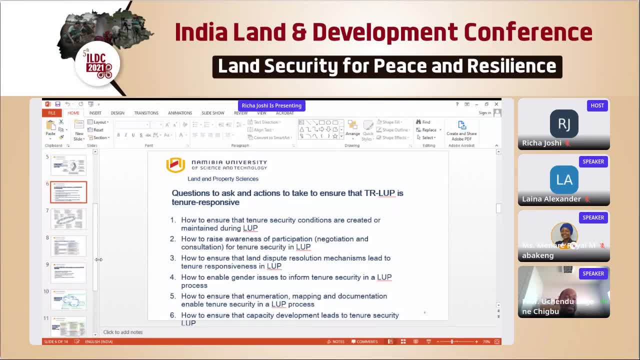 on how to conduct land use planning and as well as recognizing tenure issues. So we have specific questions that one can ask in the course of land use planning in order to ensure that the issue is addressed, The issue of tenure is taken care of. So questions that relate to how to ensure tenure security conditions are created. 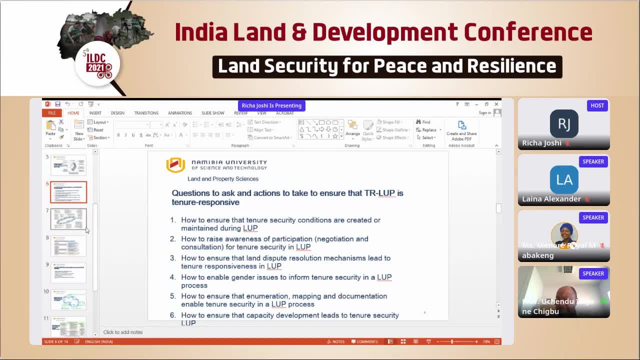 and maintained during land use planning, how to ensure that awareness raising for participation is there in terms of negotiation, consultation, how to ensure that dispute resolution mechanism leads to tenure, responsiveness. And again I come back to behavior. You see, part of land use planning is always the land dispute resolution mechanism. 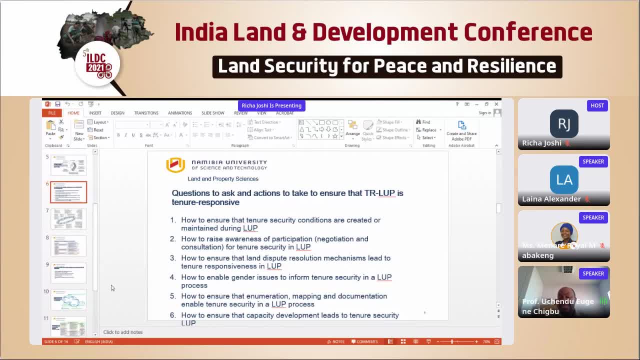 But when the land dispute resolution mechanism is not respected by parties who go through it, then of course you can blame the law, but rather you have to blame human behavior And of course, where human behavior is more powerful than the weak legal systems, socially. 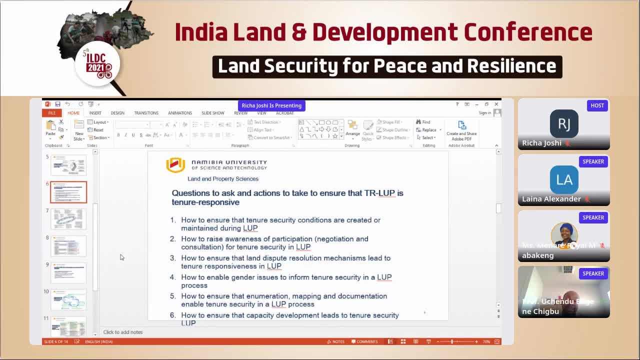 then even those who own land legitimately feel insecure because they don't know how long the piece of land or the right they enjoy from that land or ownership can remain with them, And so that's why this is very important. So when you go to the guide, you have specific questions that need. 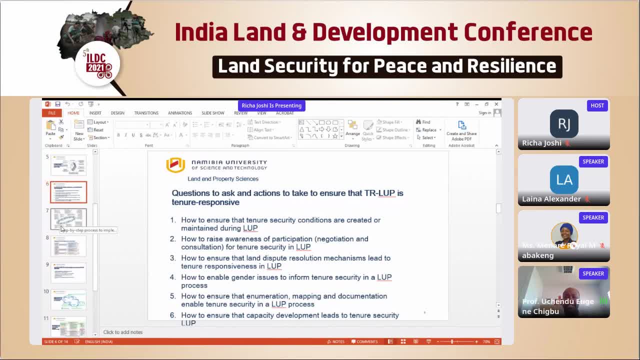 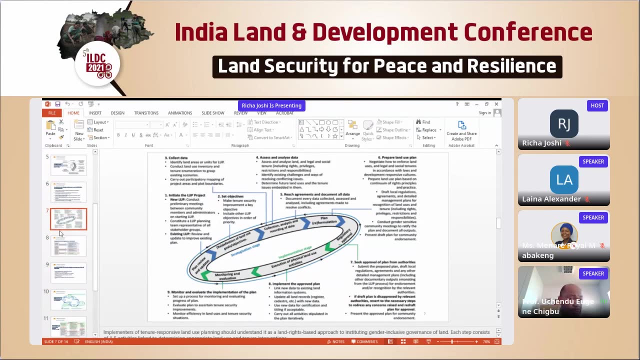 that addresses specific tenure issues which must be put into perspective when conducting land use planning. Next, Now, in this slide. I'm not going to waste your time here, because we can never talk enough of it. However, this is actually what Royal has tried to explain to you. 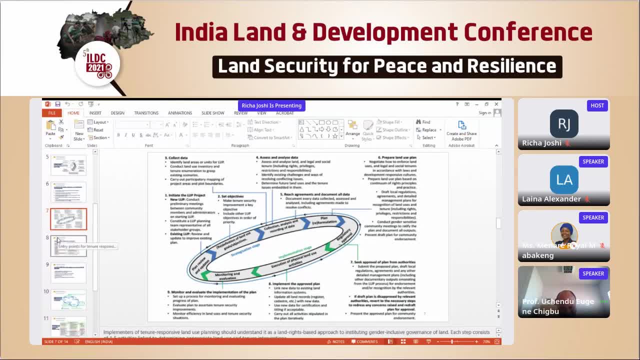 how the work was done in Gubadis here in Namibia. But I have to say one thing is that when we talk about applying tenure-resolution land use planning at the country level, of course it would vary in terms of these steps. 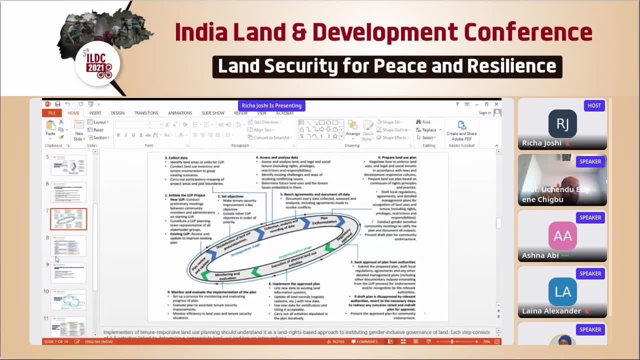 Some steps may come before the other, Some steps may come afterwards. In fact, the system can also be very repetitive and iterative. So I would say that it's There's no one way of doing it. So everything for now remains a guide. 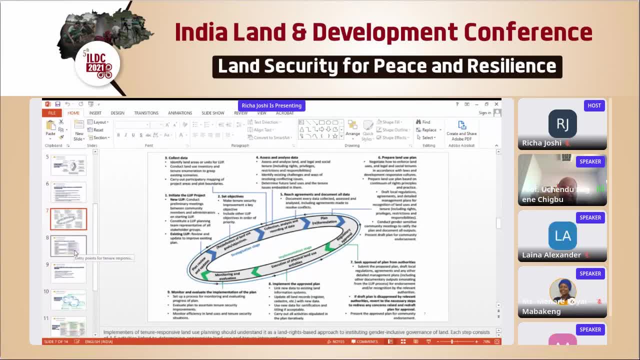 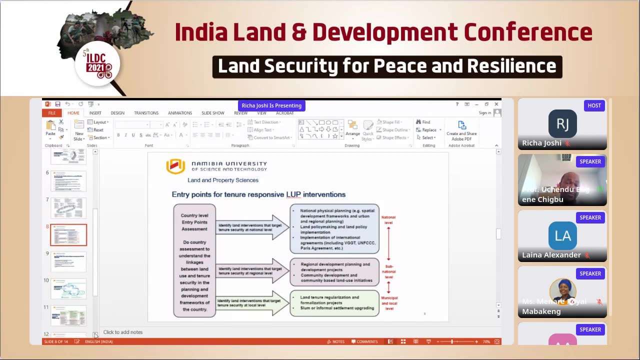 And you can have access to all the nine steps you know within the guides that I told you. you can have free access that is accessible online. Next, But one of the things that has not been there, that we've tried to do in this guide: 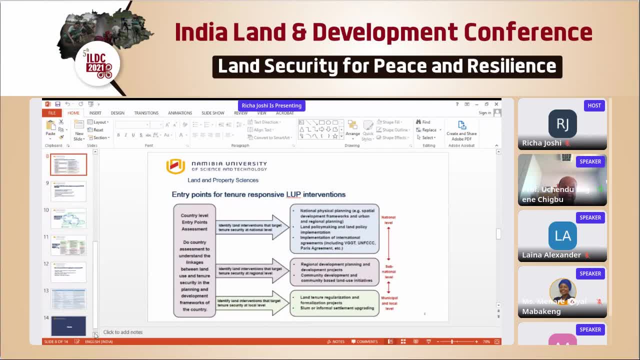 is to identify the entry points for tenure-responsive land use planning, to identify when actually land use planning becomes tenure-responsive and at what point can you make it tenure-responsive. And one of it is that at country level one has to do an entry point assessment. 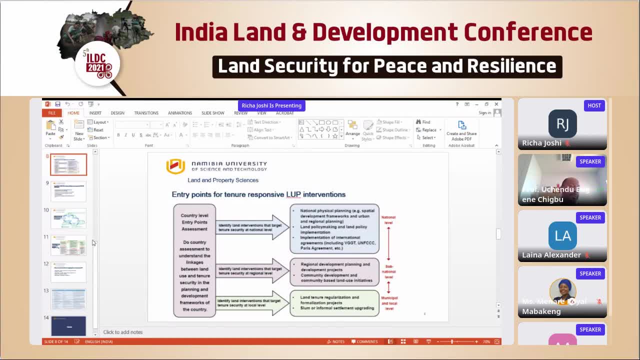 because, don't forget, land use planning is something that we do everywhere, I mean in every country you go. there's some sort of land use control, And what happens in most cases is because the focus is always on land control- Controlling how people use land, what sort of size of land- 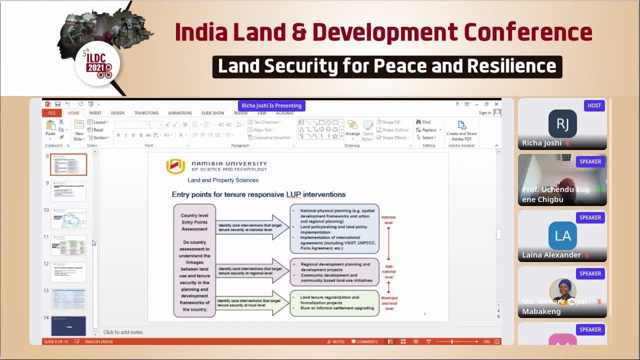 what sort of tenure they can have on land. Because of this focus on control, which I think is a very old planning terminology, because of that, what happens in reality is that by controlling you cannot actually impede on the tenure rights of people. 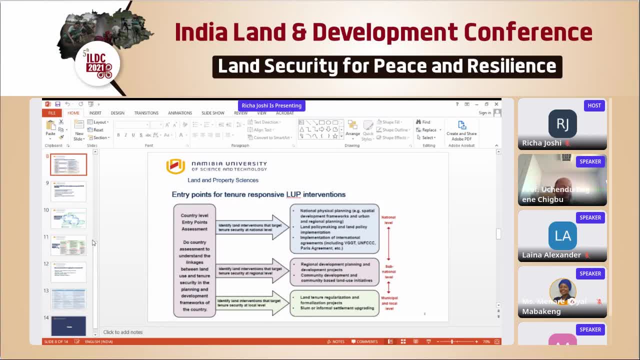 So trying to get a balance becomes, you know, a problem. So when you want to do tenure-responsive land use planning, obviously it is something that you have to do within a broader frame of existing land use planning approaches and strategies. So the question is: at what point do you begin? 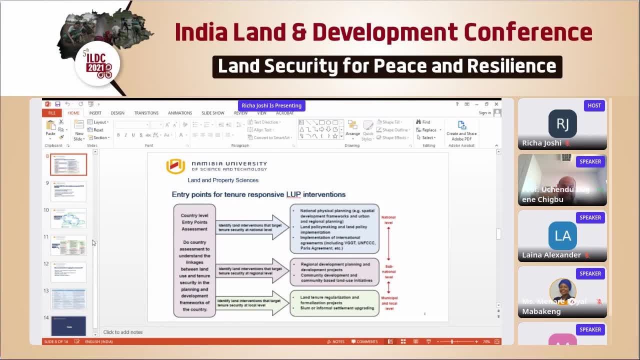 So you have to do a country level entry point assessment And at this point you have to target land interventions that has tenure security opportunities at both the national level, the regional level or the local level. At the national level we have to look at the future. 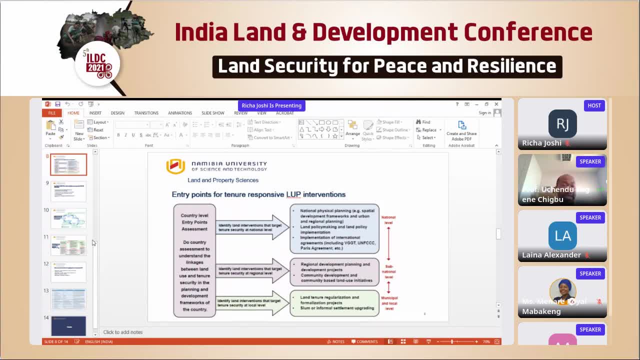 We have to look at the existing physical planning framework to see whether there are tenure improvement opportunities that already exist. At the regional level you do the same, And at the local level you have to look at the issues of regularization and formalization. 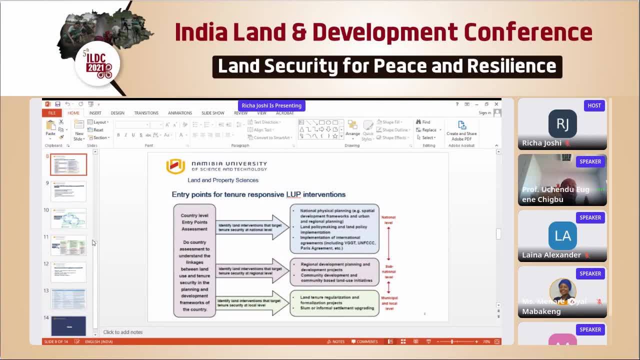 And, of course, the issues of cultural, what I normally would call cultural repositioning, or change of attitudes, And it's really, you know, a critical part of the process, And the only way this works is that you have to keep participation. 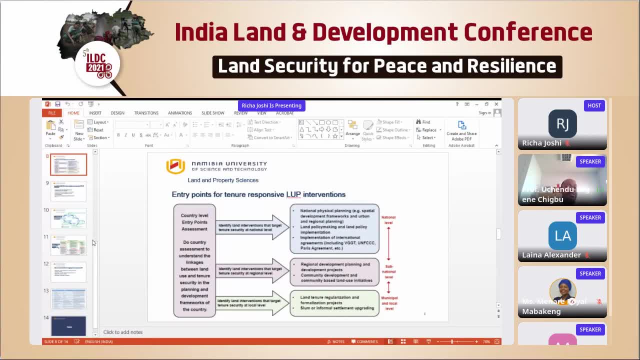 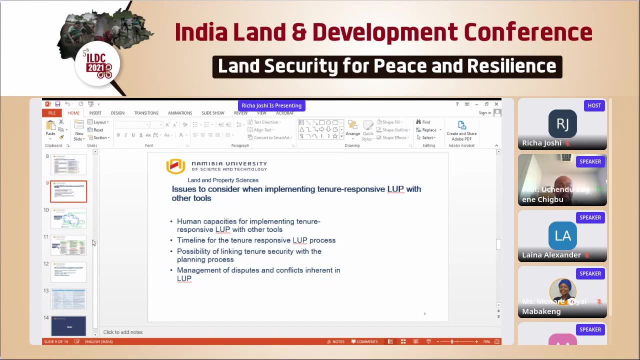 You have to keep participation And you have to keep participation, You have to keep people engaged, You have to keep people working together And you have to keep people trusting each other, such that everyone becomes part of the process. Next slide, So the issues to consider when implementing tenure-responsive. 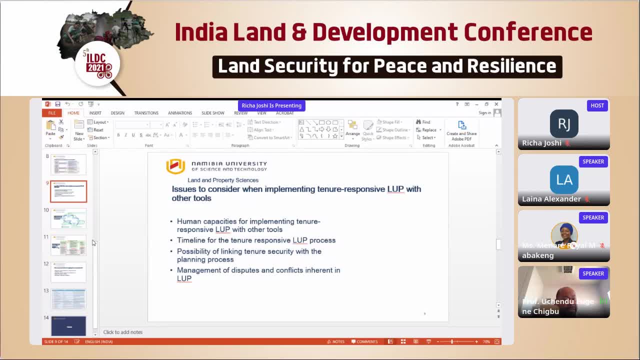 land use planning is the four critical ones is the human capacity for implementing the tenure-responsive land use planning. There's a tendency that, by feature of you know administrative rules, planners planning is meant for planners And so planners must do land use planning. 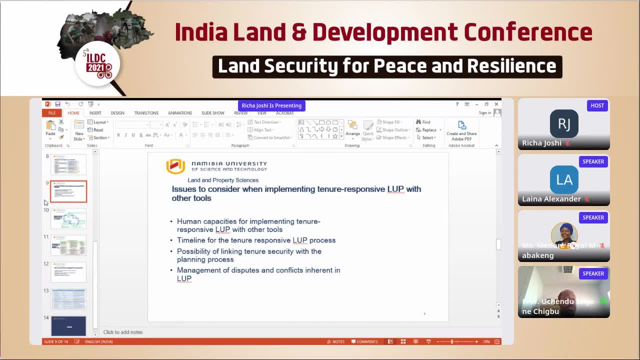 But that's not what we are saying. Planners: a planner is well suited to do land use planning. A land administrator can do land use planning. A land manager can do land use planning. A public administrator can do land use planning. A community organizer can do land use planning. 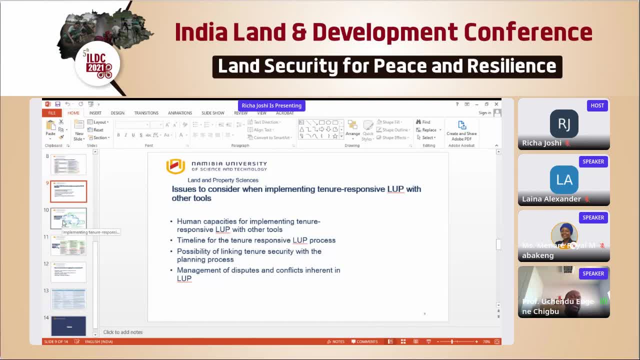 We, from our experience, have found that anyone can do land use planning if they have the requisite knowledge and skill to be what we normally would call an expert generalist. If you're just a planner, it's difficult. If you're just a land administrator, it's difficult. 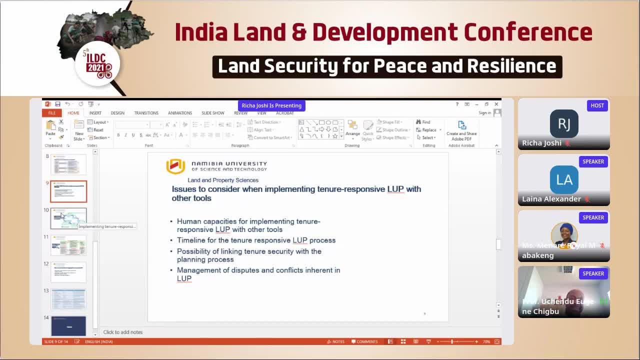 You've got to be an expert, generalist, someone who can understand to a reasonable level a little bit of every other aspect of planning, whether it is mapping, cartography, whether it is social community organization, whether it is networking law. So at this, when you put this together, 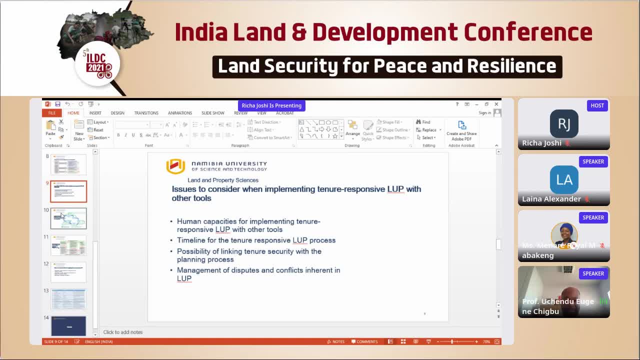 you realize that sometimes the planner is not the best person to do it. However, because the planner has the expert knowledge of planning, even sometimes it can also affect the planners. You can create a bias where a planner is planning but is actually impeding tenure. 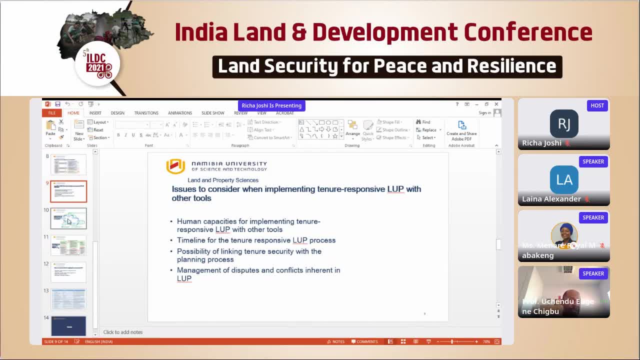 So my point here is that it's an open field. First, the knowledge you need is a general understanding of land management, land administration, land governance and, of course, if you're a planner or a land manager and you have this, of course it gives you an advantage. 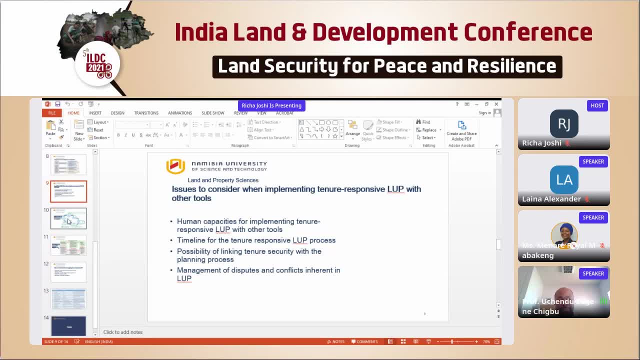 So human capacity is crucial. Timeline is important because you have to do it within tenure has to be done within tenure. improvement has been done within a timeline if it will be useful to people, And then there has to be a possibility to link tenure security issues with the planning process. 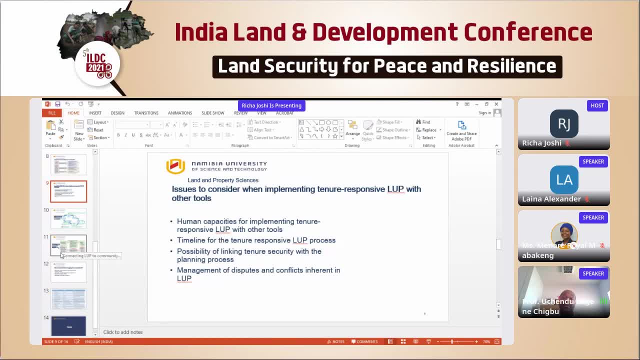 whether it is in terms of data management. the data you get from here has to be linkable to the mainstream land information system that exists within such jurisdiction, And then there has to be that skill to manage disputes and conflicts And, of course, the leadership to be able to navigate. 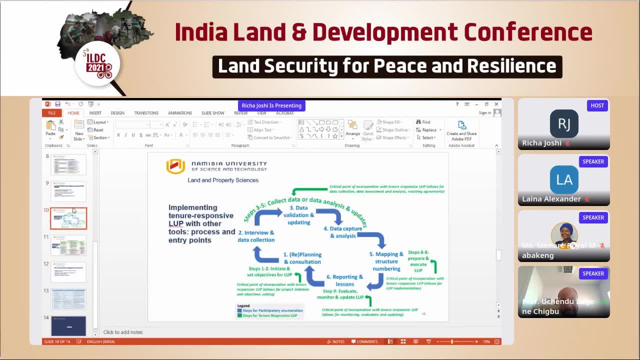 within different professions that are related to land. Then in the next slide, what you see is that implementing tenure responsive land use planning, it cannot be done alone, because no one will really, really it will probably be too expensive to simply do land use planning. 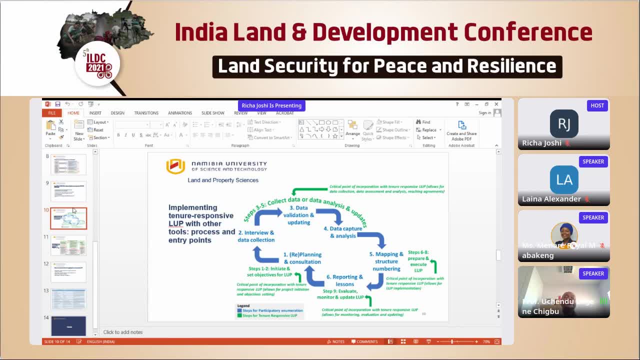 just for the sake of improving tenure. So it would always be that you're improving tenure or there's already land use planning existing and you're adding the tenure objective to reach the tenure goal, or you want to move the tenure goal elsewhere, or you're creating a land use. 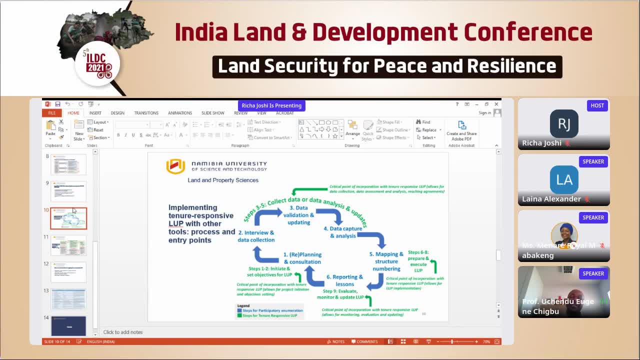 a tenure, responsive land use planning that has to fit within an existing land use planning strategy, And to do that, that means you have to work with other tools and there has to be entry points, And what we have in the guide is that we show areas that allow you to link these entry points. 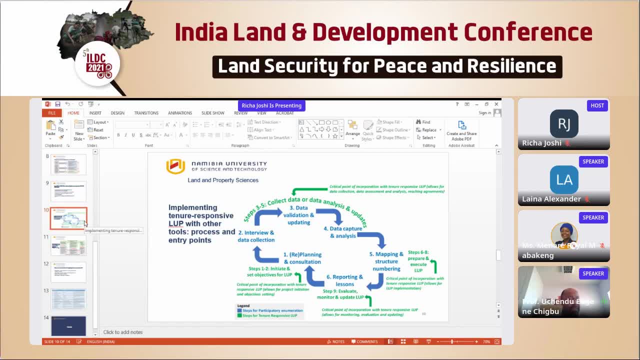 places like at the point of data validation and updating. you can move in through various means of data management to bring the tenure issues in. It can be terms of data capture analysis. It can be mapping, which we all believe is very, very crucial. 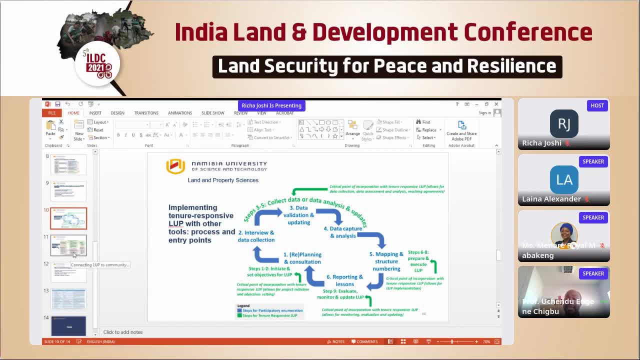 and must be a critical part of any part of land use planning. And that means visualization matters, because then people can see the land even when they're not on the land, They can see what the features of the land is even when they're not on the land. 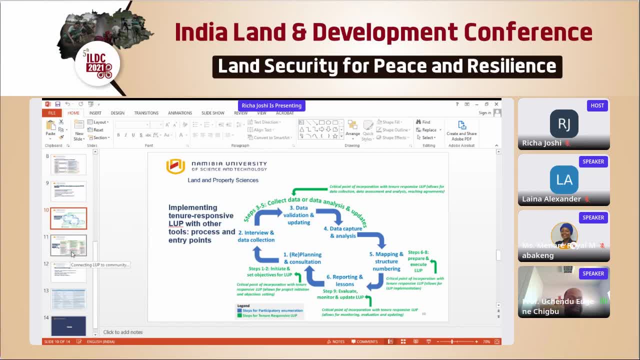 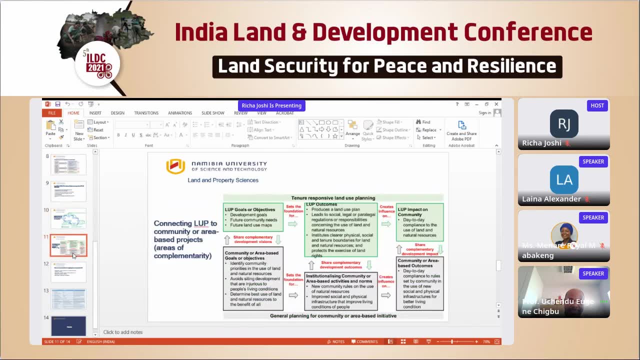 And you can do that in terms of the reporting stage, at interviews and data collection, as well as the planning or consultation stages Next slide. So another crucial thing is that, because tenure responsive land use planning is a practice that links very much to human behavior. 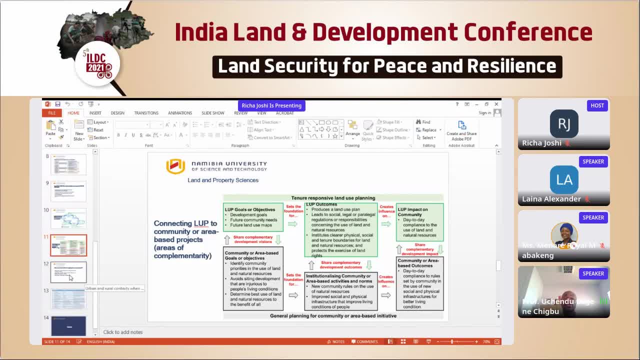 links very much to capacity development, links very much to spatial data infrastructure, how you handle it and how you manage it, what data you consider to be relevant and what data you consider not to be relevant. We, on matter of principle, believe that any information that is related to land. 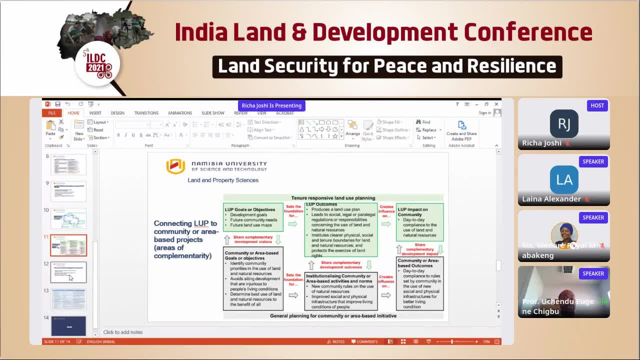 constitutes data and should be used and should be stored or managed under this situation, because you never know when such data can be used as a tool for provability, because one of the things around tenure security is that it's got to be provable And so the people around you are part of that probability. 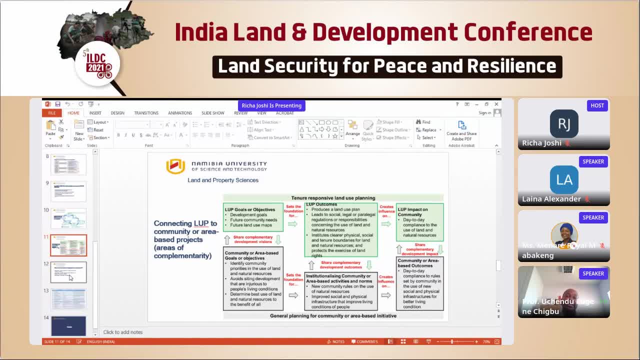 Your neighbor is part of that probability. The data that is stored in digital form is part of that probability, as well, as the data that is stored in oral form, in terms of oral documentation, is also part of that probability, But then that usually relies on the level of trustworthiness. 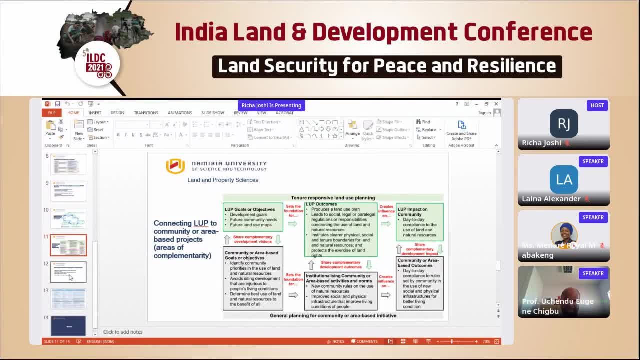 and the level of honesty of people around you. So for you to do that, there has to be a connection to community development, because communities are about people and tenure security. you don't do it for just the environment, you do it for people in order to curtail. 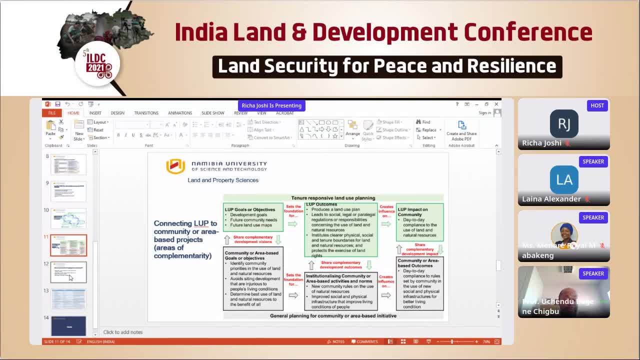 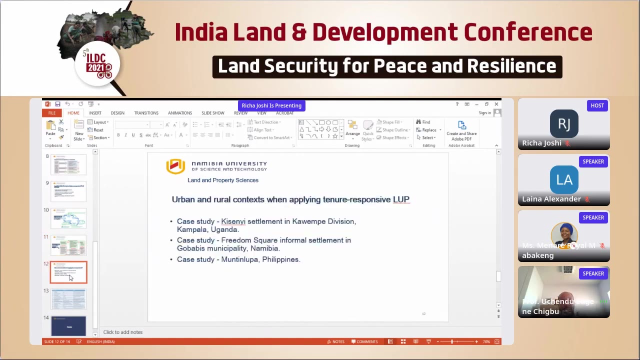 for them to use land responsibly and as an investment, And so what you have here is the connection between land use planning to community or area-based projects. So we have linkages to it and you'll find this in the guide. Next slide, Also in the guide. 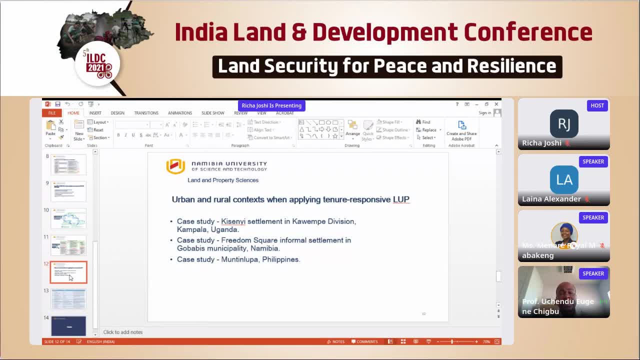 you'll find that, although I speak about tenure-responsive land use planning as something kind of unique idea, but it's something that has been there always. We have cases in Uganda in the Kisaya settlement- also a slum in Kampala- where this has been practiced. 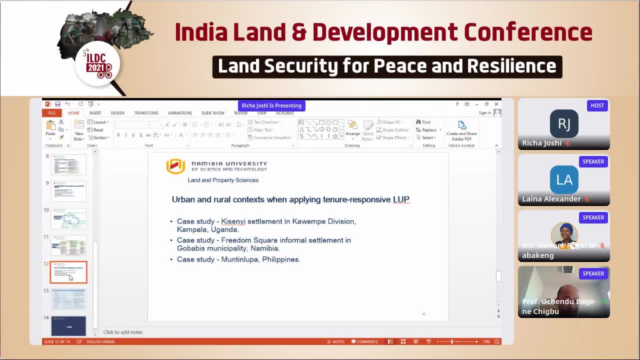 We have in Gubabis. it is there. it's been practiced in a different way, And in the Philippines it's been practiced in a different way. But one thing you tend to see when you go to these places is that there's always the GLTN. 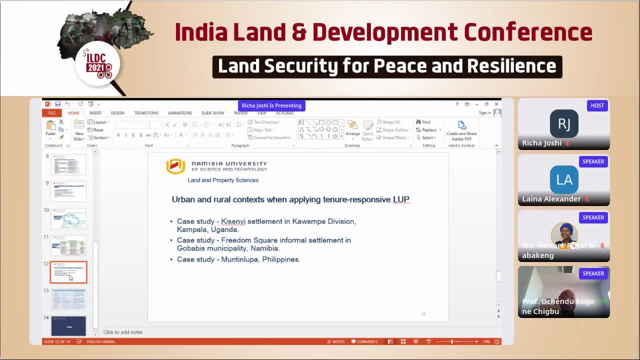 the Global Land Tool Network being part of it. So it's been an idea that's been in the oven for a while and it's being tested, and right now it's being piloted as well, But it is actually from existing scenarios of land use planning. 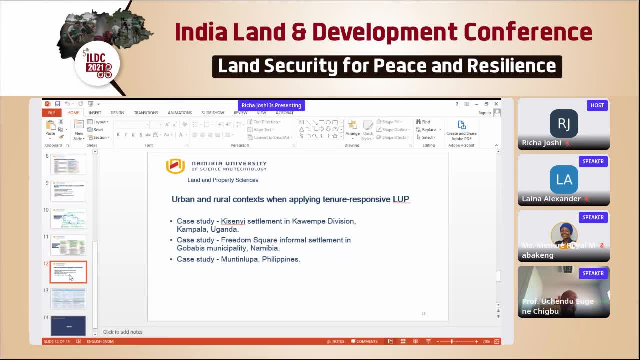 it is from there that we actually drew the idea to start emphasizing on these things, And many times, although some of these people do not get enough credit for it, it's actually the communities that these ideas come from. And I have to say, 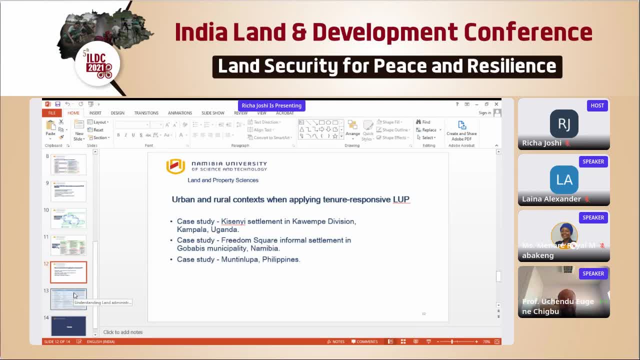 just to add to my colleague, Lina Alexander, when she was speaking: yes, the tenure-responsive land use planning thing is also one of the areas where, as a university, as an organization, an institution, we believe that we are making an impact. 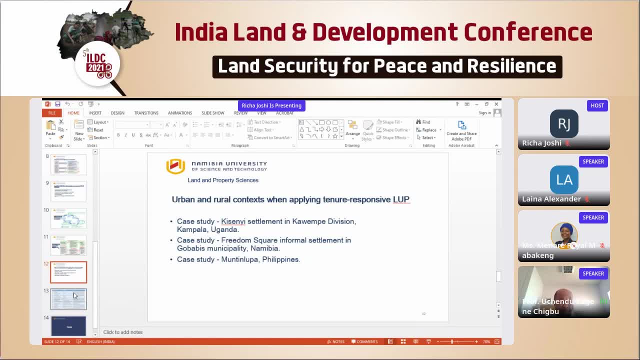 direct impact when it comes to development. It's been endorsed by the UN Habitat, by the GIZ, and it's been piloted, as I'm talking to you, in the Philippines, in Uganda and in the Laos, So it's something we want to keep talking about. 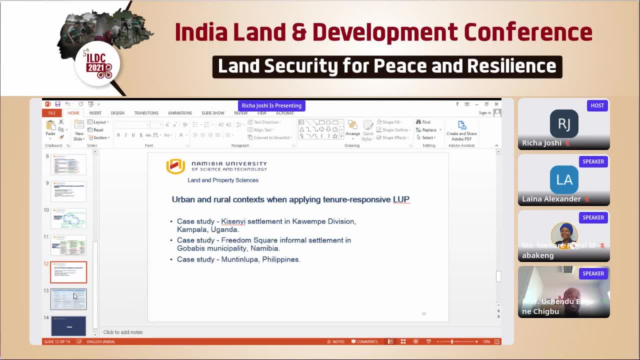 but it's been practiced in different ways, and that's because jurisdictions and cultures change. So case studies are important and you can find them in the guide Next. So why do we even have to worry about this? Why try to work, do research? 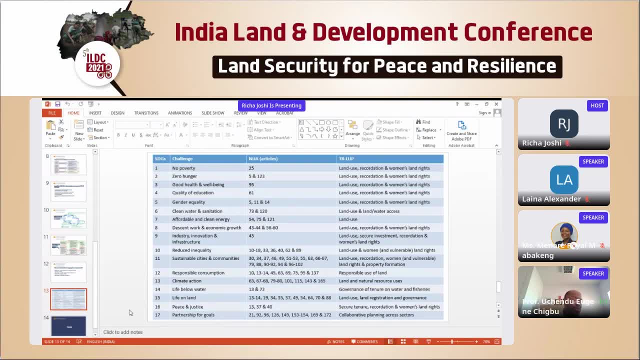 meet communities, work with communities, to simply provide a guide on how to do land use planning, Because land use planning was there before any of us here were born. but it's just because we have to find a better way to do it. because, as the UN Habitat says, 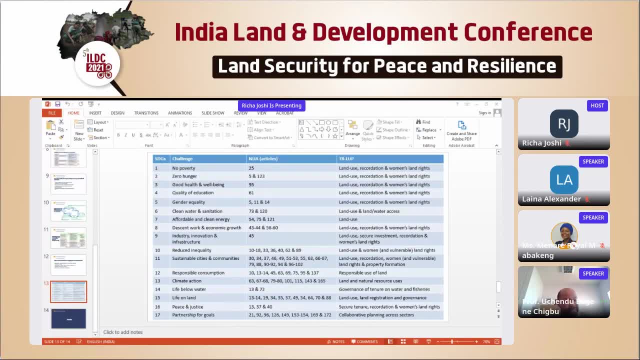 because, as the UN Habitat has shown, in fact, evidence from the UN Habitat says that for the entire developing countries to be secure- and we're talking about in terms of mapping and recording- you need about 600 years, And that of the FAO is. 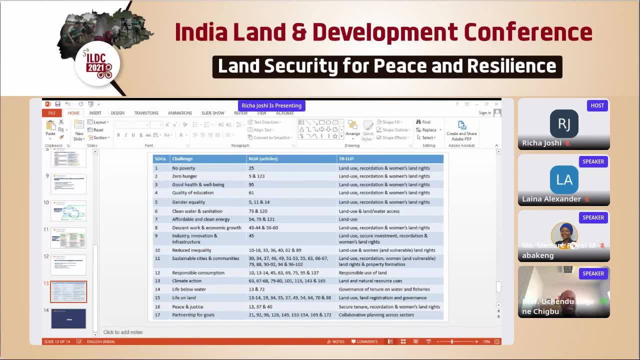 actually FAO is pushing it to nearly 1,000 years, And so one cannot wait for 1,000 years or even 50 years to do something we could do now, And so the whole idea is also that it links very much to the 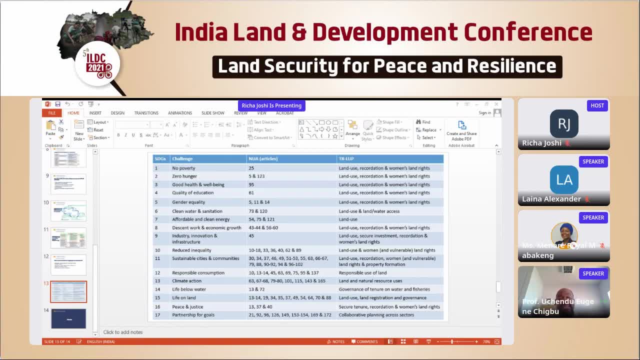 Sustainable Development Goals. So what you'll see on the slide is the Tenure Responsive Land Use Planning and how it links to the Sustainable Development Goals and the New Urban Agenda. So on the far left side you see the Sustainable Development Goals from one to seven. 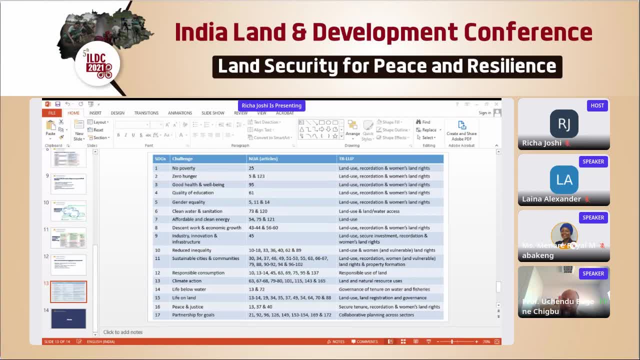 and in the middle the Sustainable Development Goals defined as challenges. And then the New Urban Agenda is showing articles of the New Urban Agenda that are linked directly to Tenure: Responsive Land Use Planning, And on the far right is Land Use Planning: Tenure: Responsive Land Use Planning. 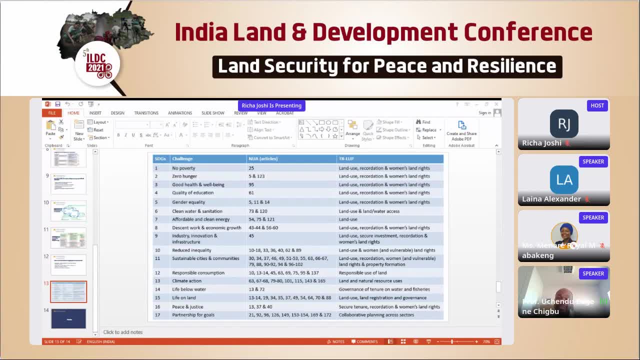 is where we are showing components of the Tenure Responsive Land Use Planning. that is actually a linkage point to either the SDGs or the New Urban Agenda, And what you see there is that land use recordational. women's rights is always reoccurring. 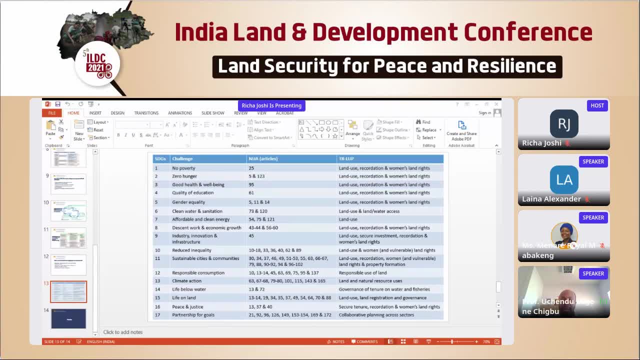 Land, water access is always reoccurring, Governance of tenure is reoccurring, Responsible use of land is reoccurring, which I term behavior, And then issues of recordational collaboration keeps reoccurring. So I will end here and simply say: 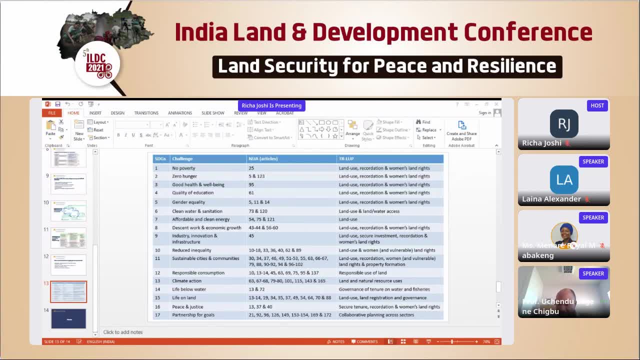 thank you to everyone And then we can have a chat. Basically, we have about 15 minutes To continue and maybe have a discussion as to what you've heard, But this is the Tenure Responsive Land Use Planning Practical Guide, which you have already freely available. 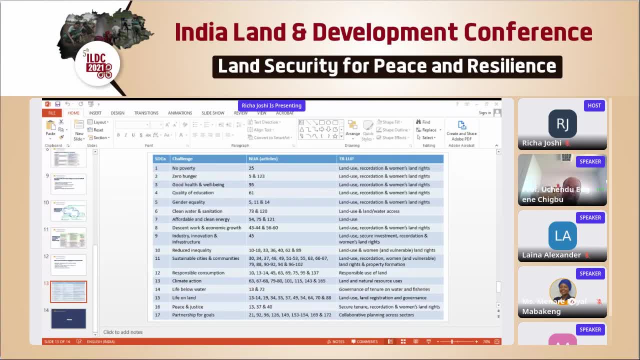 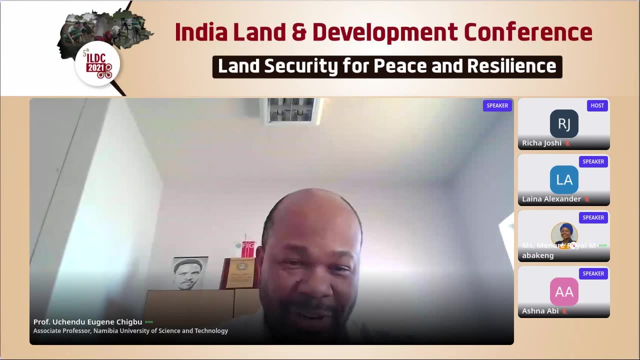 and which we intend to launch sometime in early December. Thanks very much. So it's a little bit strange that I'm the moderator and I just finished presenting. Okay, So, Roya, were you watching, If there's any questions? So what we have is that we have a comment. 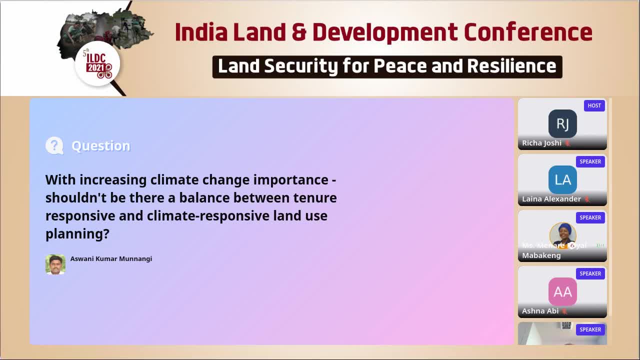 with increasing climate change? from Aswani, He says: with increasing climate change, importance shouldn't be there, Shouldn't there be a balance between tenure responsive and climate responsive land use planning? So that's his question And, yes, it's also on the screen. 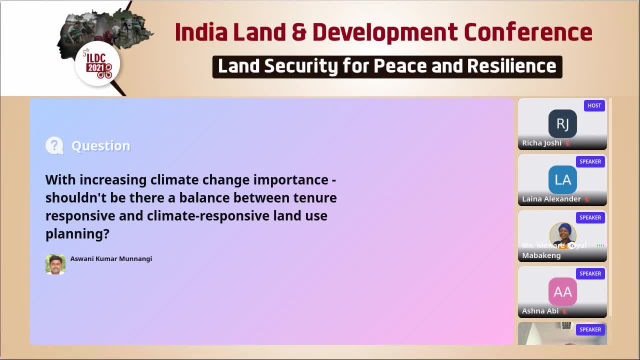 Should I go or you want to go first? No, you can go ahead. Okay, Yeah, Thanks very much, Aswani. That's a very critical question. And, yes, your question is: shouldn't there be a balance between tenure responsive and climate responsive? 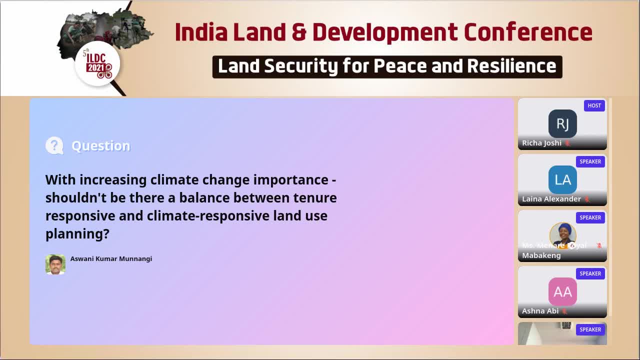 land use planning. I kind of think we are mixing terminologies here, but yes, I totally agree with you. There should be a balance And that balance in terms of policy. when you look at the tenure responsive land use planning, you will see that climate change issues are taken care of. 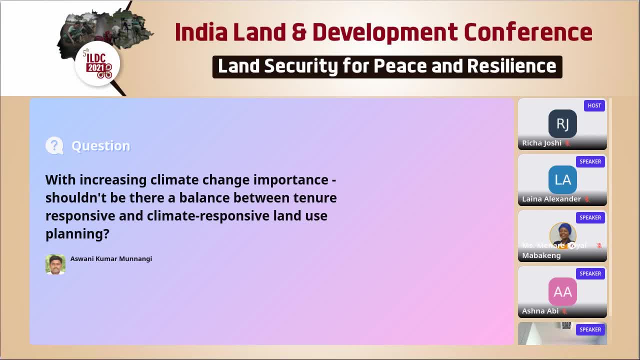 But, of course, the climate change concern is a very, very broad issue. We can, you know, being tenure responsive, whether it's in terms of land use or in terms of environmental management, landscape management or in terms of planning. 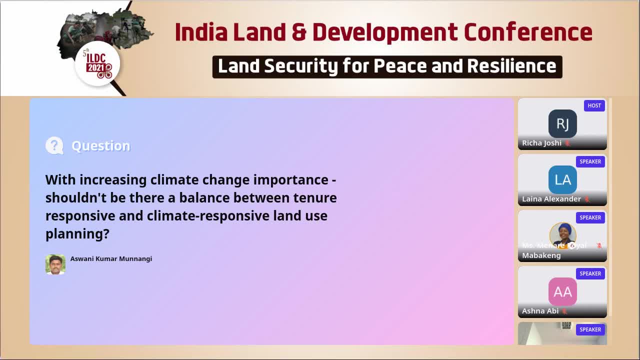 definitely will contribute to improving climate change situations, But it's not all and all. So just to take it for that, because we understand this, in the Global Land Tool Network we are actually at the moment working on. the Global Land Tool Network is working on a different tool. 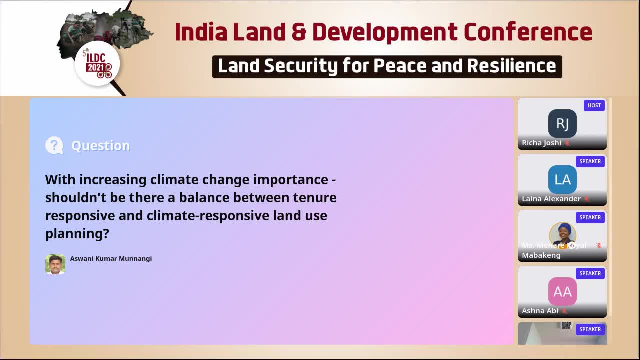 And that is the Namibian Investor Service, the Namibian Investor Science and Technology. My institution is very much at the heart of it, with a colleague taking the lead from the RMIT University in Australia and other partners, And we're looking at the connection between land rights. 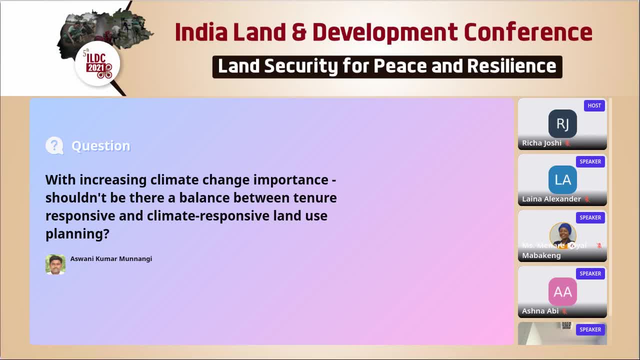 and climate change And when you look at the connection between land rights and climate change is tenure. We already know that with tenure, when people hold a right they believe they judiciously or socially can control, then the way they use land is always different. 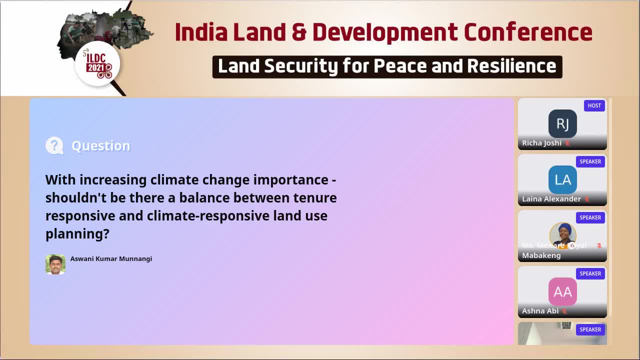 And if you watch also whereas in the climate discourse, you will see that many of the countries that are much more concerned about climate change and who are pumping more money into climate change and who are being committed to climate change- majority of them. I won't say it's all. 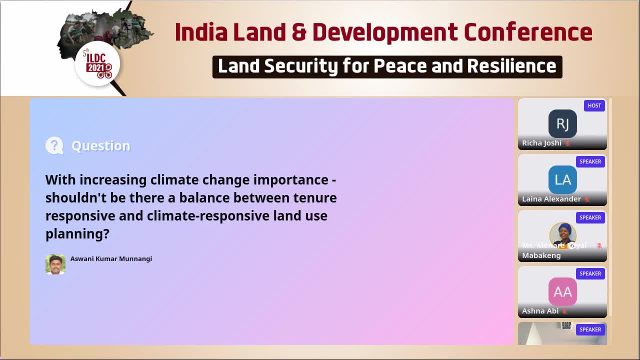 because US is. sometimes it's difficult to categorize US when it comes to climate change issues. Many of them are countries where you have very strong and secure property rights, Because when people have secure property rights, then they have a tendency. 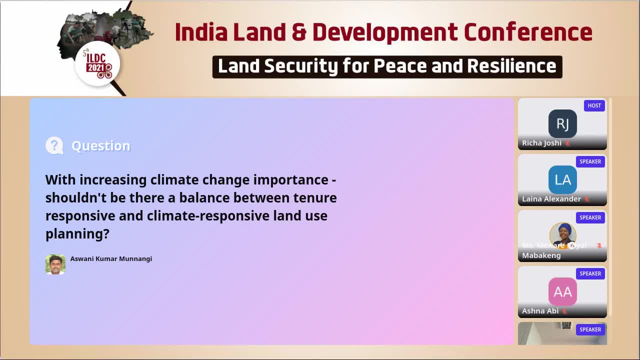 if they choose, they want to contribute to the climate commitment at the individual level. they are able to do that because they have- probably they are enjoying the best form of tenure and so can make every form of decision they can make on land. But when you don't have that sort of right, 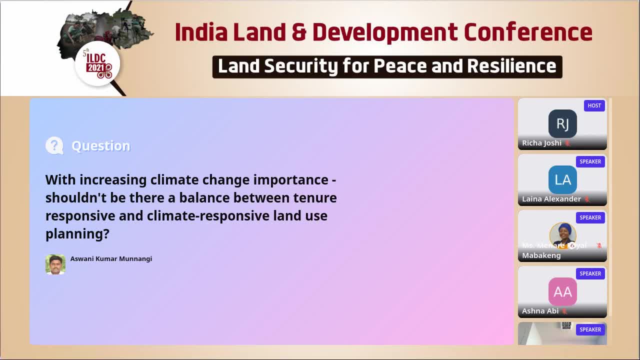 that is superior for you to make decisions- even decisions in terms of alienation, decisions in terms of exclusion, decisions, in terms of abstinence from certain land uses, when you don't have that sort of right to make them- and usually people in informal settlements don't have it. 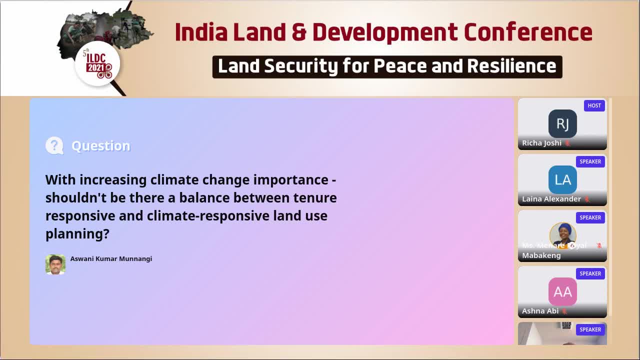 people in certain places don't have it- majority of places don't have it- then it becomes difficult for you to follow climate rules, And so tenure is a key part of it, and so the tenure responsive land use planning itself is a climate responsive strategy. 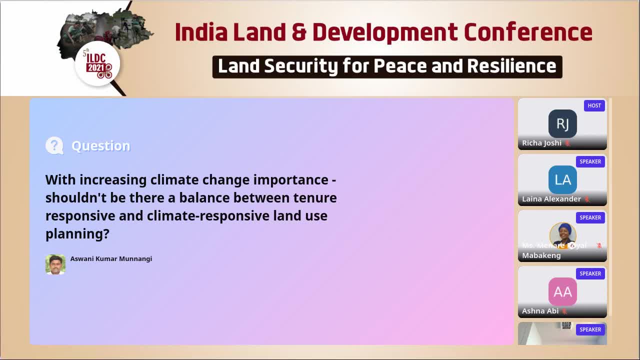 in terms of from the planning aspect, The only thing I would say is because, also, when you bring it into the climate equation, there are more factors that lead to the negative climate change we are having than just tenure. But if we can address the tenure aspect, 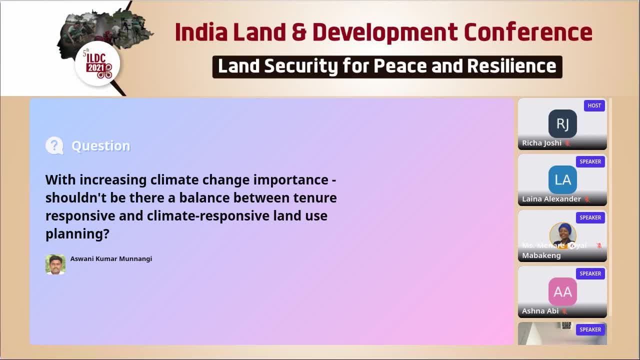 then, of course, I think the balance, theoretically, is there. The question is whether we can shape our land use behaviour and we can change the culture to adhere to it, And that's where tenure responsive land use planning is different from other forms of planning. 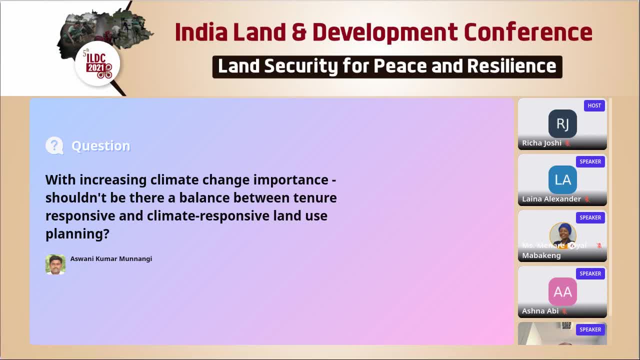 Thanks very much, Roya. maybe you have something to say, Lina, With the comment on shouldn't there be a balance between tenure responsive and climate responsive, I think you have dealt with it very well. I'm going to move on to the next question. 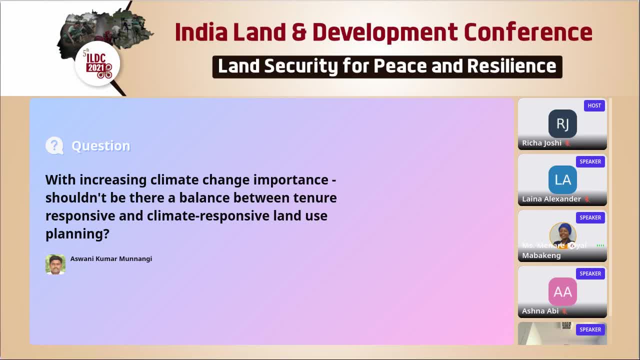 which is from Moses. He says: in physical reshaping of land parcels and planning of informal settlements, how do you protect the value of unbuilt spaces? So I'm going to start off by attempting to answer this, and then you can add on. 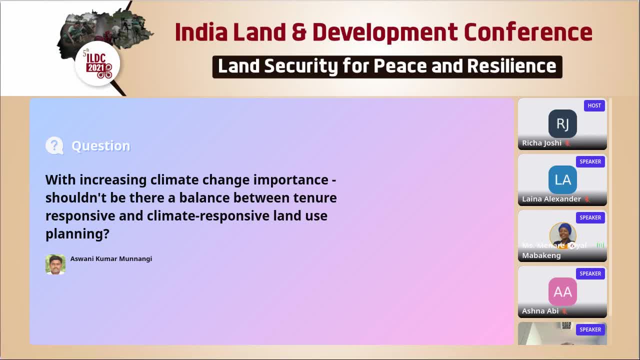 Lina, Alexandra, you're also free to contribute here. So what we have seen is, and from the interpretation of the question of unbuilt spaces, is any or all the open spaces within an informal area that have not been occupied or constructed by anything. 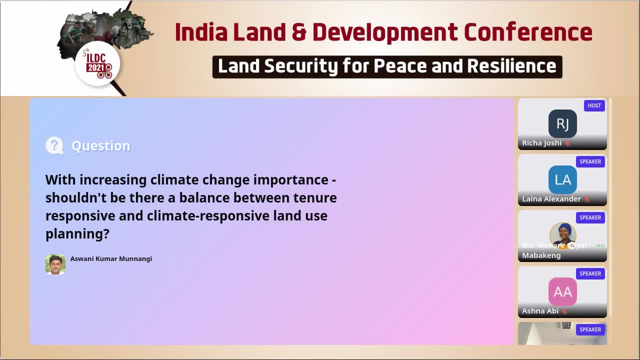 What we do take as a first step in any planning or designing process with the community is to start identifying what are the assets that are available within an area. So those here are your open and built spaces. Those also is your sort of protected trees that you do find in the community. 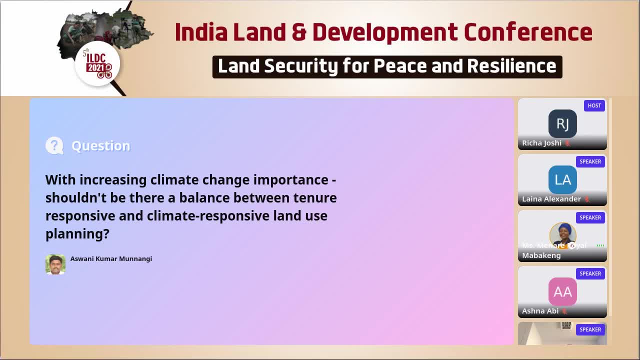 And then also identifying what are the areas that are mostly affected by flooding or are prone to some hazards. So the way unbuilt spaces are protected, I would say, or the value of unbuilt spaces are protected, is through community consensus. And what do you get to maintain? 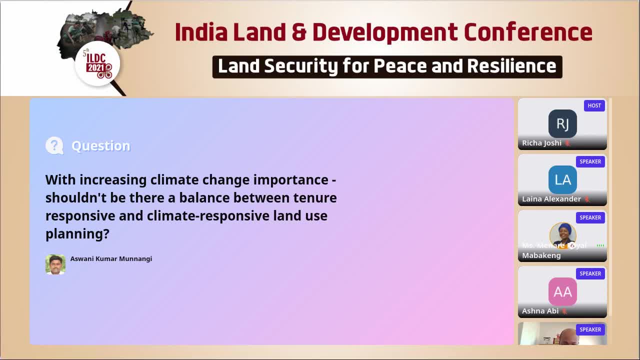 and what do you get to build on? I'm answering it more openly here. So what we have seen in the projects that we work with, there is quite a promotion of open spaces within the area. So we have a new layout. It is also a requirement in planning practice in Namibia. 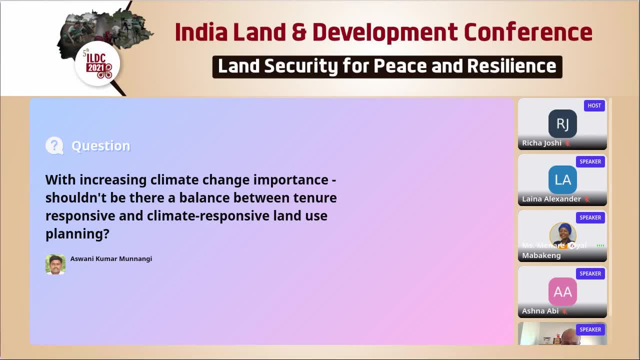 to maintain a specific percentage of open spaces that can be used for community activities. So it comes from consensus and also ensuring that when we do plan for informal settlement upgrading, we also stay in within the requirements, the formal requirements of town planning, Because any planning that is done by the community 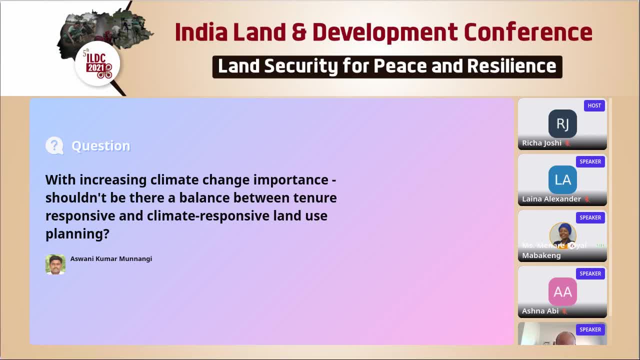 later on has to be approved on a national level within the planning regulations. Thanks very much. I would ask Ms Alexander if she wants to say anything before I go on. Lina, are you there? Okay, I'll move on. 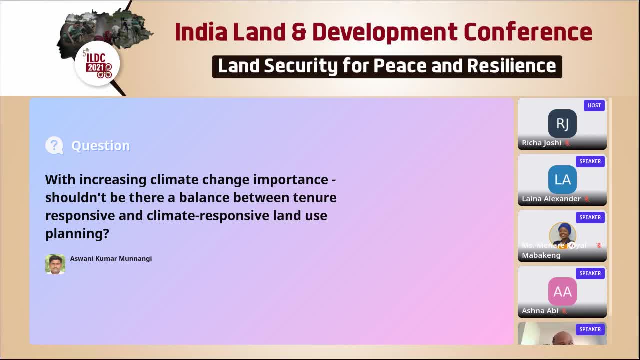 So thanks very much, Royo. I think you handled the question from the perspective of informal settlement. And for the person who asked the question, one thing I have to say is the Tenant Responsive Land Use Planning approach has not been there for a long time. 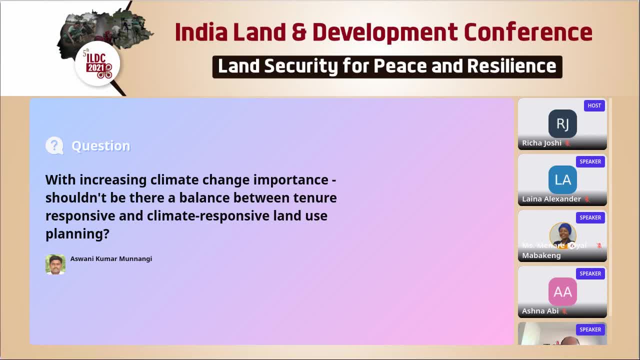 You can see that the guide was just published this year for practical application, So any responses we are giving to you at the moment are purely based on responses that we can only derive from when this was tested before now. starting with what Royo said, 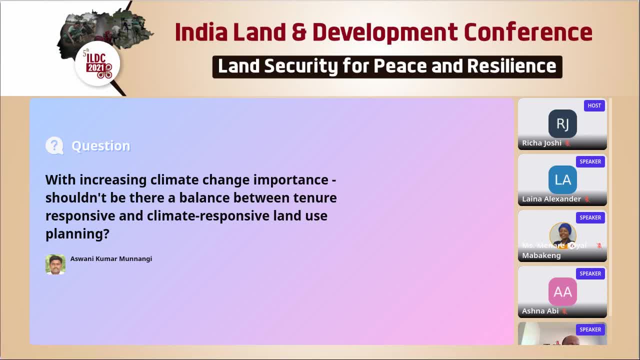 In my own experience. actually, the area where I've been able to supervise Tenant Responsive Land Use Planning application is in the Philippines, not in Manila, but rather within the space of the indigenous people And within the space of indigenous people. what I'm saying here is that I can't answer that question. 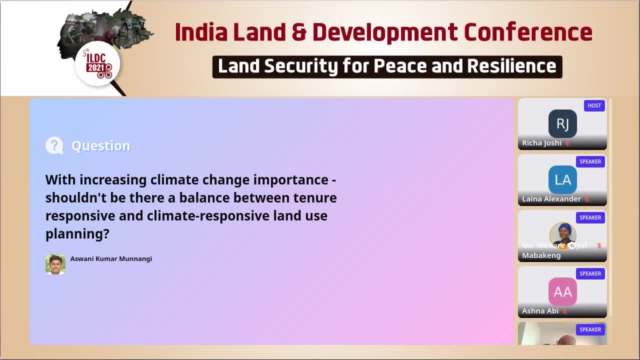 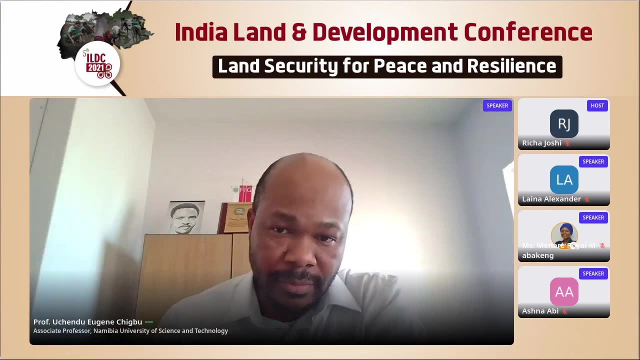 from the perspective of the key urban area, where I know that land value is seen purely from the financial side, But from the informal settlement, from the indigenous people's perspective, where I've been, it's about consultation, Like Royo said, 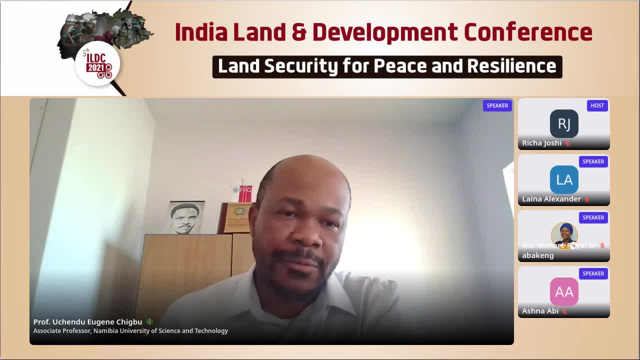 it's been about consultation You can't to start with with individual indigenous people. open space is important to them because it's part of their ancestral domain culture, So they have open spaces. They have they still in some cases. 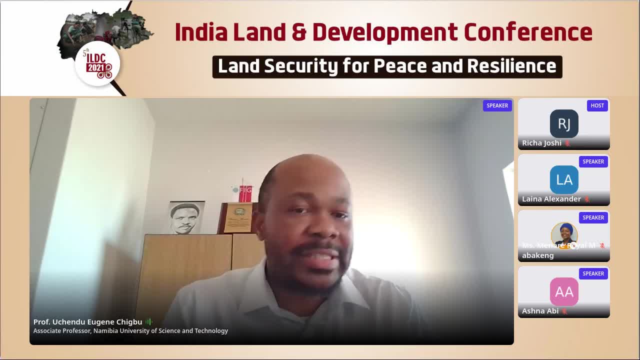 they still follow, And actually the conventional system is not allowing them to follow when it comes to farming, when it comes to other forms of land use, But what I realized there is when it comes to value. of course, value is much more geared towards, not entirely monetary. 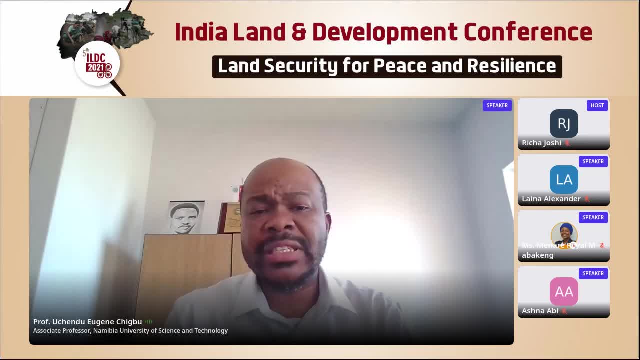 but more to ancestral heritage. But it has always been about, you know, consultation, trying to understand what the value means to these people and then trying to relate it to what it would mean to the state, and then trying to find, trying to find a balance. 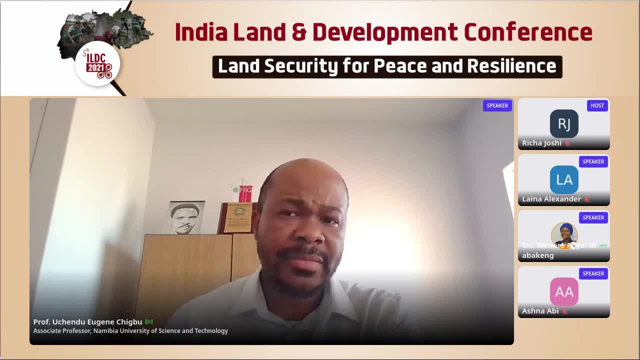 But at the level of the built up area I haven't had an experience, So I can only speak late on, you know, from that perspective And from that perspective, I would say that consultation will be part of it And, of course, 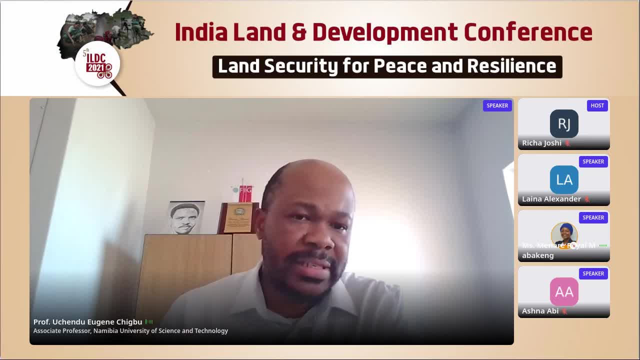 the normal valuation processes would follow. But one thing that I've also learned from working in Nigeria: even in situations where values have been professionally determined, when somebody's stubborn, you have to negotiate. You have to negotiate values because, and when it comes to informal, 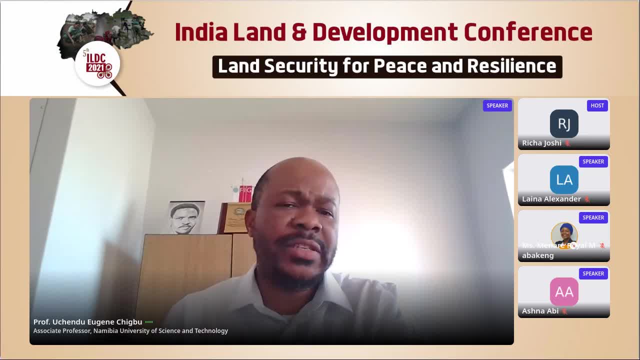 when it comes to open spaces. one open space means something different to another community, But where tenor responsive land use planning is key, I think, if I follow the principle now- and I may be speculating- is that the tenor responsive land use planning goes beyond the ownership. 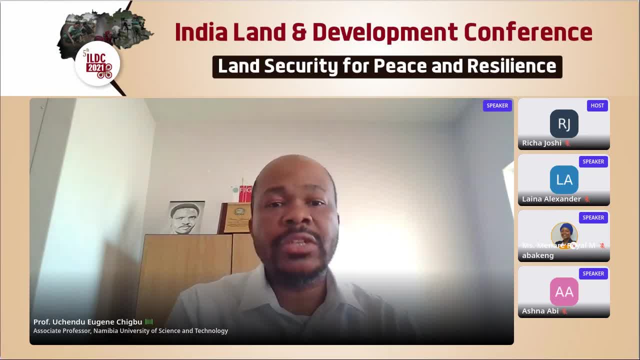 and right holding. But it also goes towards compensation for those who enjoy privileges, or have enjoyed the privileges that emanate or that subsist on a piece of land for a very long time. So, which means if there's an acquisition, if there's a change in use, 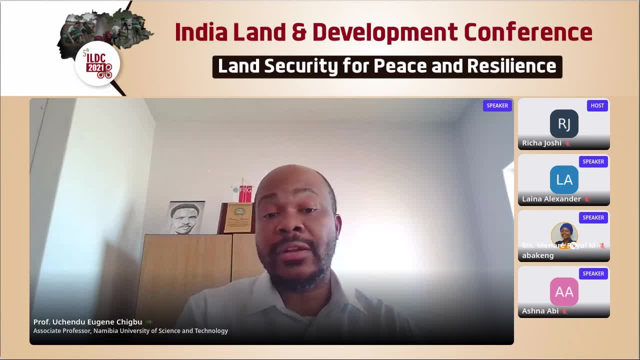 whatever effect that you would have on them, even when they are not part of the ownership in the legal sense, they deserve to be compensated for a loss of privilege or a loss of right, that is for sure, and a loss of ownership, And jurisdictions will always change. 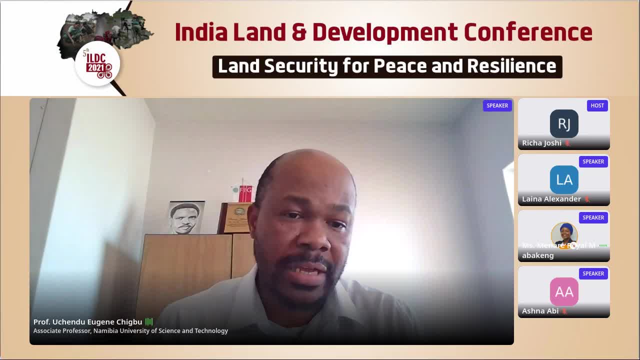 And rules will follow in terms of valuation And, of course, as determined also by human interaction, which is negotiation. Okay, Thank you, Chikwu. I'm going to give you another question, as I'm taking over moderating now. I see. 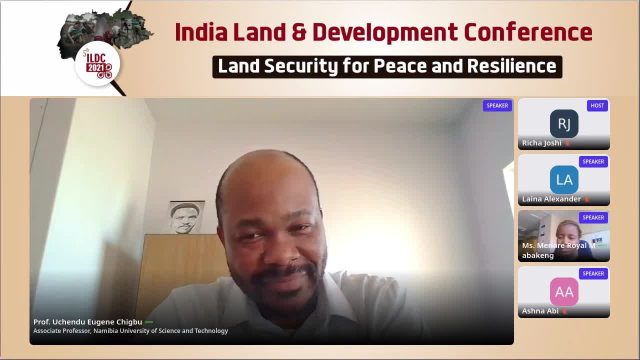 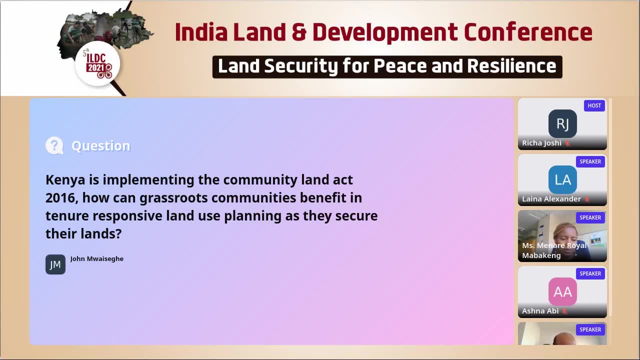 All right, There's a question here from John, quite an interesting one. John says Kenya is implementing the Community Land Act of 2016.. Yes, there it's on the screen. How can grassroots communities benefit in Kenya? responsive land use planning. 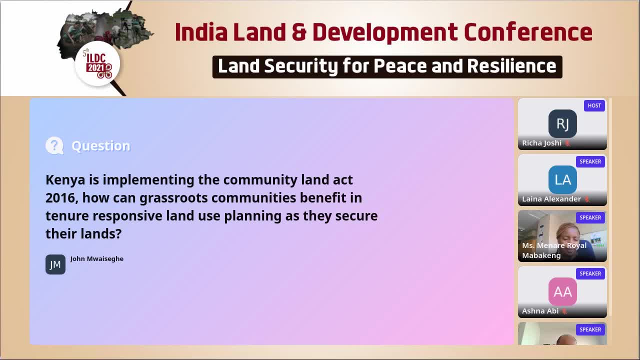 as they secure their rights, their land. Okay, Yeah, Thank you, John, I think. yeah, I'm glad to hear that the Community Land Act has been implemented. So actually, Kenya- I forgot to mention Kenya- is one of the pilot areas for the Tenant Responsive Land Use Planning. 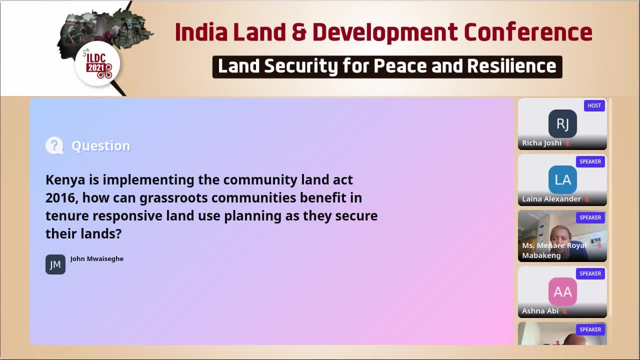 And John, if you've had, I know, I want to take you to a particular case where Tenant Responsive Land Use Planning has been used in Kenya, And it is. I don't know the region, but it is. the rice paddy farmers somewhere in Kenya have had to use Tenant Responsive Land Use Planning for community water use. 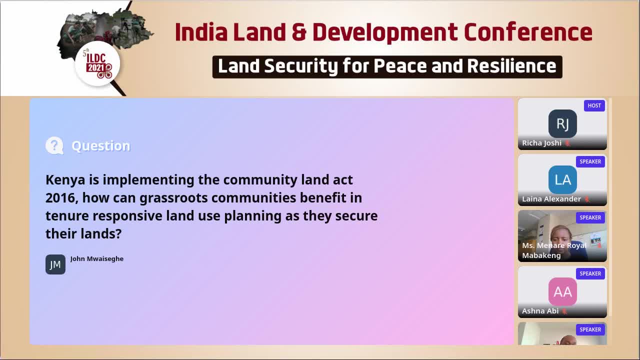 So your question is important because it takes time. It's important because it takes us just beyond the physical land And so, but some of these things are already in some of our previous publications, So I would like to refer you, I'd like to refer you to a publication we did on. 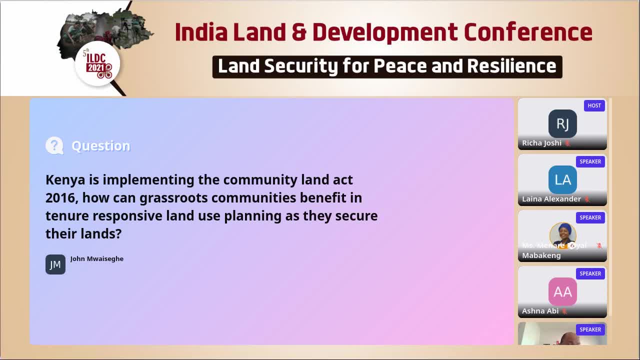 on on learning initiatives for Eastern and Southern Africa. It's presented at the World Bank Conference in 2000,, I believe, 2017.. So there, the Tenant Responsive Land Use Planning, for example, was applied in a Kenyan community. 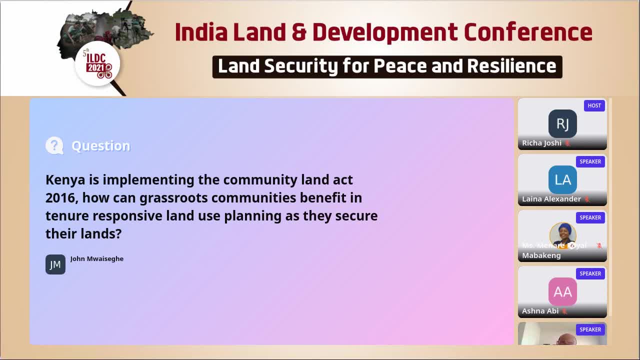 but a rice farming Kenyan community where you have water user association And they had to use the. in this case, the focus was on on on data, Focusing on data as the entry point for tenure. They had to use the. 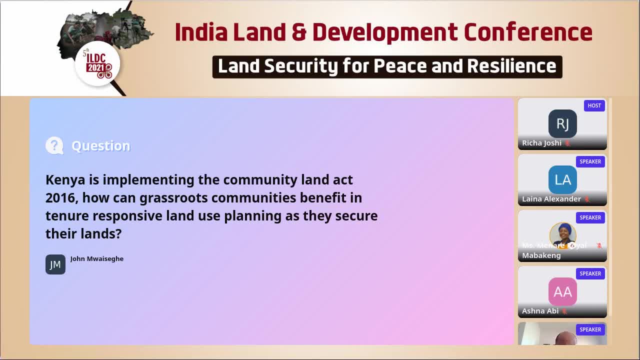 the social tenure domain model of the global land, to network, to record data in order to also determine how to rush water And to determine who stays and what obligation that has to be paid or responsibilities of the water users, as well as their interaction with the community. 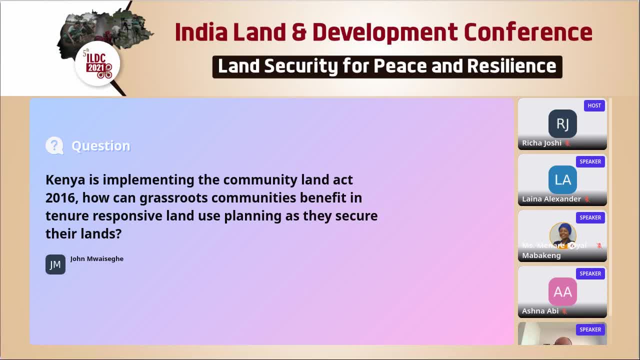 So, in this case, what actually happened is that the, the, the, the knowledge now, or, if you allow me to use the word, knowingness, or the consciousness of the water users association. well, farmers who are rice farmers, their consciousness of the 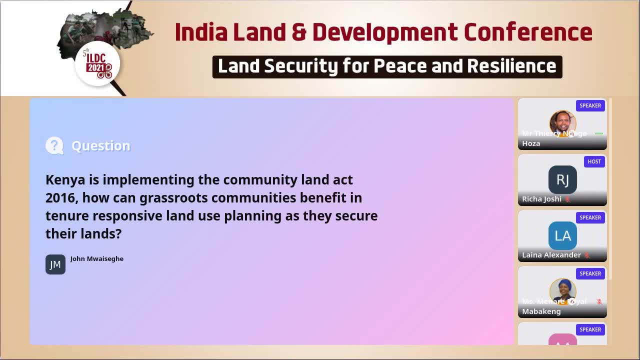 of the data that's that is available to them now happened to be a key entry point with which they could use to make tenure decisions as well as management decisions. Another place that I would that I could direct you to now- this is now an informal settlement- is in Uganda. 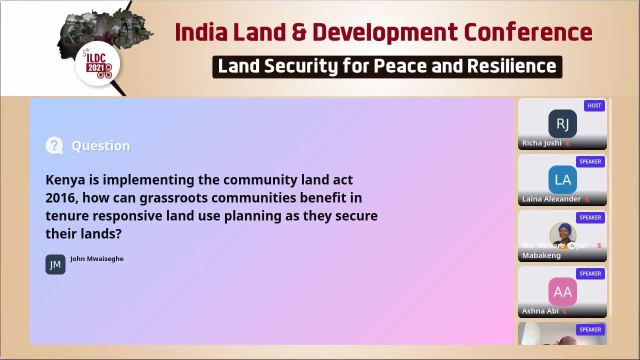 but in the northern part of Uganda, I think, I don't know, Mbara or so- Here the the community, and when I say local community I mean informal settlements, dwellers, and that's also part of the Sharks Dwellers Federation over there. 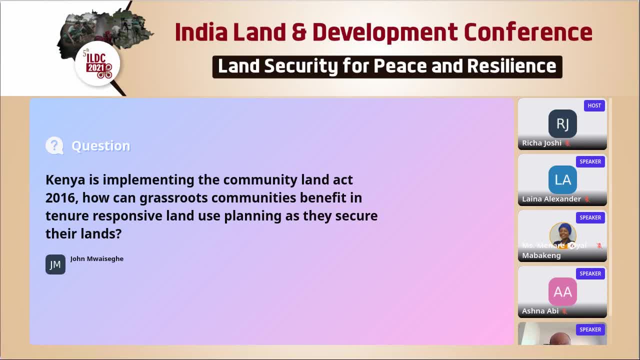 They actually use the social tenure demand model, following the principles of tenure responsive planning, to determine and capture all data that is necessary for them in their informal settlements. And because the local government, the municipal government, does not have data to work with, they don't know how many people live in informal settlements. 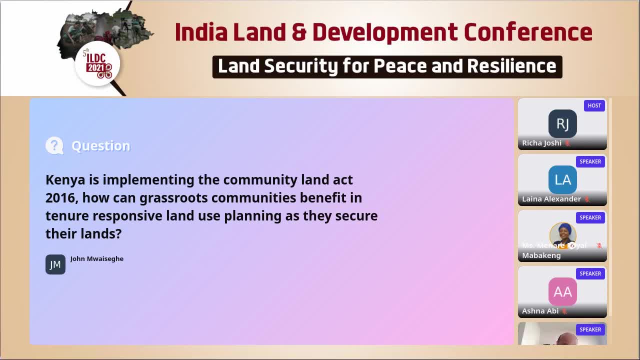 They don't know what sort of land is informal settlement. They don't know land uses. They just had no clue about how to make decisions in terms of urban planning. They now had to be consulting the this community that has this data and the community now is actually. 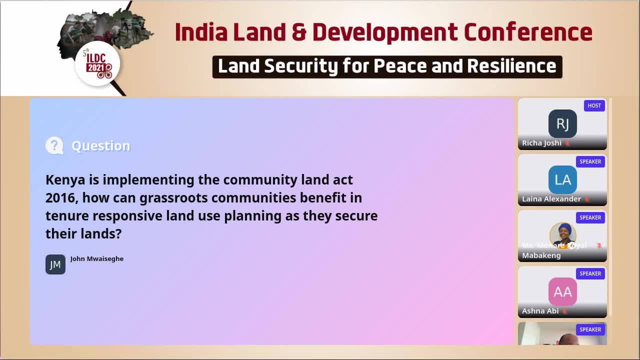 they gave them an office at the municipal office there so that they can tap into the data, because you need informal settlement data in order to manage informal settlements And governments don't have it. So what these people now did? they became a negotiation, a negotiation tool for them. 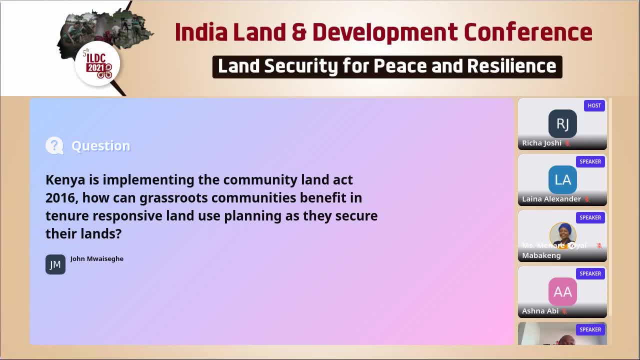 We give you data that you need and then we can also demand, make our own direct demands in terms of informal settlement, upgrading, And this has been working. you know that's the only way I can explain this, And I think that, when it comes to community, 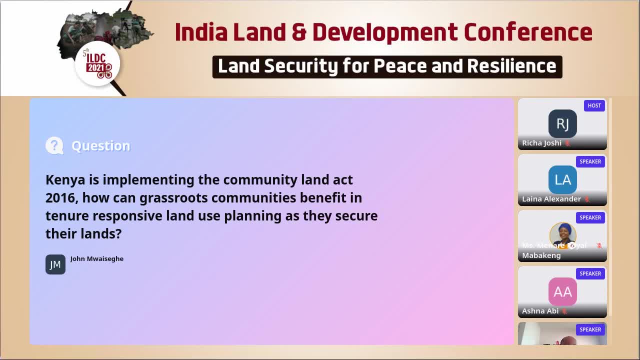 you know, implementing the Community Land Act in Kenya, the grassroots negotiations, the grassroots consultations and the ability for you to own the data that emanates from your own area would be a key point in this sense, And to do that, you have to plan. 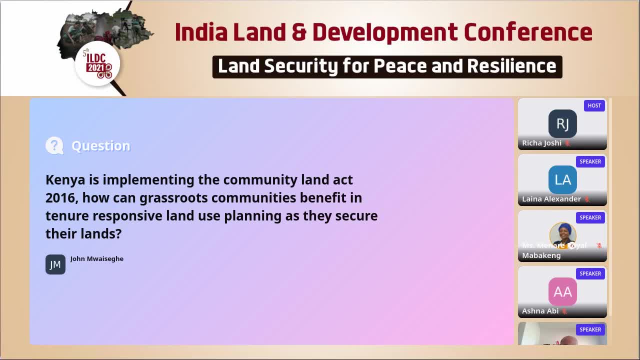 You have to do land use planning and you have to focus on making sure that every data that is available to you, that you capture it and is useful And, at any point when it's needed, you can use it as a point of negotiation. 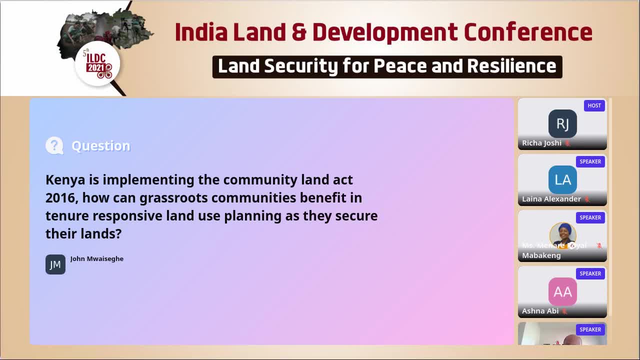 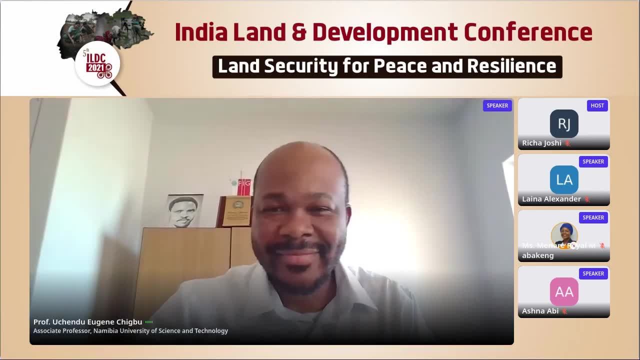 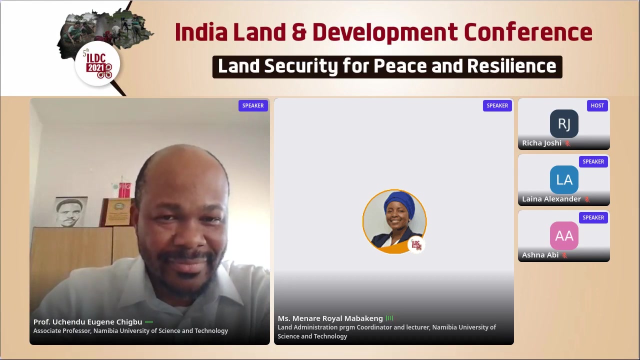 as you try to balance the power dynamics. I don't know if I made any sense, Roya, you're muted. Hello, Yes, sorry, Yes, I think I think you have dealt with the question, the answer, very well. 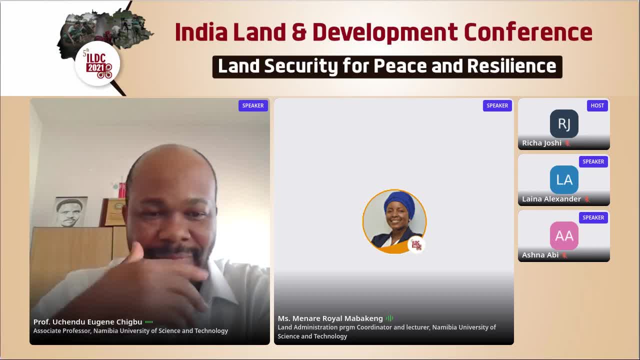 Like we always discuss within this field, when communities start being key implementers, or at least key partners within the implementation of any legislation, it means that tenure security would be the best possible outcome for them, Because if they are being provided, or at least being given an option of having less secure land rights, 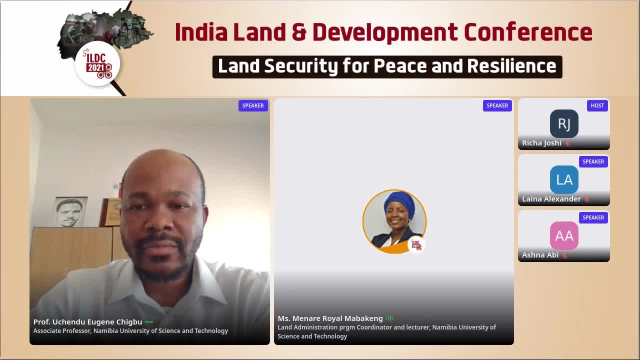 we have seen that there has been concerns that were raised. So what we within the Namibian case, at least from my area of research and experience, is that communities that are engaged in the discussions around how to plan or rearrange the informal area. 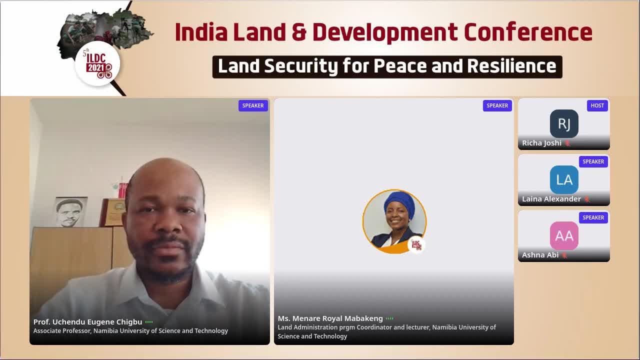 are always able to secure their land rights at the end of the project. In most instances, when we have areas where there's a high limit, there's a high level of tenure insecurity. Also, within the rural areas, it's a result of government projects that were implemented using a top-down approach. 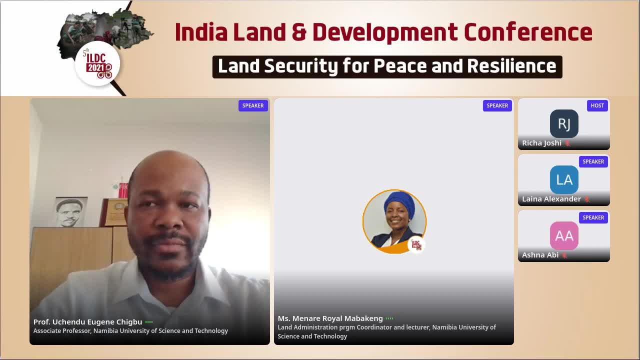 So we, I think, for the Kenya exam process that is going to come forth. They can benefit in using the tenure responsive land use planning by starting and initiating the project with the implementers, including the national government, and then having the communities have an active voice within the project itself. 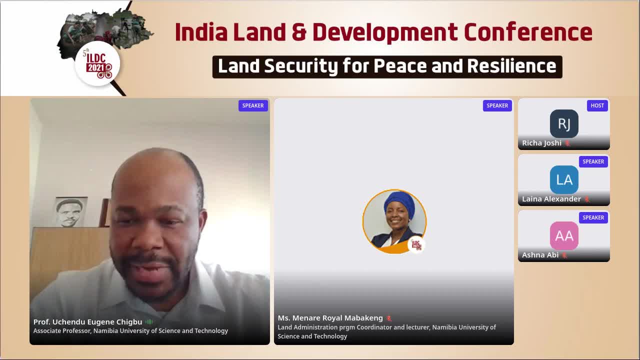 Yeah, that's all. Yeah, I have to add: we, you know, our time was up seven minutes ago and I think they extended our time by 10 minutes, So we only have three minutes to round up. So if there's no other question. 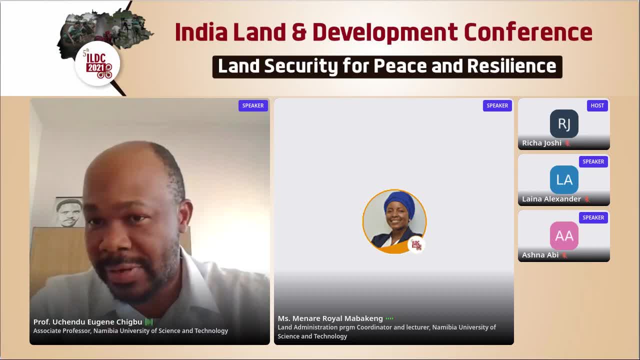 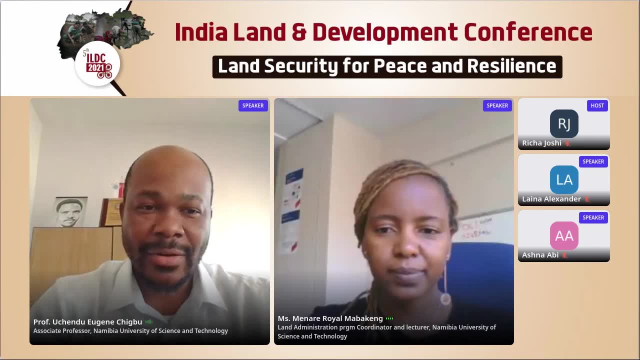 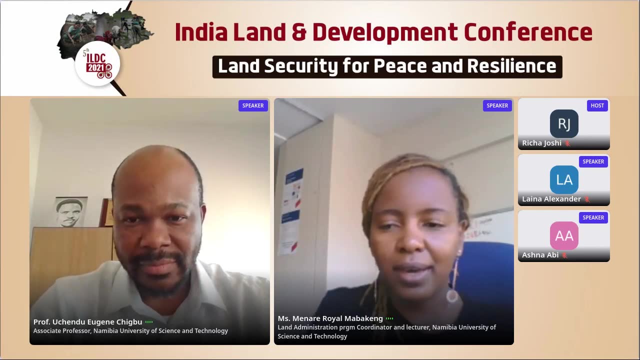 Roya, if you have a or if anybody Laina hasn't spoken, has any words, any final words, then we can close. So I give you the opportunity for a final word, then I'll close. Okay, I guess. thank you to everyone that has made time to attend this session. 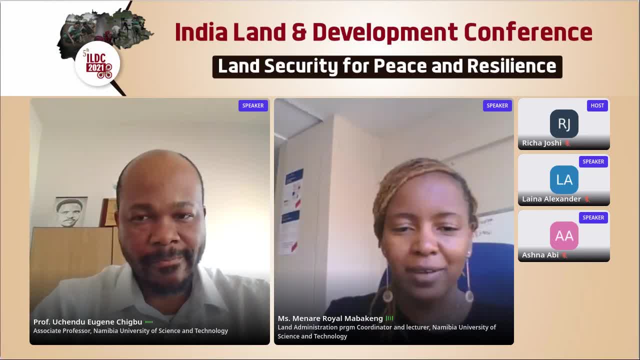 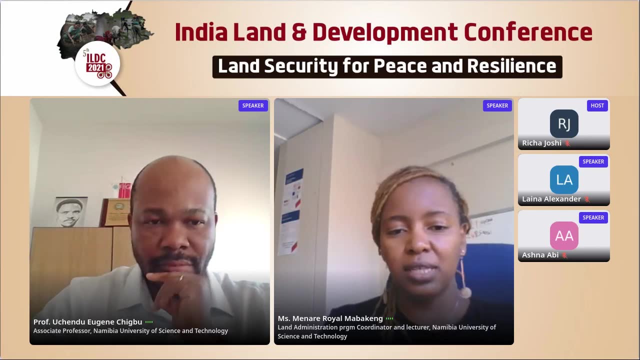 And if you have time, you can always make time to join our discussion. from the 8th to the 10th of December, We're going to have a conference centering on land governance and societal development, So if you're interested, we are available to share more details. 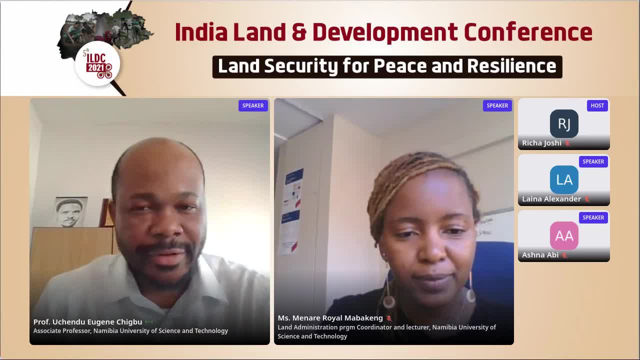 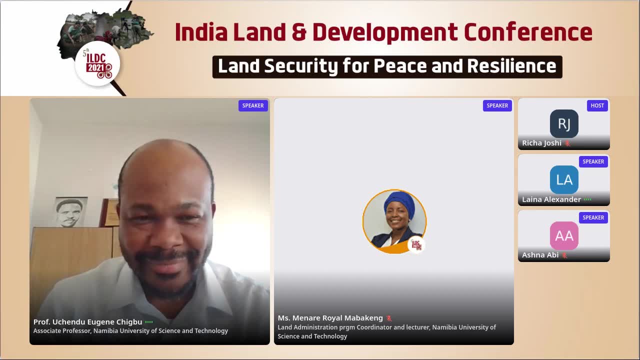 Thank you, Thank you, Thank you, Royo. Laina, do you have anything to say before I close? Nothing, bro, Okay. So first of all, I'd like to thank Royo. I'd like to thank Laina. 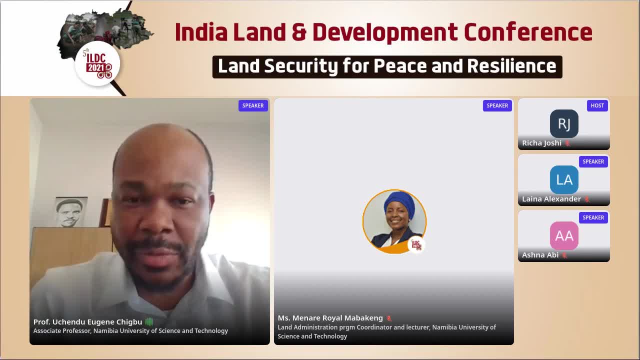 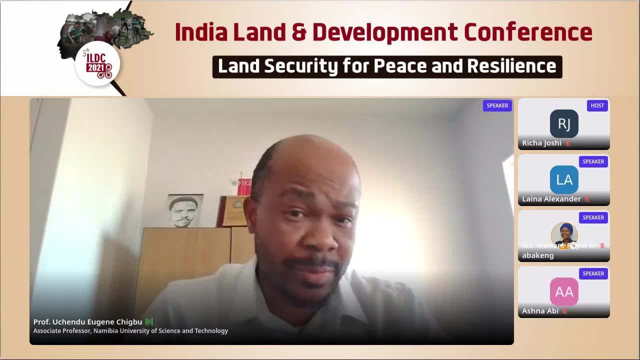 I would like to thank my other colleagues who didn't speak here but who made everything here possible. But I also, most importantly, would like to thank our Asian partners who made it possible for us to have an African day today. It's our first step in our networking to move beyond. 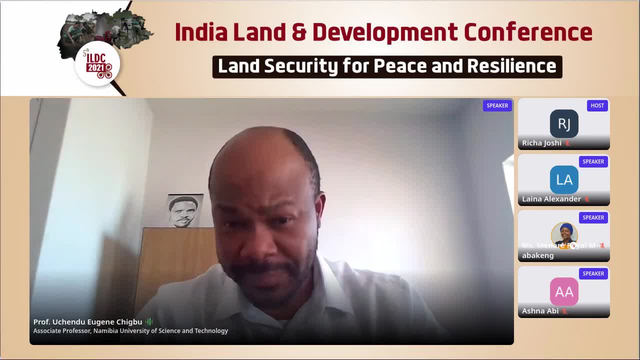 you know, goes direct to Asia And we have a memorandum of understanding to start working with our Asian partners And we hope that as we go on with our conference coming up between the 8th to 10th of December, that our Asian partners will be part of it. 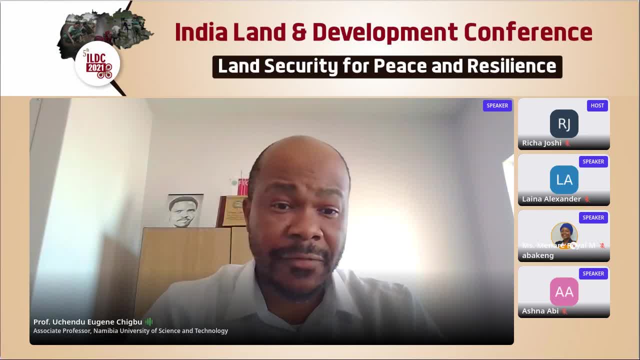 And we continue this partnership, you know, in terms of collaboration in terms of writing papers, collaboration in terms of proposals, collaboration in terms of projects, collaboration in terms of having one voice in, you know, projecting the global discourse on land. 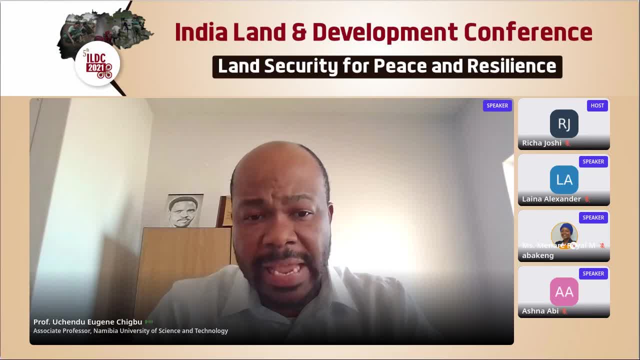 Now, please. you're very much welcome to join us between the 8th to 10th of December at a conference which is termed Land Governance and Societal Change. The conference is a collaboration between the Namibian University of Science and Technology. 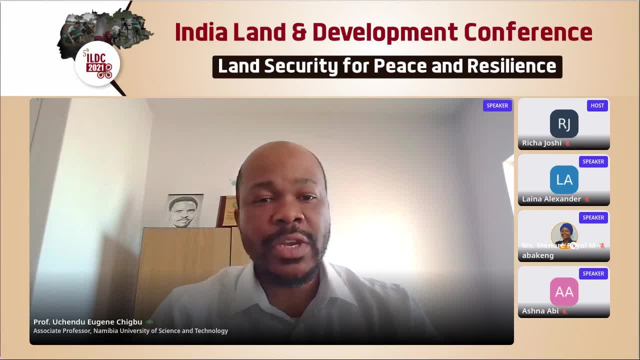 and the Hans Seider Foundation in Shandong, China, And we hope to have all of you there And in that conference. the book that my colleague Lina talked about, which I don't think is my book, is an edited volume. 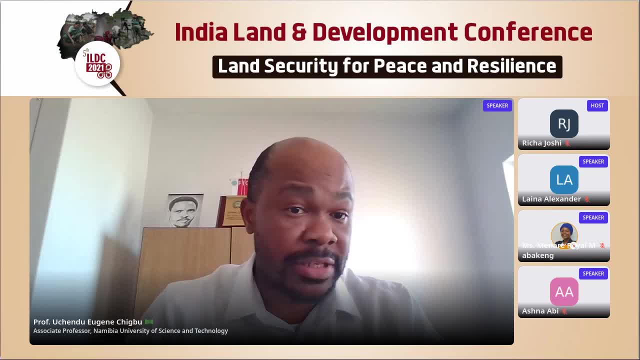 will be launched. This book will be freely available because it's been funded by the Hans Seider Foundation for Open Access, So you're going to have open access to it. But what makes this book interesting now, which is why you have to be there?